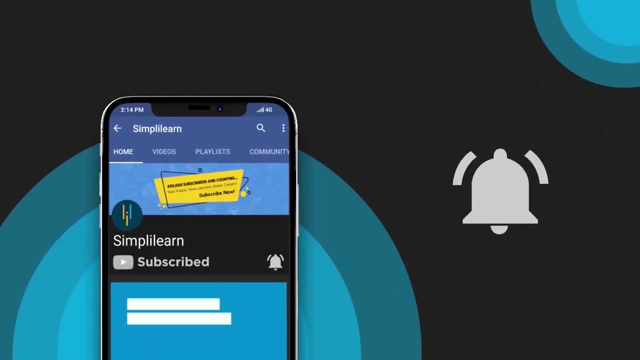 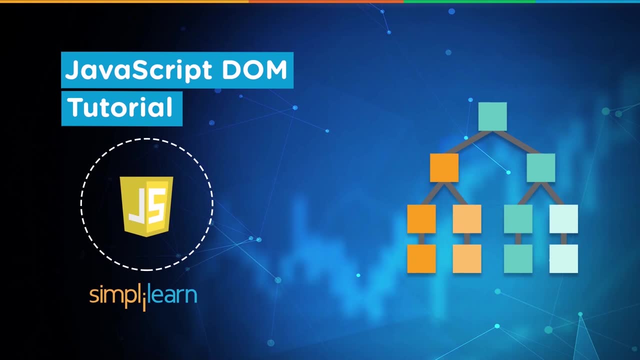 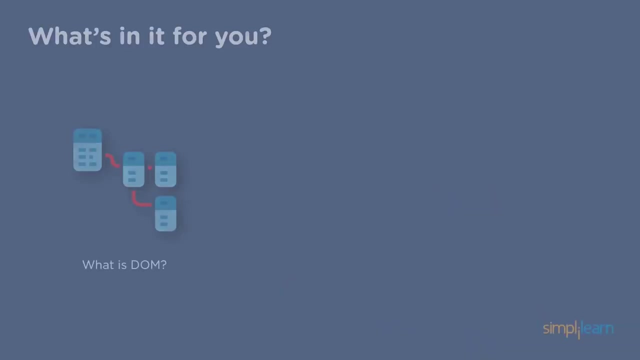 Hello and welcome to this video tutorial on JavaScript DOM. My name is Ezhi Lapparajat, I'm a corporate trainer and I'm with Simply Learn team Simplylearncom, the world's number one online bootcamp. Without further delay, let's get started, And in this session, we. 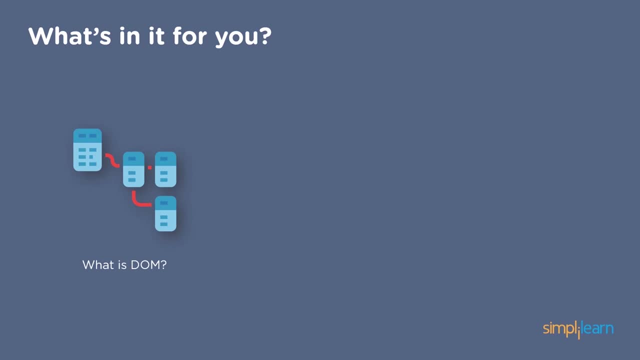 will be seeing what exactly is DOM, which is Document Object Model, And how can we manipulate the DOM, How do we interact with the DOM elements and nodes. And then we will wrap up the session with a very interesting and engaging demo, which is about movies. So we'll be creating 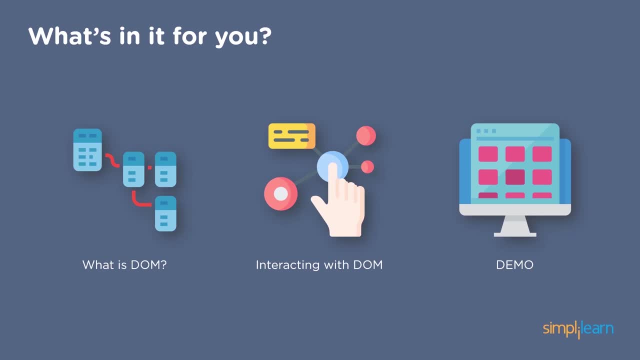 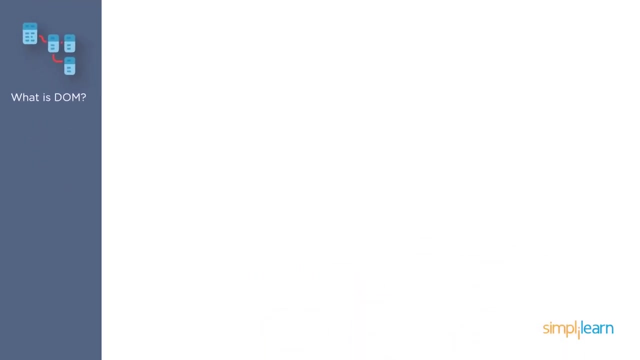 a movie web page where you can see the list of movies, You can search for these movies and we also can add a new movie and delete a movie. So these DOM manipulations will be seen for a movie web page. So what is DOM? Document Object Model? It is the data representation. 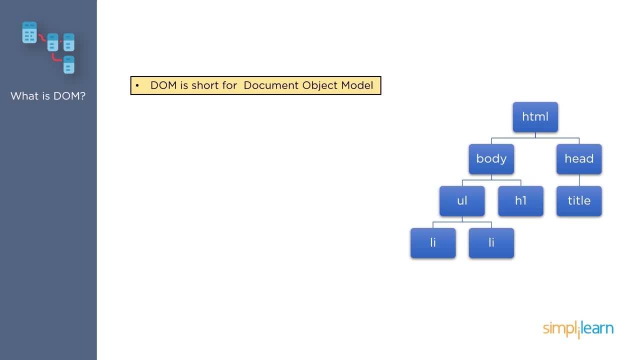 of the objects that comprise the structure and content of a document on the web. So this is the page so that the programs can change the document structure, style and content. DOM represents the document as nodes and objects. This way, programming languages can connect. 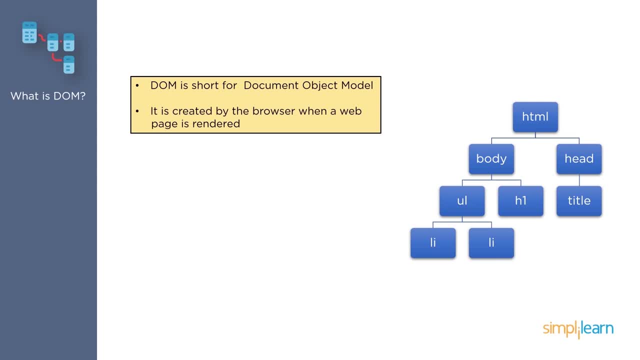 to the page. A web page is a document. The document can either be displayed in the browser window or as an HTML source, But it is the same document in both the cases. The document- object, model or DOM- represents the same document, so it can be manipulated. DOM is an object-oriented. 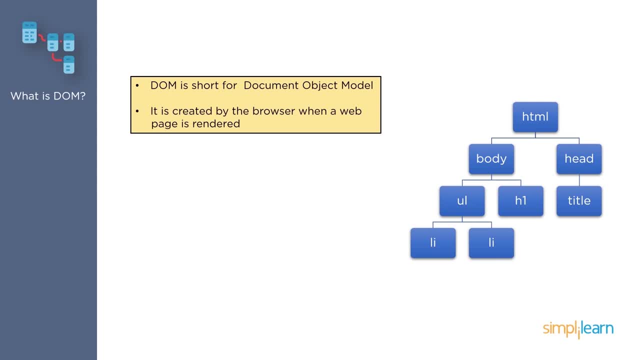 representation of the web page, which can be modified by the scripting language, a very powerful language like JavaScript. DOM is usually represented in a hierarchical tree-like structure, So you can see this picture on to my right, where you can see a HTML element. 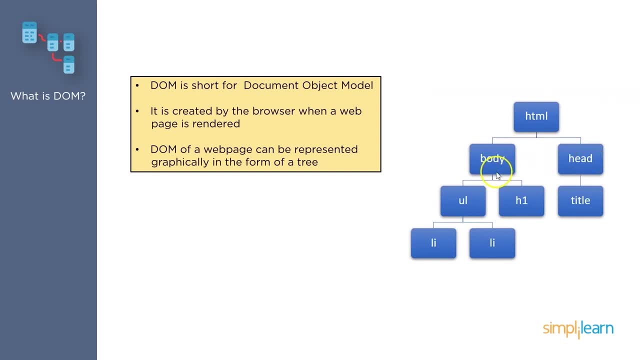 which will be the root, And this is the HTML element And this is the HTML element which will be the root, And this is the HTML element And this is the HTML element which will be the parent element. And it has two child elements that you can see. One is the head. 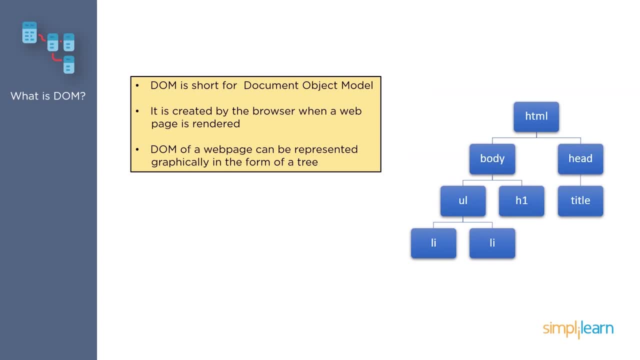 And then we have the body. Head consists of the metadata, like title, It also consists of script and style tags, And body comprises mostly of the content of the web page. So in this example you can see a H1,, which is a heading tag. You also have another element. 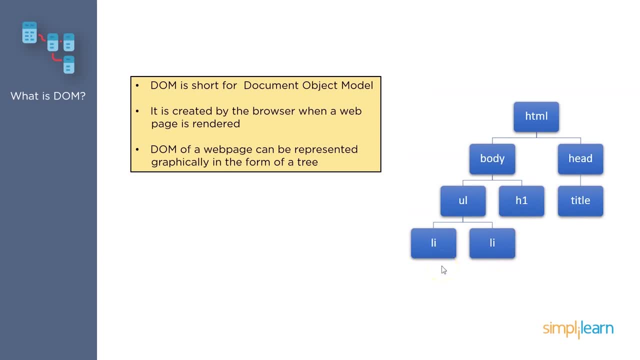 which is the list element that you can see, which is an unordered list element, And this is an unordered list which consists of two list items. Now, these two list items are the child elements of this particular unordered list And these two comprises of the child. 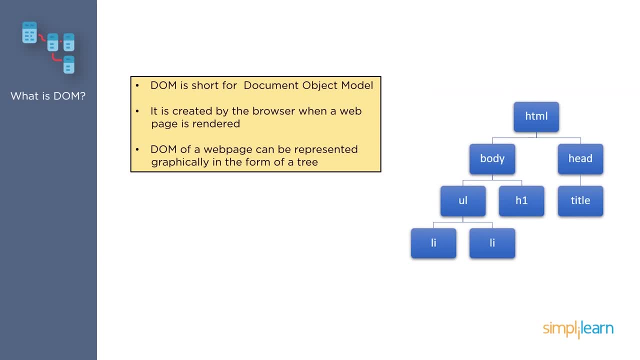 element of body which in turn is the child of the root HTML parent element. So we have a parent and child relationship that you can see over here And when we speak about events later in the module. so you can see like how the parent 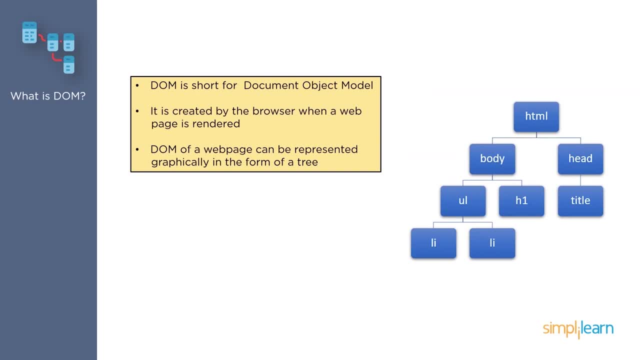 element can handle the child event or the child can be able to manipulate the events of the parent element via JavaScript. So we can use JavaScript to perform different task of DOM manipulation, like traversing the DOM. You can read the text, or HTML text or inner. 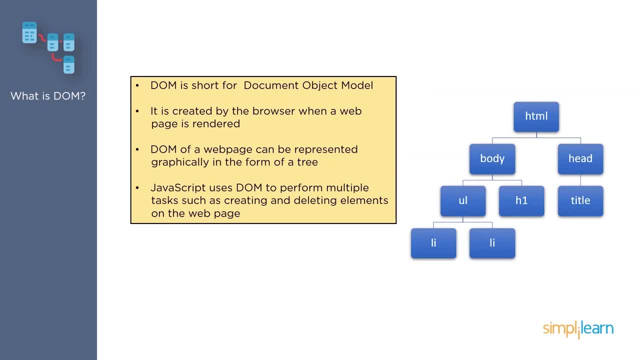 text or whatever property value which is present in the form of the element, inside the element. more So you can do a read operation, basically, or you also can edit or update something and you also can add new element. We can delete the existing ones, We can change the style, So we. 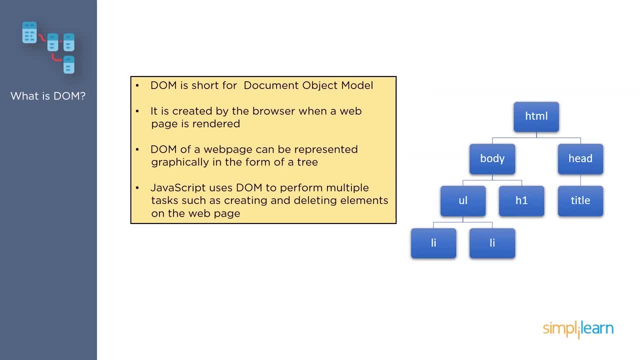 can do all these manipulation of this document object model using just javascript. So all of the properties and methods and whatever events that we have available for manipulating and creating pages, and these are organized into something like objects, So the document object that represents the document itself, the table object that implements 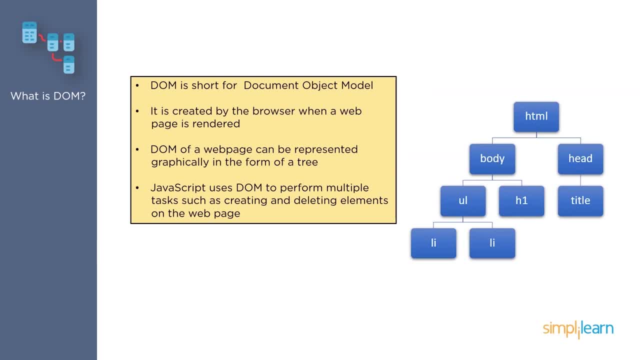 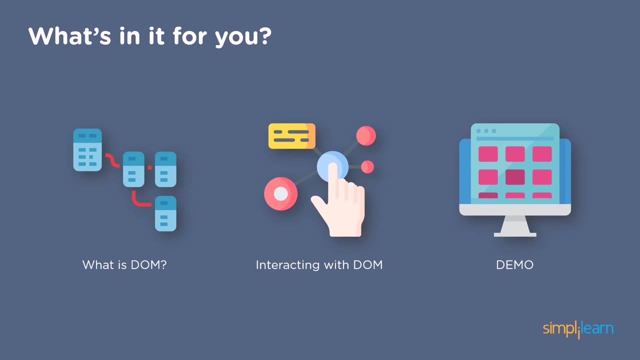 the special HTML table element, DOM interface for accessing HTML tables and so forth. So the entire DOM. if you see, it's like object reference, object by object reference. So what is the power of JavaScript in manipulating this DOM? So we'll see the perspective of JavaScript now. 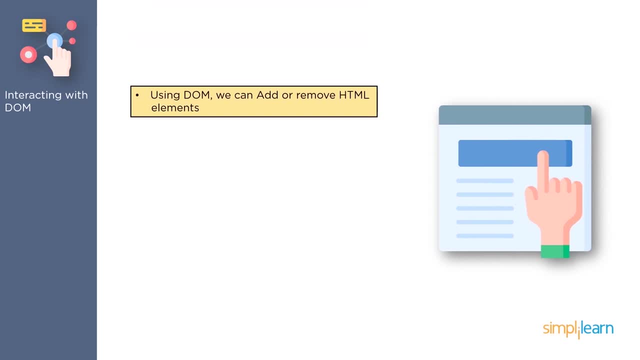 So using JavaScript, as I told earlier, so you can add elements or nodes or you also can remove the HTML elements or nodes that we see in the structure, But this is just not HTML elements of the content. Even you can manipulate the style, So you know cascading style sheet or the CSS. 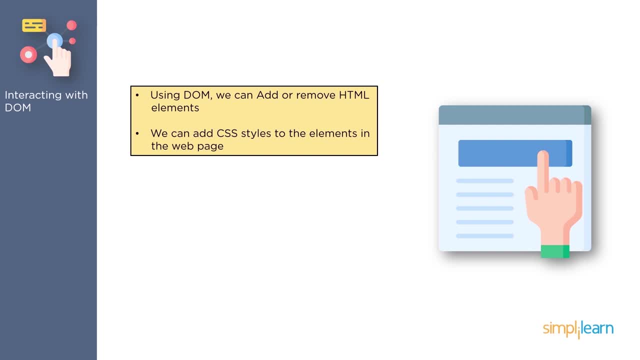 which represents the theme of a page. So for a web page, the theme, or style, is very, very important. So the HTML represents the content and the CSS represents the style, And the JavaScript is the core functionality or the feature of a web page. So these three things. 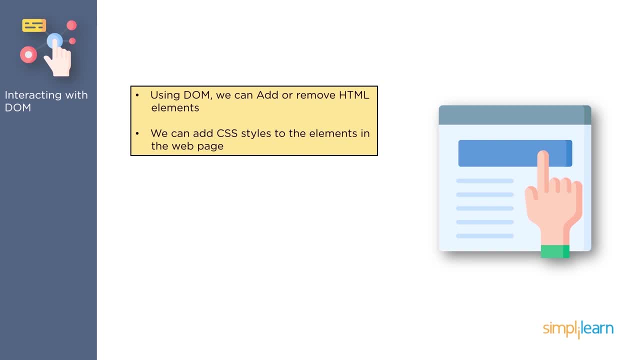 are, like you know, like a trinity of a web page or website. These three things complement each other and go hand in hand. So just with your JavaScript. so your content is definitely important. Content is king for any particular website or system, So content is mandatory. 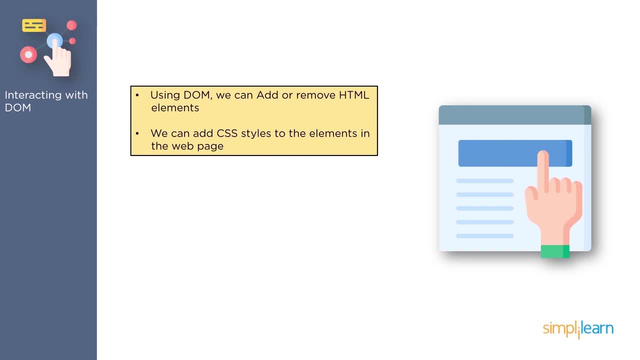 It has to be there. So without, Without content, it's nothing. But style is also very important. So if you have to attract your first-time customers, so you can attract them only with a very nicely styled theme or design. So this UI and UX design plays a very important role to attract your customers. 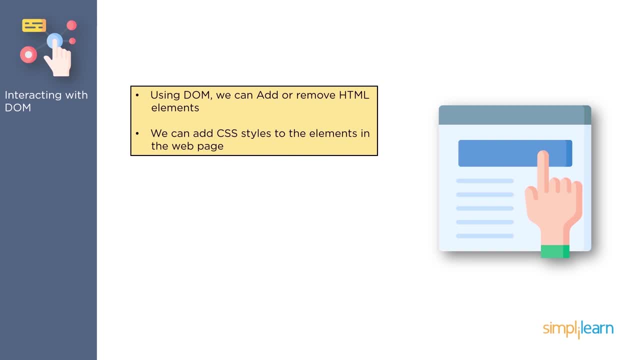 So, after attracting your customers, so these are just not enough. It is also important to provide good features. So your customer is now trying to shop from your website. So he is so attracted by your design- minimalistic, beautiful design- So he starts shopping. 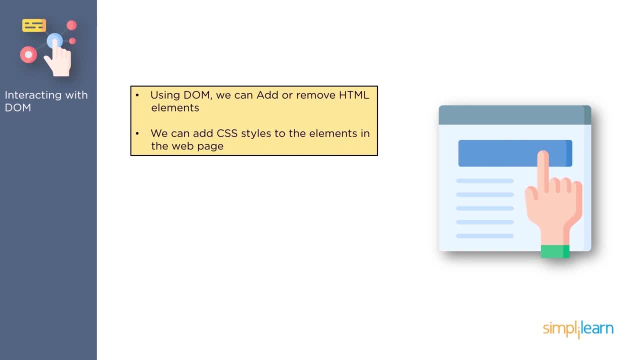 And after that, at some point or the other, he's unable to put items in the cart or he's not able to contact you via some contact form. So these are provided for your JavaScript or some JavaScript packages like jQuery or Angular or React. So this is very, very important. 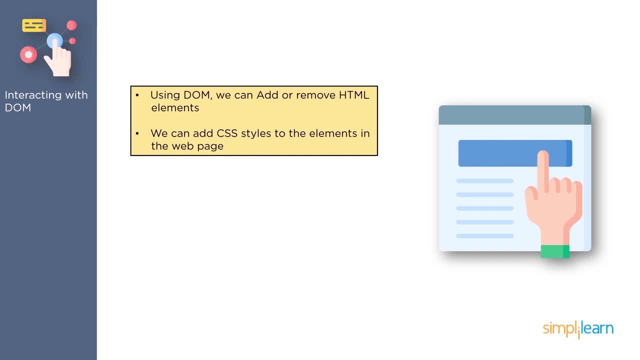 So the functionality and features. if you don't provide it, of course the customeryou're going to lose your customers custom. so your javascript is so important and powerful here that so i was saying that using your javascript you can add a whole lot of html content. you can from scratch, you can add styles. 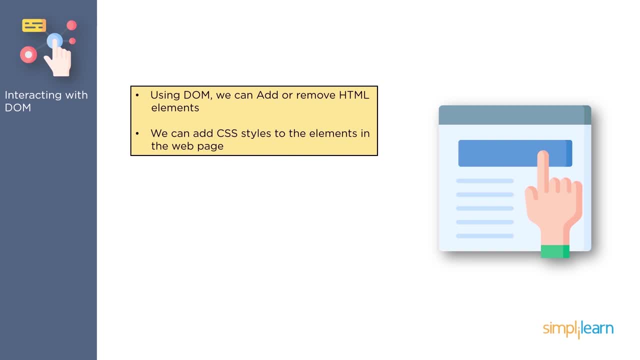 also, or change the existing style, not just the font and color. you also can completely change the spacing, padding, alignment, everything. so the entire theme, style and content you can change via javascript alone. and coming back to your events now, this is very important part of javascript. this is the place where the user interacts with that web page or website, say, 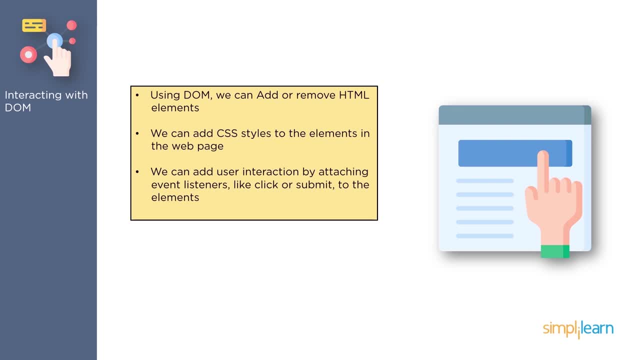 for example, in the form of a form, so you have a registration form or a contact form. so using these forms, so where we have these input elements like a button, we also have a lot of text boxes and check boxes. so all using all these input elements so we can get the input and we can 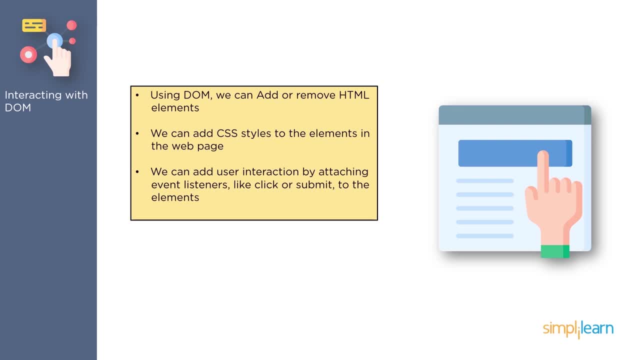 interact with the user. so the user can click a button and he can select something he can blur or he can get into some particular input element, but by giving him something focus. now, all these are done in the help of some triggering points, which is called as events. 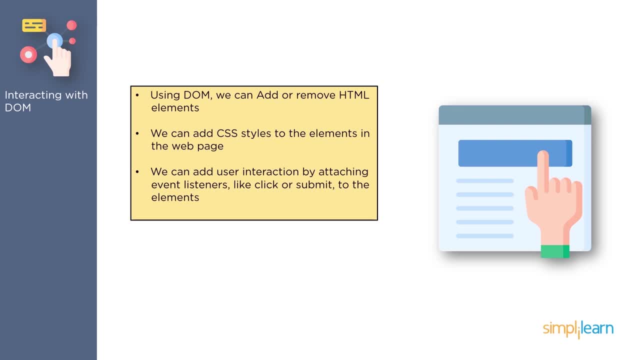 now we have these event listener, especially for older browsers, and these events are nothing but some triggering point which can trigger some actions. now these actions are termed as functions or your handler for that particular event. so to put this in a very simple layman form, say for example: 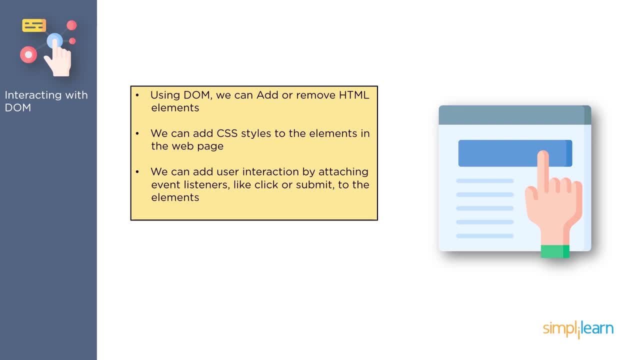 simply, you are attending your door's. your door is the floor and, of course, if you wereénding the door and checking who's itand you are getting up and uh, you're attending the door, you're attending the door, so you're opening the door and 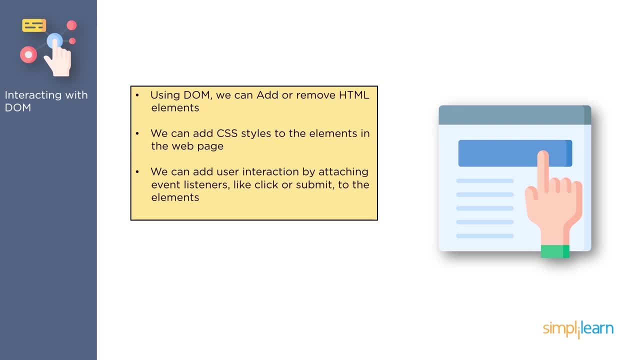 checking who's it. so in this scenario, so someone ringing the bell is the event and you getting up and going and seeing so who is it and accordingly responding. so that would be the function, so that is the action. so you, that particular event doorbell has like that one in the confirmation. and the steering and the structure. so all that you have to do to enable this event is simply not working and that is where the thing starts. so just make sure that this prevent that, if the event is in order, we can try to do that so well, because if we do, you can do that the other way around. 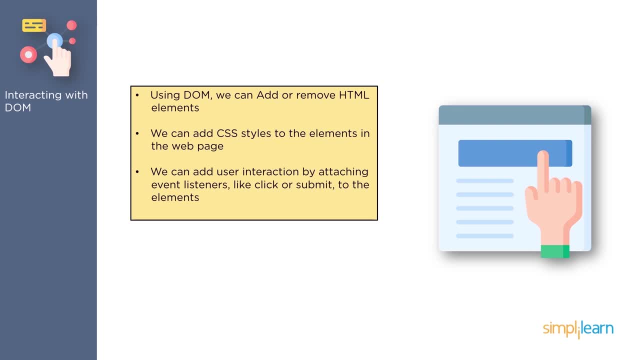 you can perform the following way: like with this and the other way around, doorbell ringing has triggered you to do or take some action, which is your function. so we will see more about this event. so in this project we'll have a lot of events and we will also be handling. 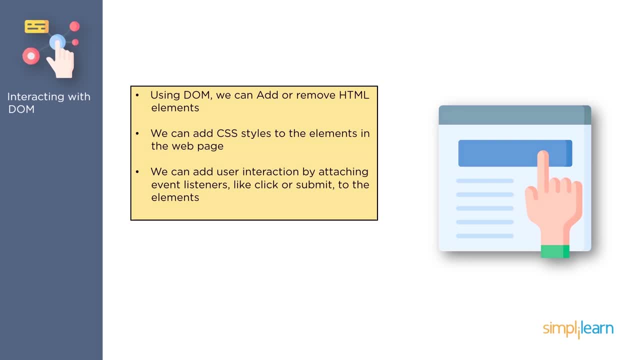 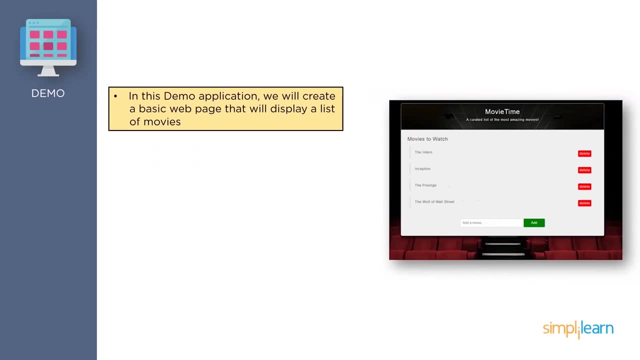 those using some functions and actions. so what next here in our project? so in this demo that we will be seeing, what are we going to do? so what is the takeaway? so what can you expect out of this? so you can see this screenshot. so this is the web page that you will be creating. 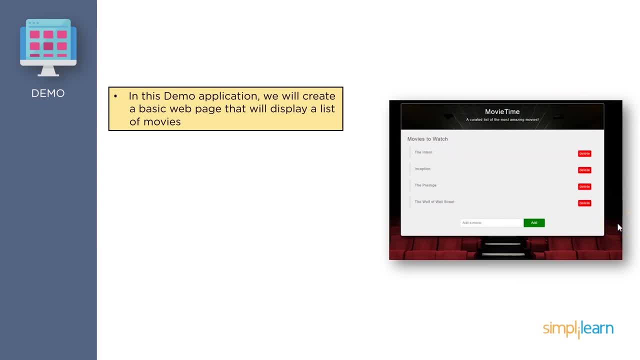 now this web page. as i told you earlier, it is a movie website, so it's like a movie web page. it's a single page that we are going to create and you can see a list of movies, to watch some latest movie. so you also have some red color buttons to your right. so these buttons, like so here it is written. 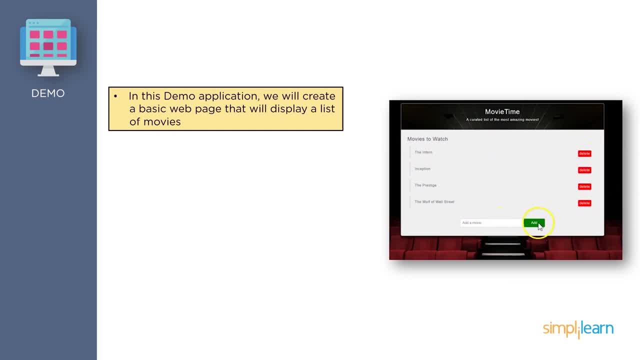 as delete button, and there is also a green color add button over there, which is at the end of the page, where you can input some movie name and you can dynamically add it. now, all these we are doing by our javascript, so you can statically add it also using your html, but in this particular 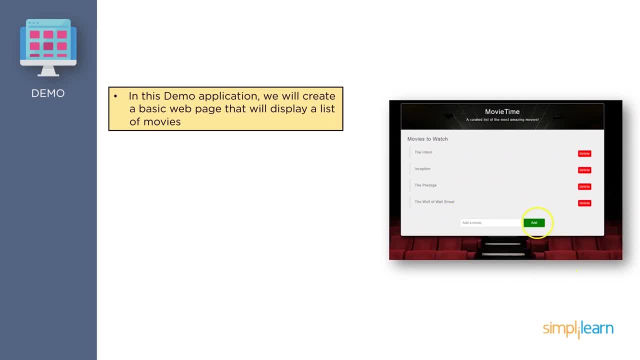 video we are going to show you how to add a movie name to your javascript. so in this particular example, so we are going to use javascript to dynamically add a new movie and if you want to delete those movie, we are going to delete that also. so this is what we are going to see as an 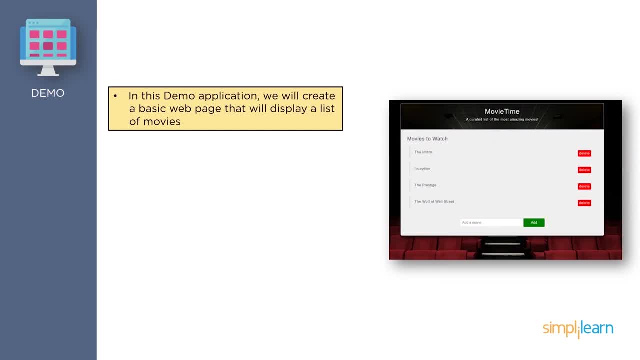 example, and in this demo application, so where you can create these uh details of the movies. now i have to say something here. so i have styled this using css, but we will not be going in depth into the css because that is not in our scope, but i will walk you through the code that i have written. 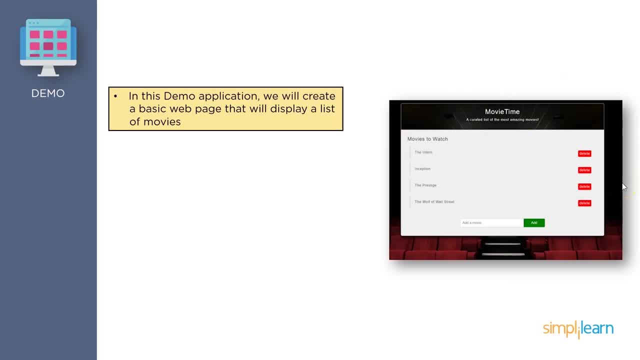 so that you get this beautiful. you know the background image and the alignment and margin and padding. those are the properties that i have included to get this style, so i will walk you through that then, once that is done, so we'll focus more on our javascript code so that we can create this particular um movie website in an easier so. 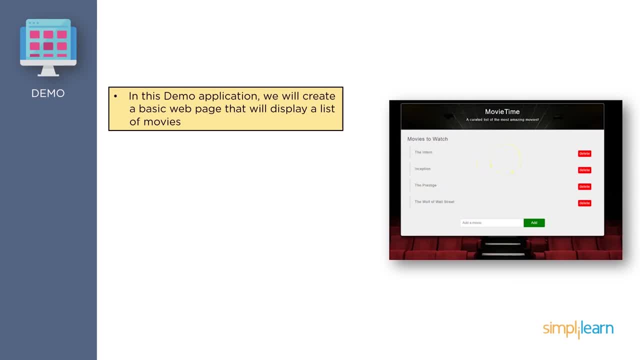 very, very simpler, easier manner, so how we can implement this particular concept of them door manipulation so that we will be seeing in our movie project. okay, so let's get started, and before we begin with the actual coding of creating a new movie and deleting a movie, so before we do that, i would like to walk you through the um actual application. 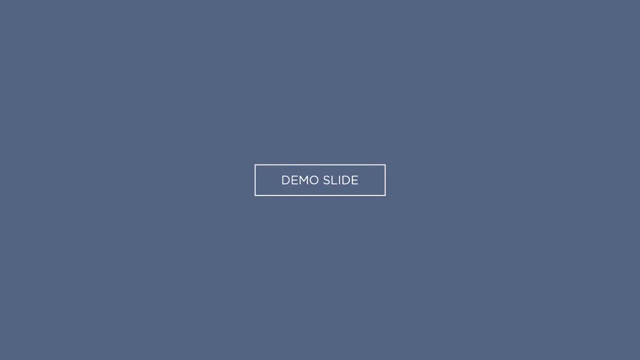 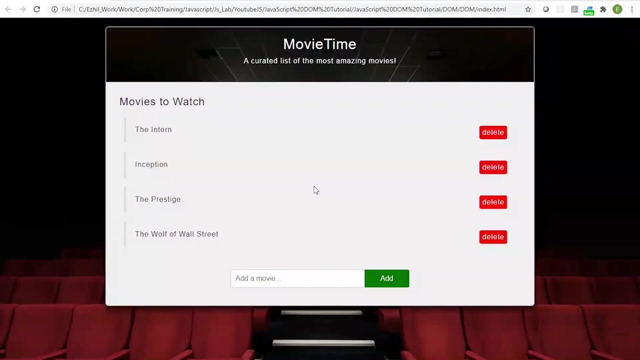 so let's get started on that. so before we get on to the coding and stuff. so I would like you to take a look at the final web page, or the website that you would be creating. so let's take a look at that now. so this will be the website that you will be. 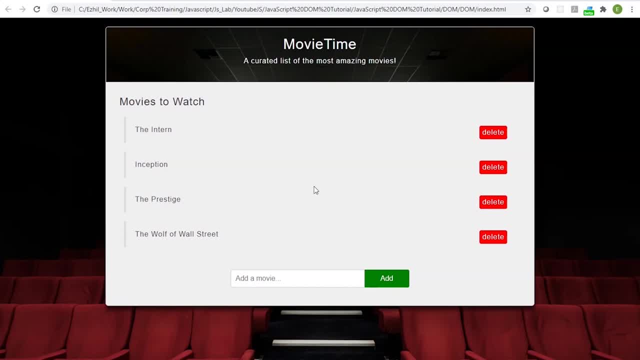 developing so you can see that it's a movie web page. it's it's kind of a single page application, because we are creating just one single web page for this particular demo, so you can create any number of pages you want later, but for this we are just going to create one index dot HTML now in this, if you 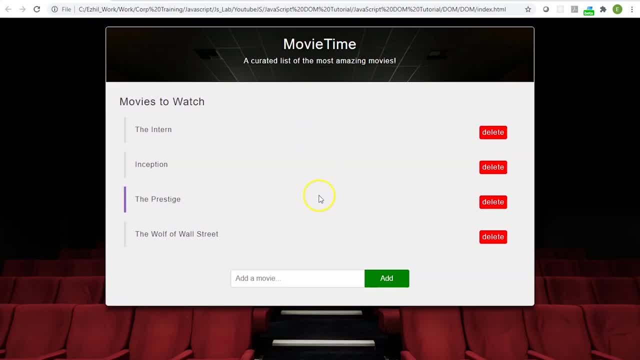 can see. there is a list of movies here, popular movies, yeah, so most of my favorites that you can see. and as I move my cursor, you can see this window and it will apply to any of the movie…. there is a purple color like a border. that's actually a border that I have. 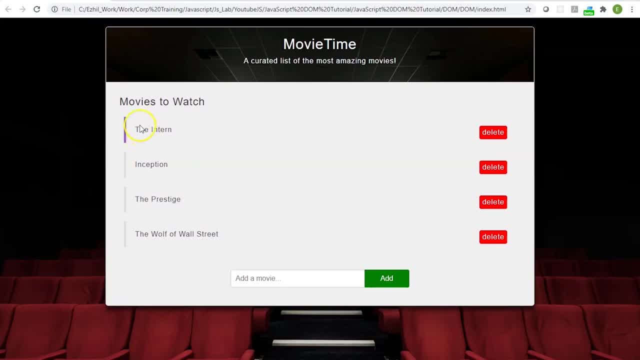 written in CSS. it's a border property. so you can see that on the left, which is highlighting that particular row, and you also can see a corresponding button in red, which is the delete button. so when I press it's going to delete that particular movie, and you also can see a text box at the end of this page and 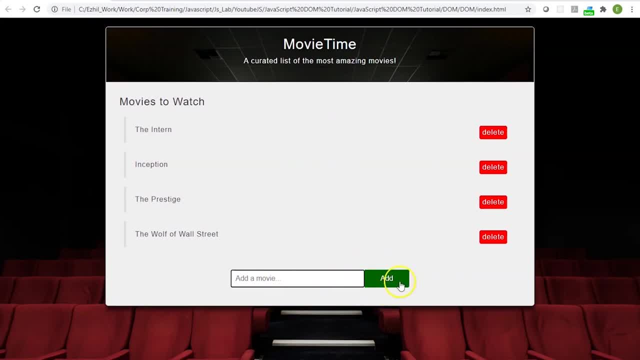 there is a green color button to add a new movie for this. so you can see, the entire page has been styled in CSS so it looks quite appealing. so I have given an image which emulates like a movie screen, movie theater screen, and there is a card. 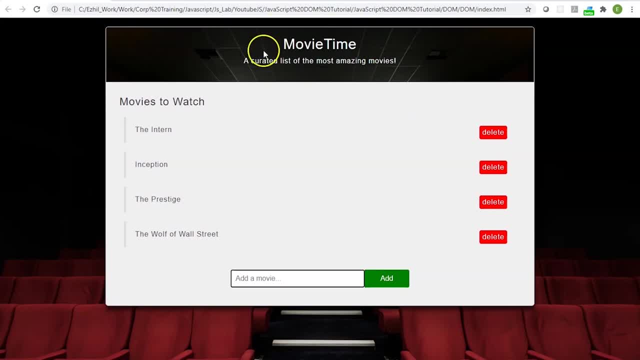 that you can see. so this is the card and so, which has this title and a tagline and all the other things that you can see here. so you can see that I have given an image and I have given a title and a tagline and all the other things that. 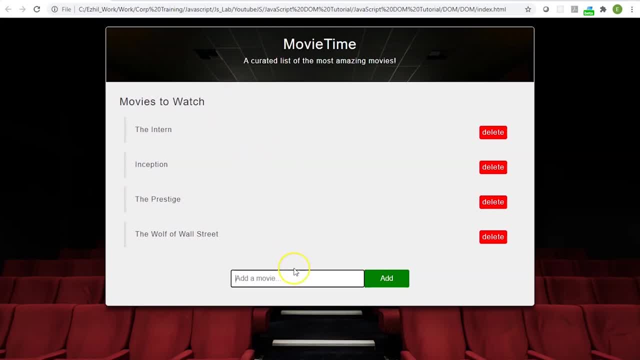 these have been aesthetically arranged here, as you can see. so there's a lot of CSS here. so which goes about to create the theme and style of any web page? so CSS is very, very important. so if you have to attract any- you know- probable customer for your page or for your business, the something 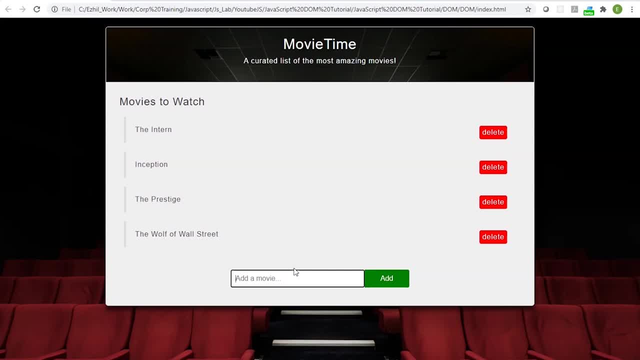 that is very important. the entity that is very important is your style or your theme. so the CSS plays a major role over here, so I will show you the. you know I will have a code walkthrough of how I have styled using CSS. so let's try to add a movie over here. you also can see there is a. 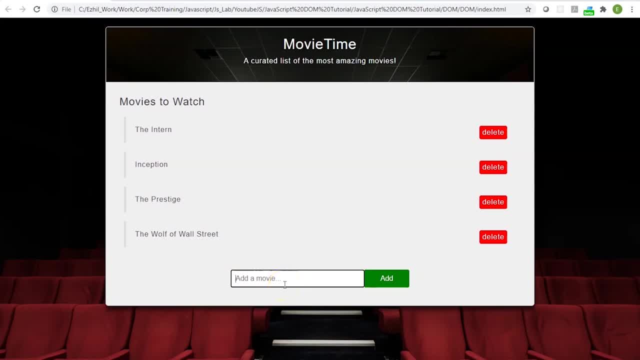 placeholder tip. also text also over there: mmm, let's go on with this movie, yeah, the popular one. so let's say add and you can see instant connection now Avengers getting added at the end of this particular room, and you also can see that there is a delete button that got added automatically. so if I have to delete a movie, so you can see. 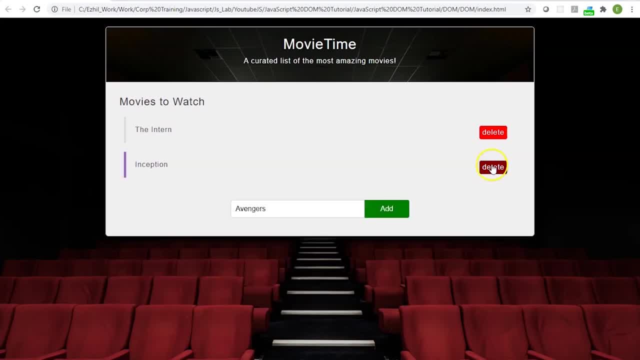 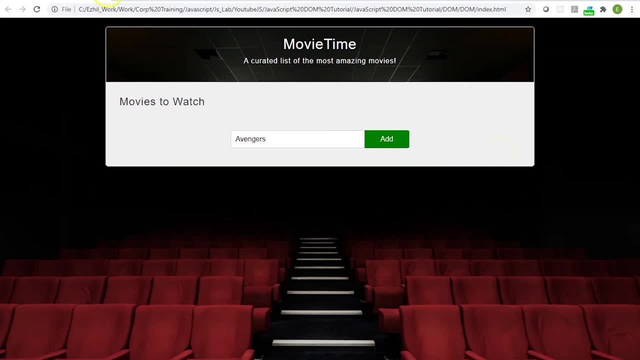 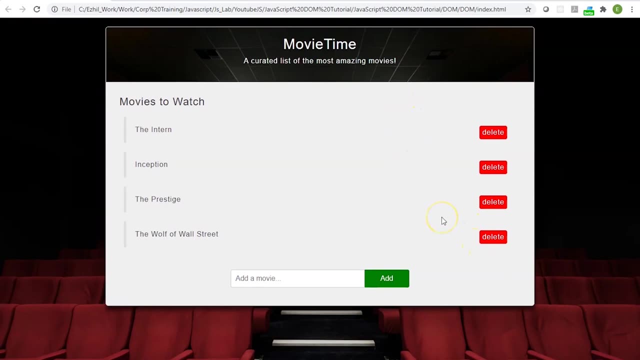 that it just goes off instantly. and I have to remind you so this is not linked to any database, so it's not persistently stored. so if I have to refresh it, you get everything back. so this is just like stored in an array. so it's just a list of movies. 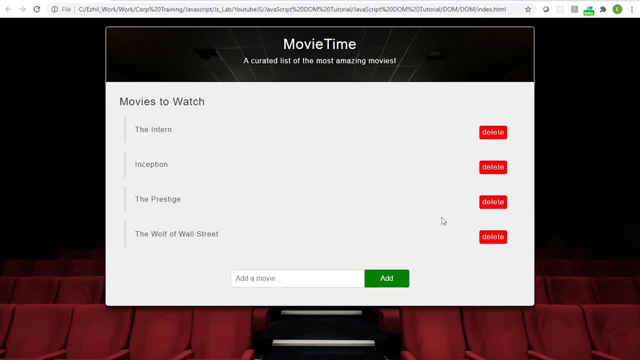 that we are just going to store in the page. so if you have to have these changes reflected, of course you'll have to connect it to a database. so this is what we are going to do, so using the Dom and using the JavaScript features. so how are we going to add an entity or element to your Dom? 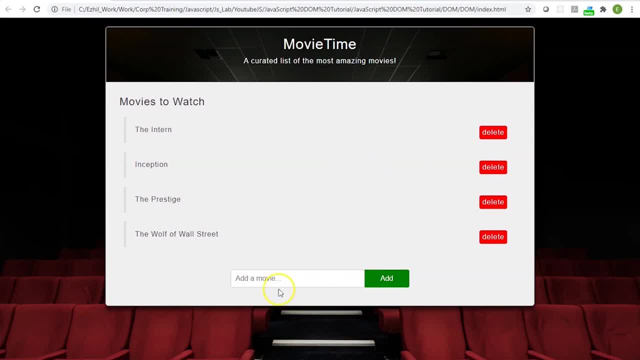 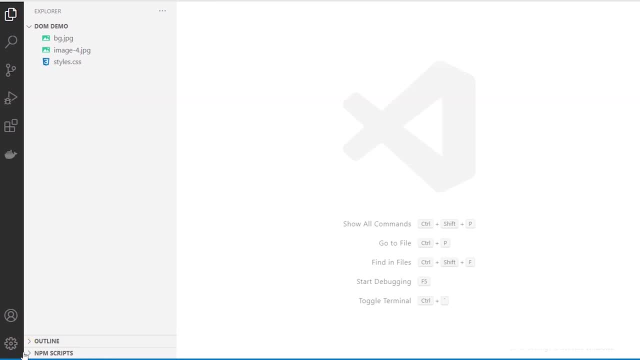 and how are we going to delete it. so this is what you can expect out of this demo. all right, so here we are in the editor. I'm using Visual Studio code, so this is the editor that I'm using currently. I do use other editors, like sublime. 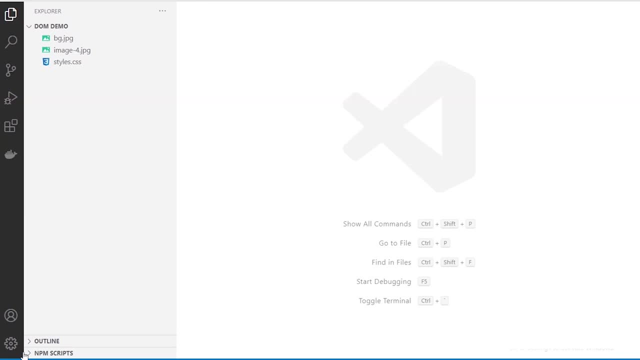 brackets webstorm. so this is purely up to you. whichever is the editor that you're comfortable with and you're already working, even if it is going to be notepad plus plus, or if you're from a Java background and you use Eclipse more, you can go ahead with Eclipse. so whatever is your editor, your preferred, preferred choice, you can go with. 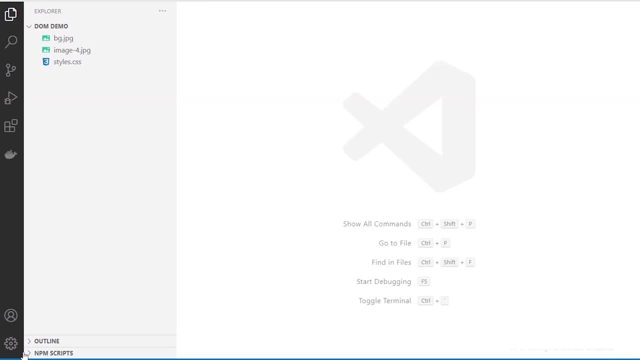 that Visual Studio code. I've been working since the inception so I have. I'm also from the dotnet background, so I've worked exhaustively with Visual Studio also. so here this editor is very comfortable. it is just not for JavaScript. it you also can use vs code for angular or react or python any other. 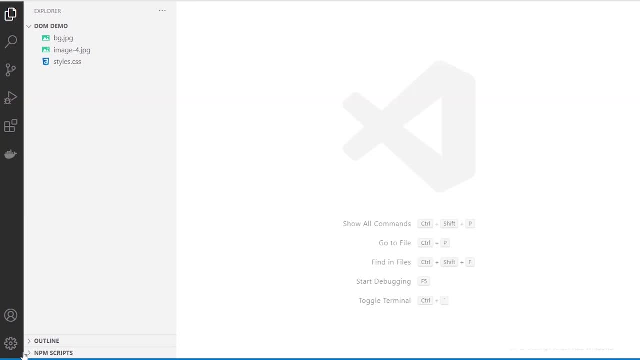 type of technology that you choose, any type of web development, you can use Visual Studio, so it has a very nice, intuitive and simple user interface and it has an integrated terminal, so where you can run your server also, and it has a very good debugging options with IntelliSense and you can install packages on the go and you can also use this. 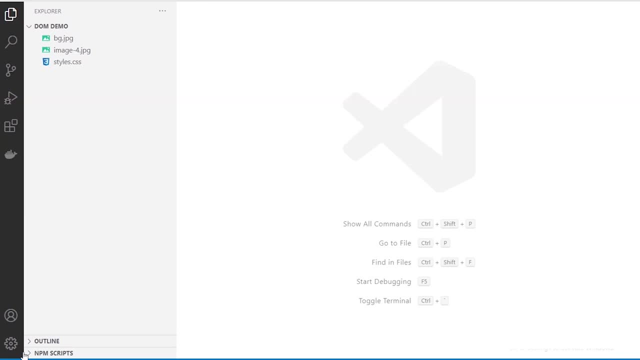 particular space for deployment also. so it's pretty easy and comfortable. so if you prefer Visual Studio and you're from that background or you have been using exhaustively for mean, stack or monstack, so you can use Visual Studio. otherwise it's completely up to your choice. 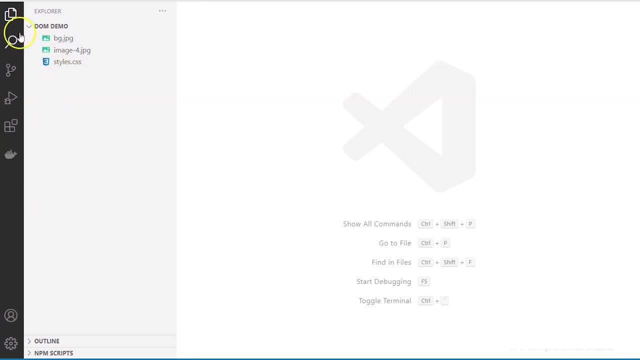 so you can see that I have a folder which is called as Dom demo, where I already have three files there, so two of which is nothing but some pictures. so this is the background so that I'll be using. so, if you could recollect, so I have shown you the web page with that theater background. so 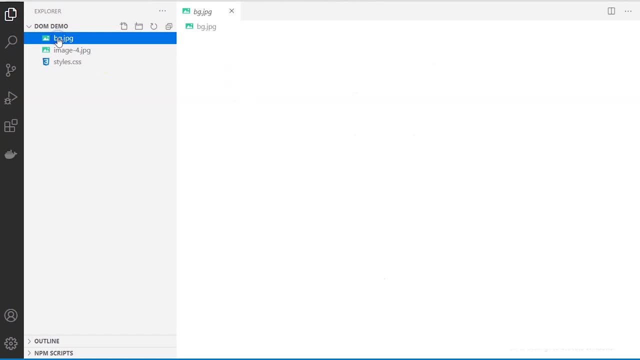 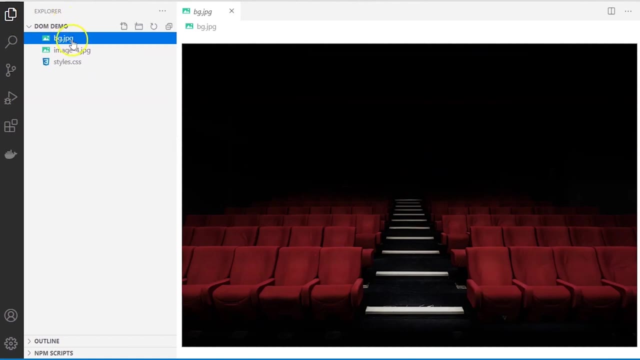 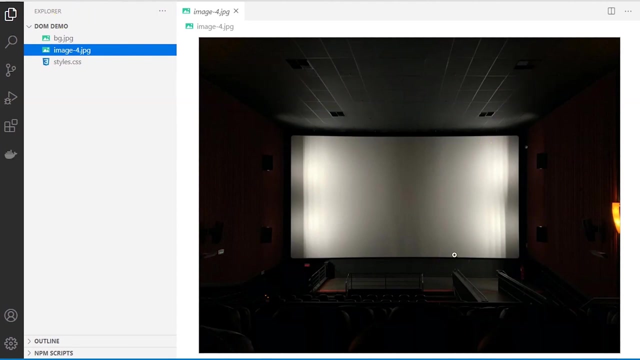 I will be using these two images for that, so you can take a look at it, so you can see this one. right, you could recollect that. so I will be using this for background and where I will be listing out the movies. so I will be using this image. I will not be using the entire image. I will be 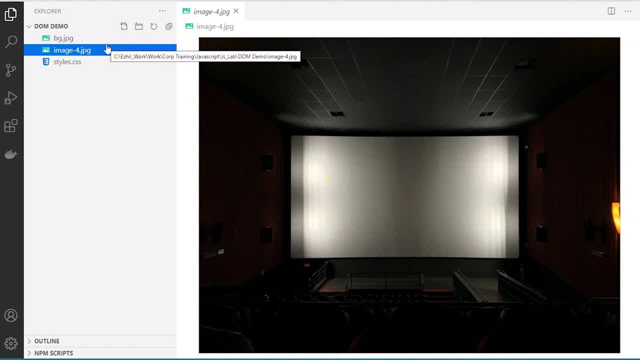 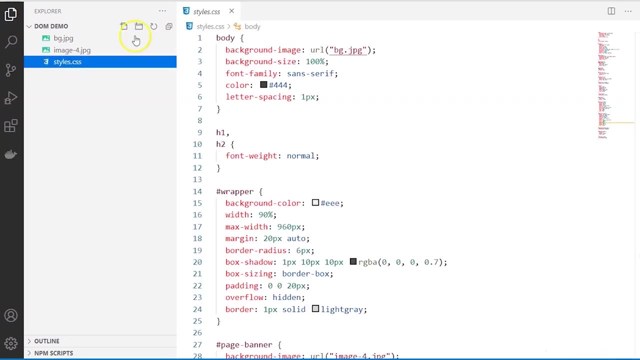 cropping and I will be using it and the all these style to use these images for other style features also for including those buttons and you know the rows, all these. I have used CSS cascading style sheet, and so this is the style that I will be including, so so I will not be. 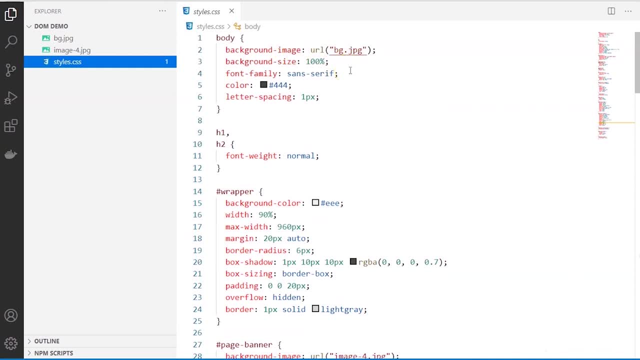 um, you know explaining each and everything. so I presume so you all have some basic knowledge of CSS and HTML. um, so what I have done, briefly, to get that style, I will explain it in a very, um, precise, concise manner so that, like you will get an idea like where, what feature I have included and you can explore on your own. 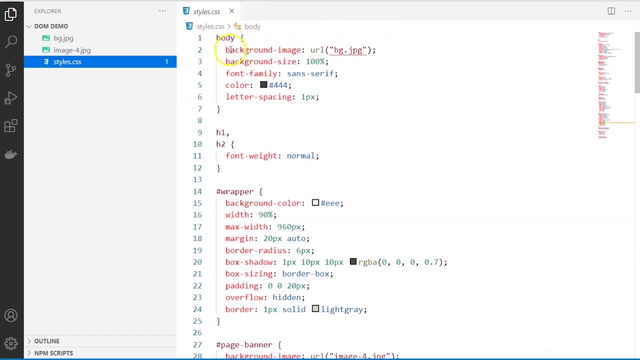 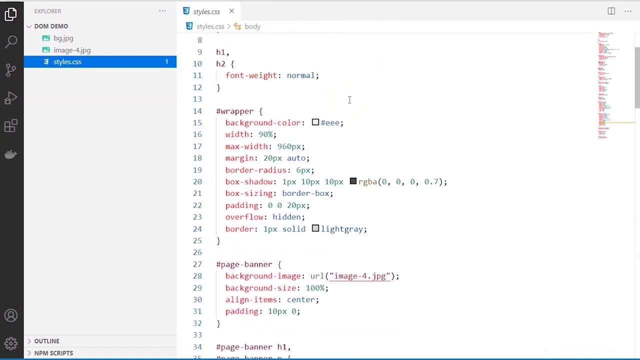 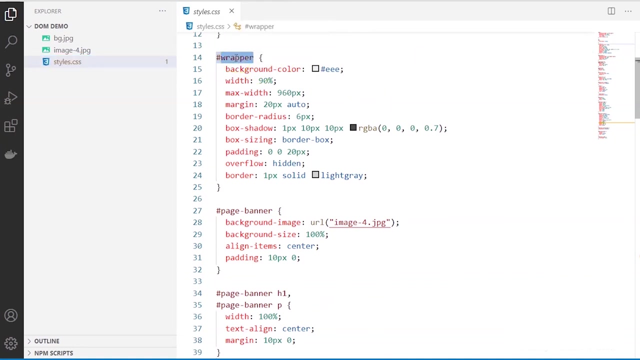 these style features so you can see that the background image I have added as this property and the size, font, family and colors and spacing I have set. this is for the heading, and so you should be knowing about different types of selectors, like ID selectors, tag selector, class selector. 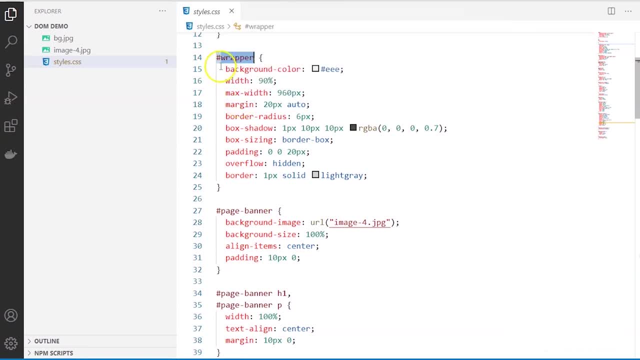 so this hash denotes the ID selector. so I will be using this ID selector when I'm creating my HTML page. so what I have done is, for that particular, I'm creating one container. okay, so for that container I'm giving a name called as wrapper. so where this? 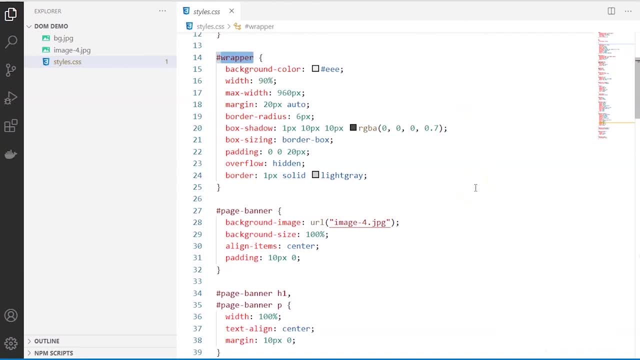 container is the one which is going to list out all the movies for us, so the margin padding border. now, these are very, very important. so if you want to have a evenly aligned, a readable, legible list or text or content, so you have to play around with these different properties of CSS. 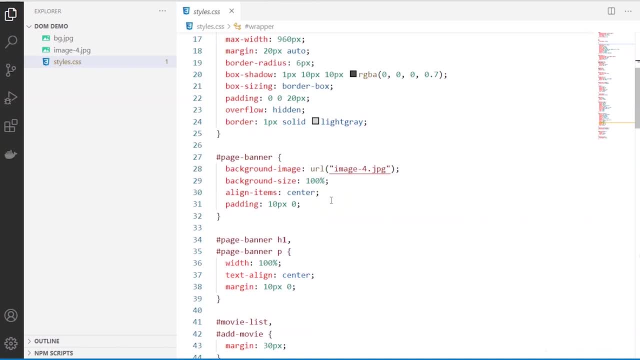 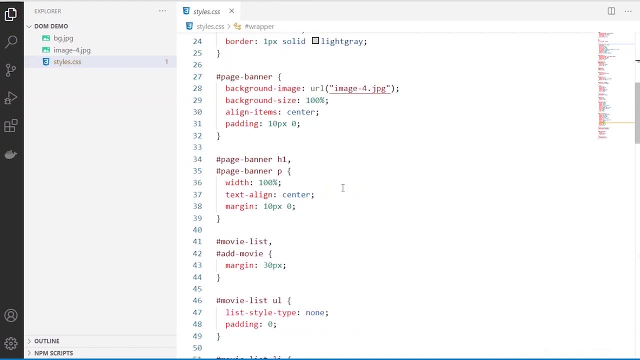 and you also can see that, um, there is a page banner, so this is the outermost container. then I will also be showing an image within that where the movie list will be displayed and within that I will be giving the- you know, the top movies, that list. so for that and the paragraph for the tagline: 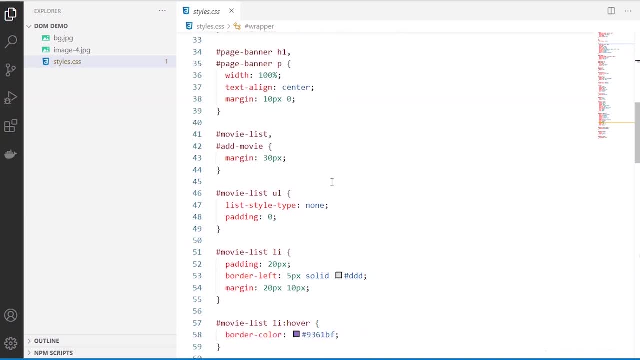 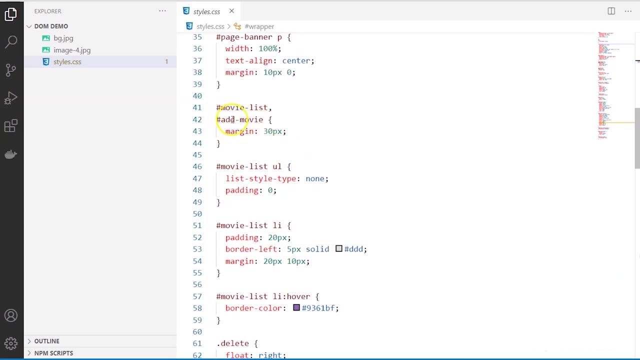 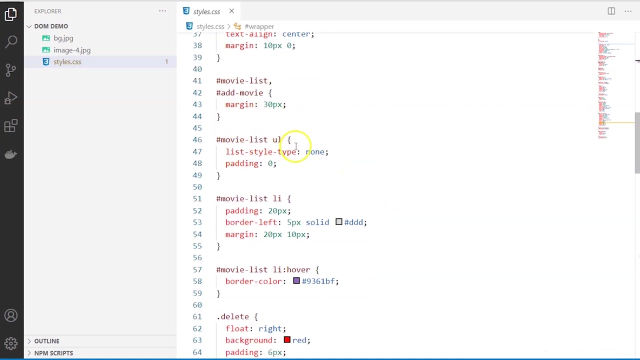 so alignment features and width and margin I have given. so you also can see that I have given certain elements with these IDs: movie list- and this is for the button ad. movie margin has been given there and the list I do. it's an unordered list, so unordered list. I don't want to specify any particular bullets. 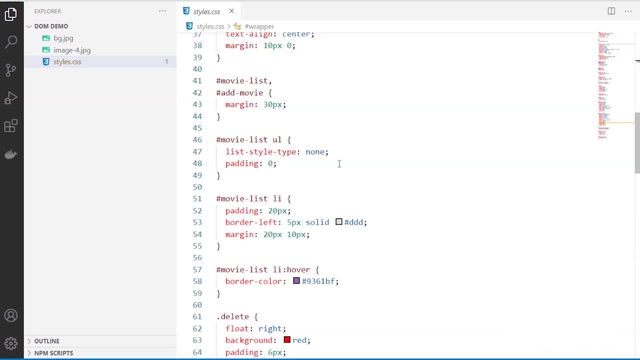 there. so ordered list will be having like 1, 2, 3 or ABCD, unordered. usually bullets will be displayed, so I don't want any bullets, so I am displaying that as none, and so this is the one I have used for the list items that you can see. 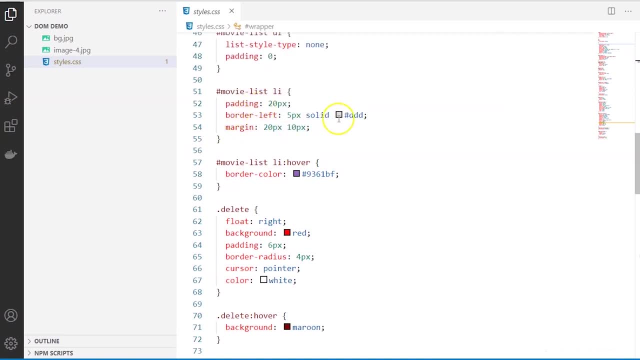 and by default, if I don't move the cursor, the border left. if you can recollect, I had one purple color, one right, which got highlighted only on the left border. so by default, I have made it, as you know, great so, but when I hover the. so this is. 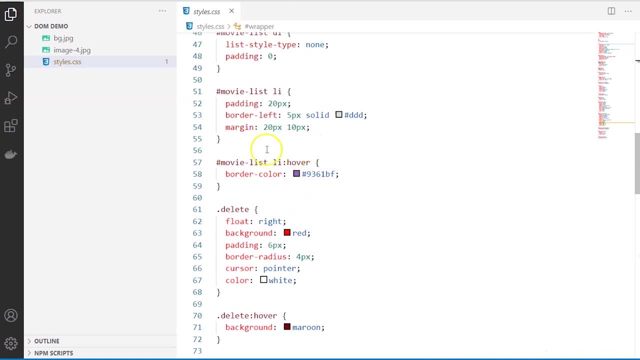 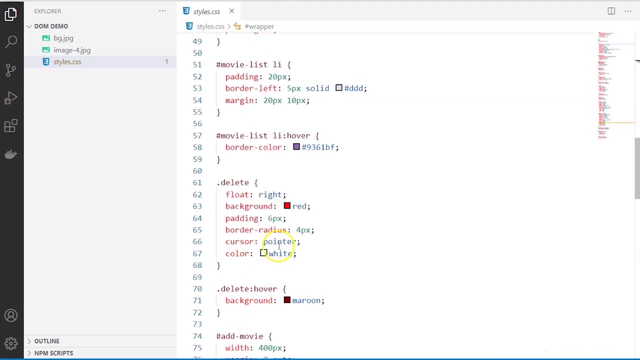 the pseudo list. so when I hover over it, so the state it gets changed, so it becomes the color becomes purple here, and these are the style features that you can see for the delete button. so this is the delete button, so it's a class, so that's where it has this period symbol, and so what are the difference? 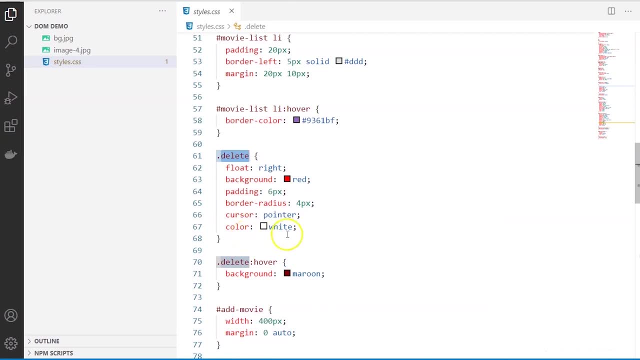 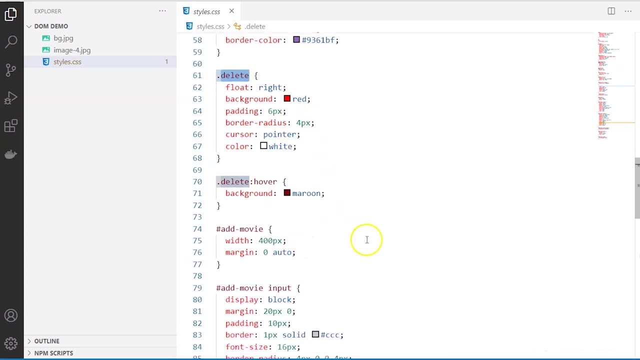 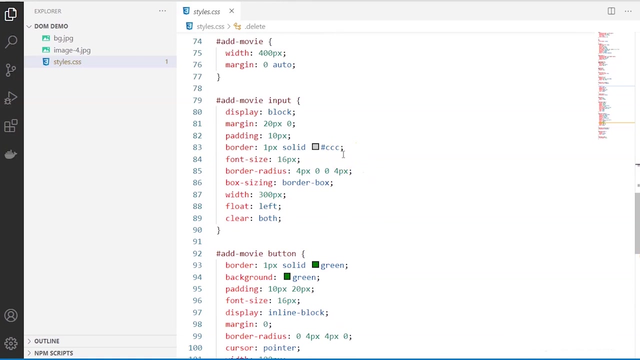 so it has a radius, it has a rounded corners, that button, and the text is white. so all these and again, like when i hover, so from red, it changes the background color and you also can see. um, this is the style for the add movie button. you can see. 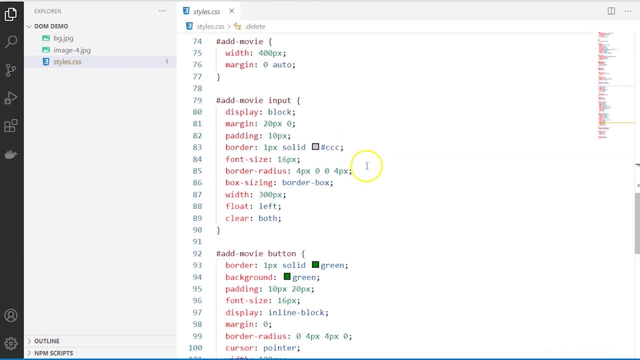 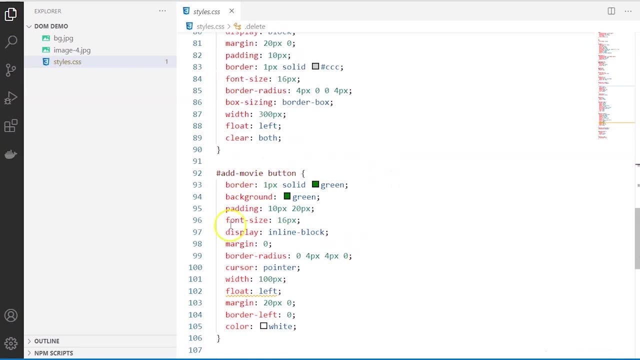 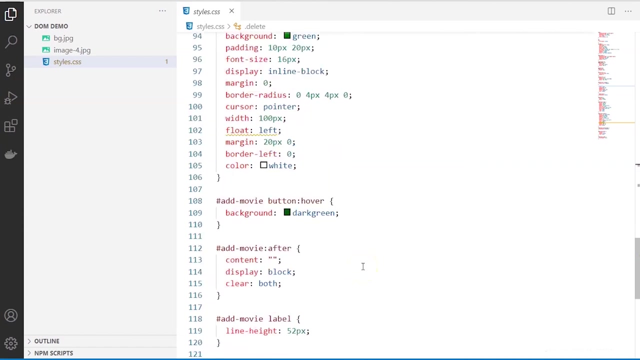 that. so this is predominantly, it is in um gray color, and so this is for the input, which is your text box, and this is this is the add movie button, so this particular button, so i have made it as green and you can see the other features also and again. so, however, it becomes like a dark green. so 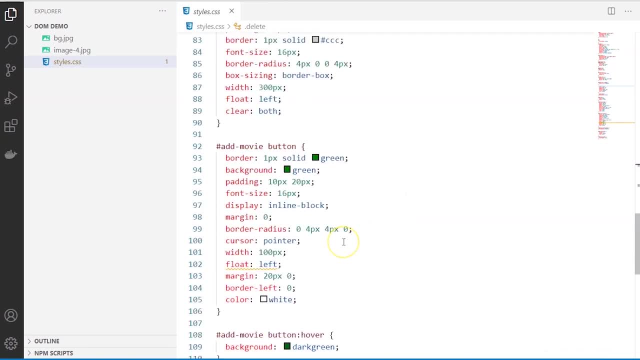 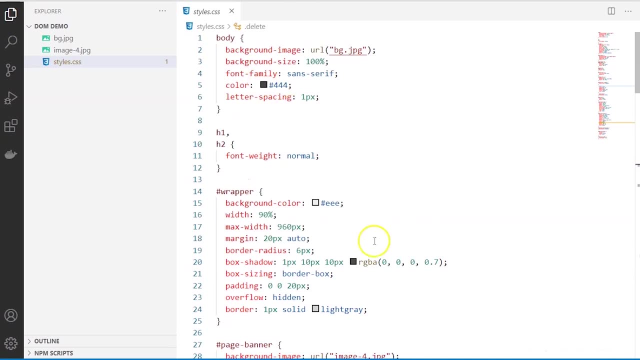 these things and all you can change right, and for these labels, so for all the elements, um, that i will be creating now in the indexhtml. so this is the style that i'm going to apply, so you can go ahead with your own style. there is no restriction. so you can change the color, the alignment you want to change the. 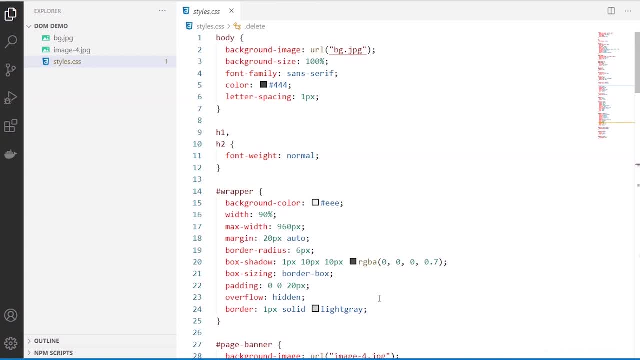 um the background layout, so completely up to you. so our focus is not css, uh, for this particular demo, so our focus is on the javascript's don manipulation. all right, so let's start creating our webpage. so the first step- how do we create our web page- is by creating a html page. 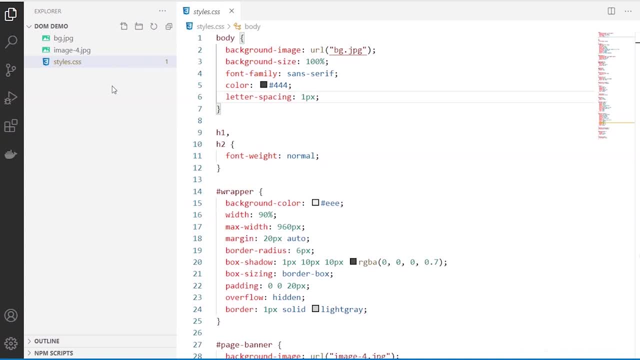 after we create a html page and set those content- you know the list of movies- we'll try to create, uh, the most important file, which is your javascript file, and we will connect all these together to your html file. so we already have the stylescss in place. um, so, after we create, 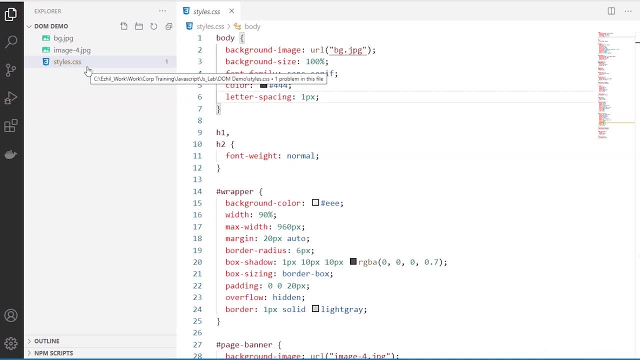 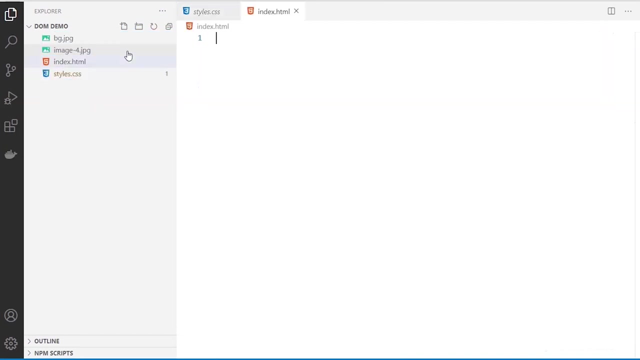 our html page, we'll be creating the javascript page also and we will be connecting all these three. so here you can see there is an icon which states new file and so let's give this name indexhtml, and you can see the icon gets magically changed over there. um, so i have a corresponding. 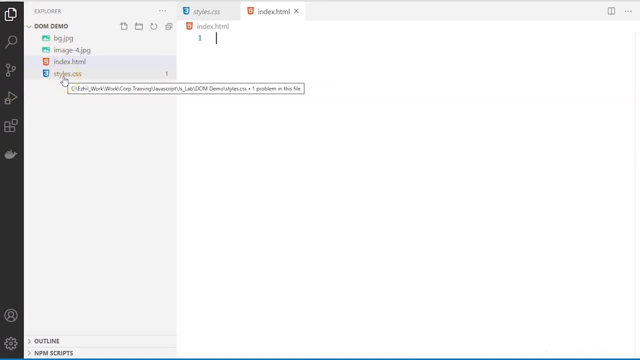 uh, you know uh extension, uh file, which actually gives all these uh extension. the logos will be automatically updated. so you might not be having that uh by default. so if you want, you can just go ahead the DR these extensions. you can see that. so you can see this. this is the one that 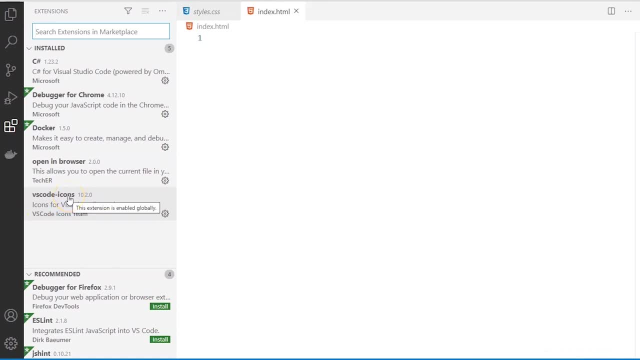 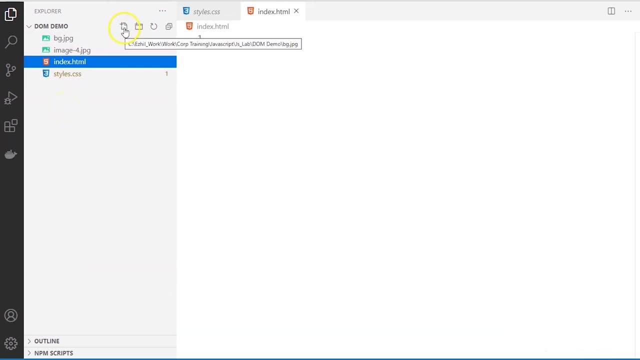 i have already included these code icons. so if you want to have those logos so that you have a clear picture of what you're creating, you will be able to do it. so here we also can create, which is your app dot js. this is the one that you will be creating next, so you can see this. 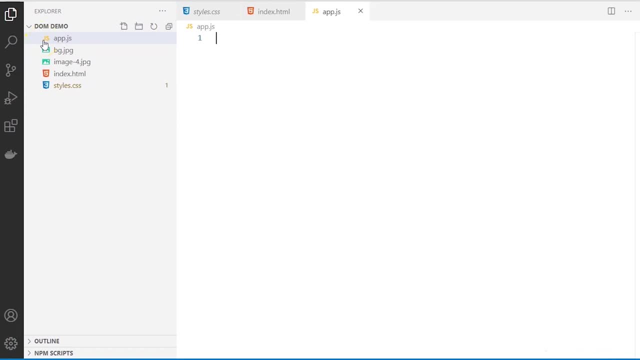 js icon also pops up nicely. so by default you might not be, uh, seeing this icon, so, but if you have that particular extension, that file, you should be able to see it. all right, so inside my um indexhtml. so let's start with our coding. so first thing, so you can see that very nicely, this: 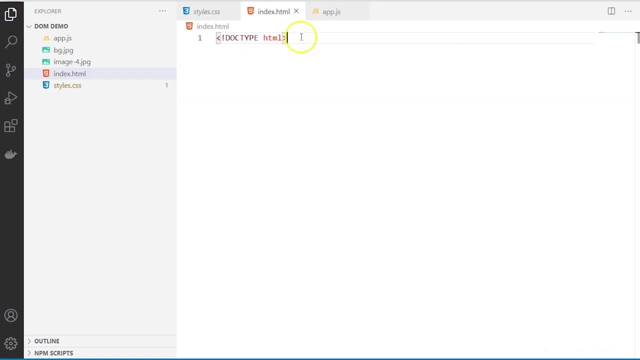 intellisense is also popping up. okay, so here i say that it is a html5 document, so the html document. earlier we had html4 version for many, many years. so recently it was upgraded um w3c, which is our world wide web, upgraded that to the next level, which is your html5. so here 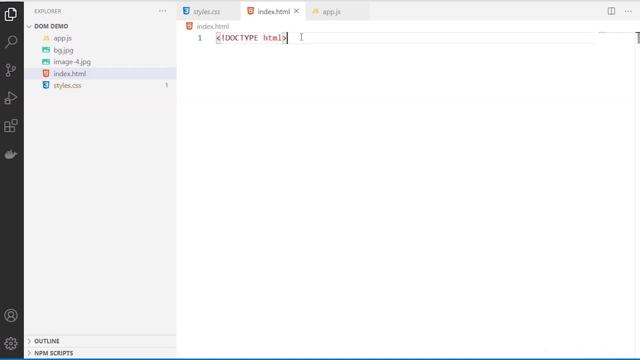 this particular the first line, where it denotes the html5 name space. it's much more concise and precise now. otherwise, if you know about, if you have already coded in html4, you will know the pain of writing that you know lines and lines of that namespace. so the first line indicates that it is a html5 document. so now we'll have to specify the. 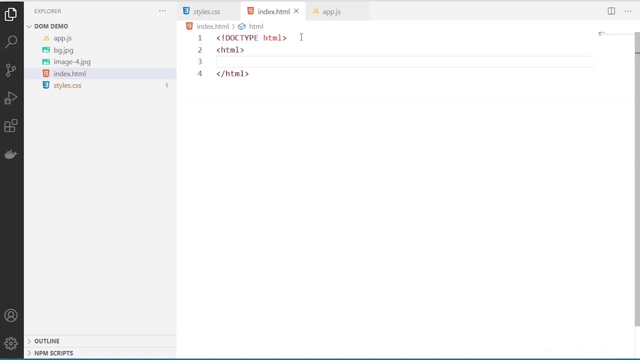 root element or the parent element, or the outermost one, which is our html, so all our tags and elements goes inside this html tag. so we have this head and we also have the body. so so head, as i told you earlier during the discussion, so where i was saying that all the metadata and other properties, 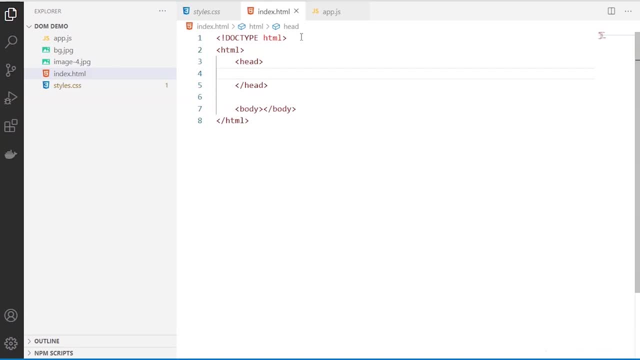 like your title and so if you want to link other files like your styles or your script, everything inside your head, um. having said that, uh, you also can include your um script src anywhere inside your body also. you can have more than uh one script source also, not necessarily that it has. 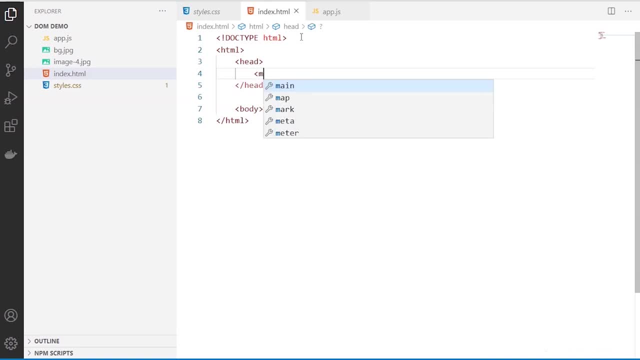 to be inside your head only, but we specify some metadata and other um within your head elements. so here i'm including one character set here, so this is the default one which is your unicode. okay, eight, so not mandatory, but you can include this one and, as i told you, we can also. 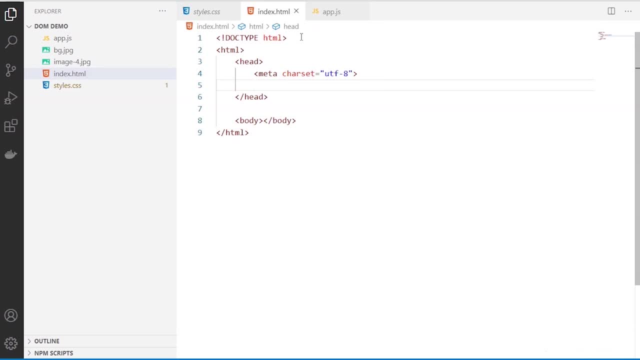 include your style and you also can include your script, but we'll do that later, so right now i'll just include my title so which will be displayed on the web page: uh title bar. on the uh top most one that you can see, i will say: title bar: a s vit time right. so now this goes inside the head. 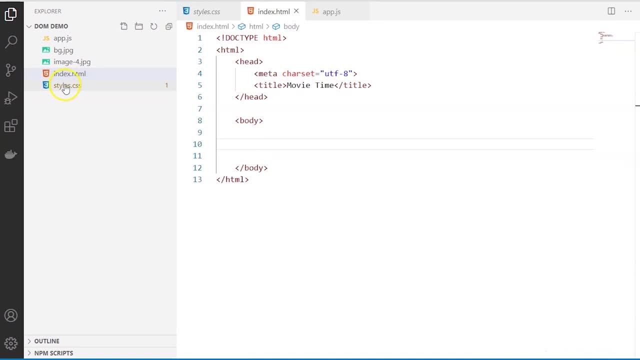 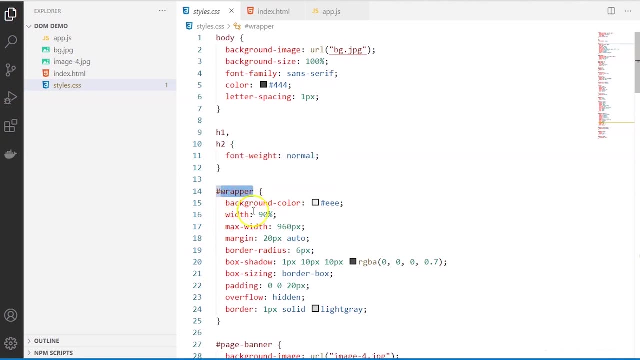 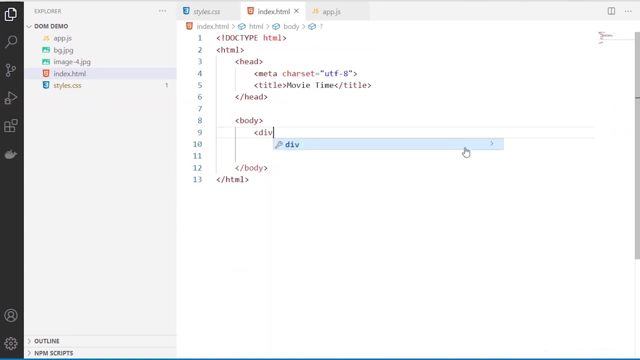 inside our body, as i told you while we were going through this style. so we have already created this outermost contender and i have given some name for that, so we will be using this in our html content. so where i'm going to create a dot and all the id, so will be represented as an 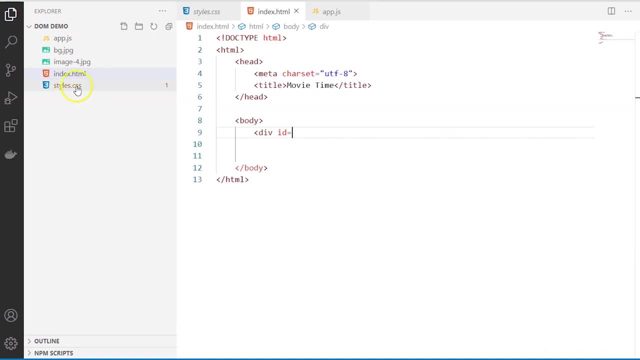 hash that you will be using in your CSS. So you can see this one, So I've used this hash. It means that we'll have to use an ID over here, So let's say, wrapper. Now, this is going to be my outermost. 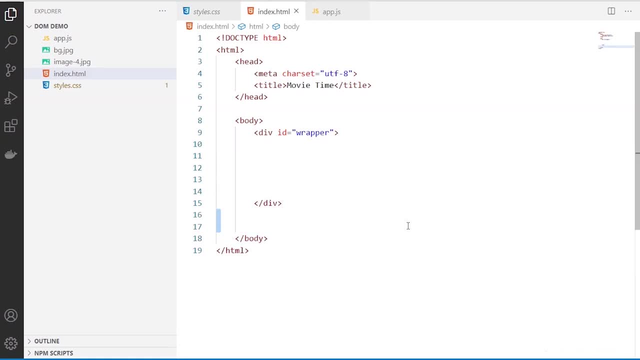 div and all other elements are going to be present inside this div. And inside my div I'm going to have a header- So this is a HTML element header- and inside this header I'm going to have the title, So, which says movie time, and it also has a tagline I showed you. 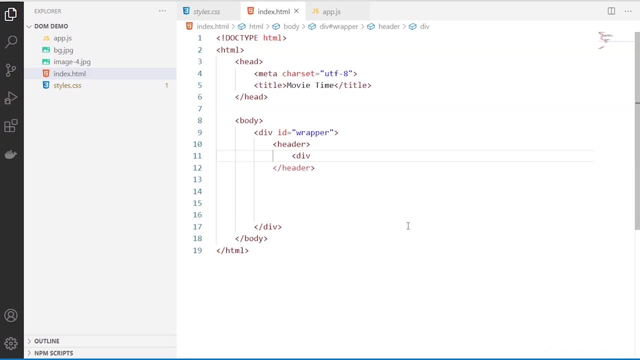 in the finished web page. So those movie title as well as the tagline, I'm going to include it here. So inside my header I'm going to have this 1 more div and I've already created the style for this, So this will be the. 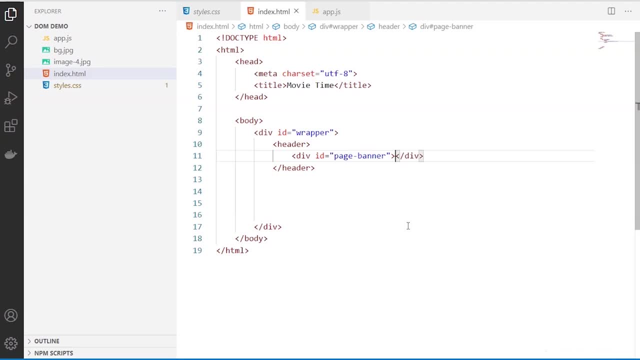 page banner and inside my page banner I'm going to have this title, So the movie title. I am going to use H1 over here and I'm also giving the class because I've already defined And you also can see here that I'm already made a title. It's not a video title because what you see here is alak cut fetal and you be also giving that class because it's already defined and you also 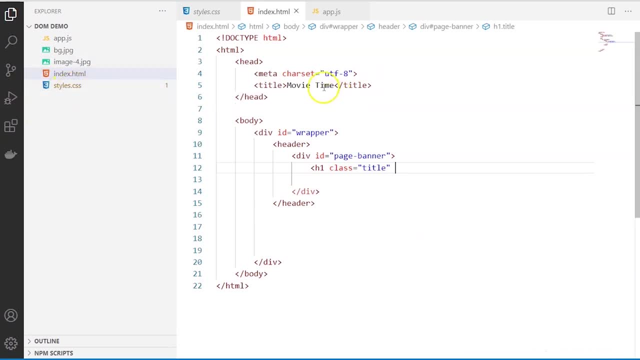 can define the style outside, or you can have a style inside the head that you can refer. So in that case it would be referred as internal style. Now, this will be external style, but if you want, you can also have an inline style. Say, for example, I can include a style property here, So this will. 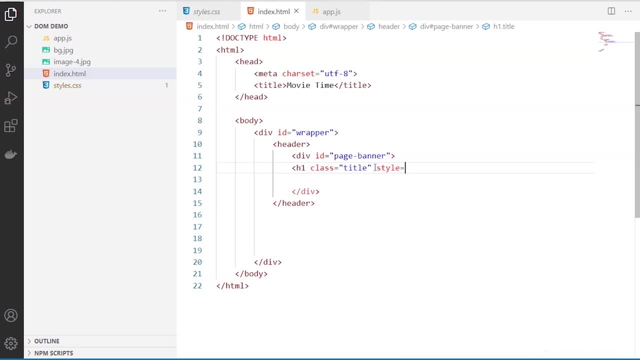 become the inline style of H1, which will have the highest precedence. So in this I say: I want to have a white color, so you can either pick from the text as such or you also can give this hex value, So both are same. Then after that, so all your CSS properties are terminated by a semicolon and it's: 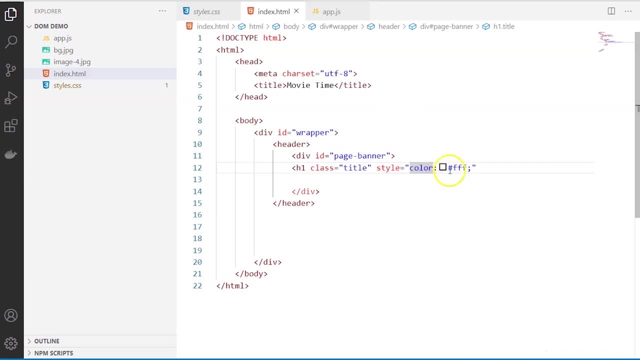 a semicolon. So all your CSS properties are terminated by a semicolon and it's a semicolon. So all your CSS properties are terminated by a semicolon and it's a semicolon. So here you specify whatever is the heading that you wish to display, And next we will be giving the tagline. So let's. 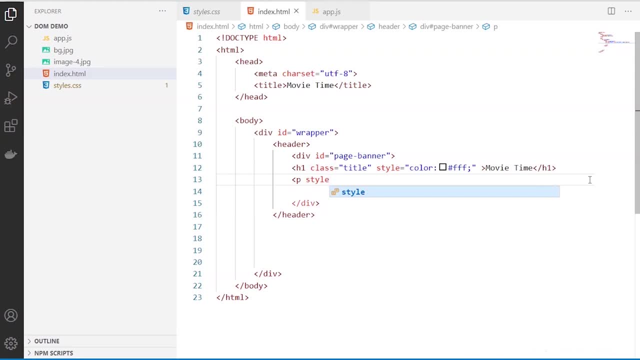 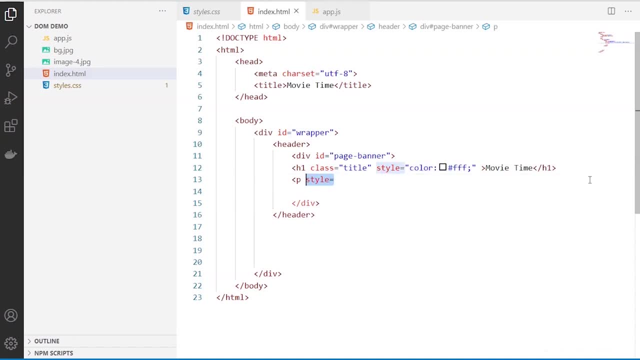 background. so we are using the white text here, So I'm copying and pasting it here. Yeah, so here. so you have to close this here, let's say: curated List of most amazing movies, So you can write your text like however you want. 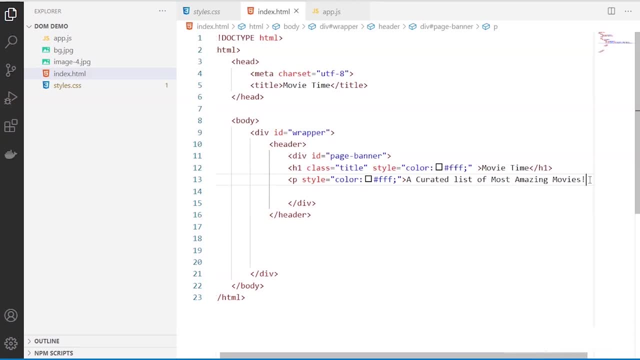 So, however, you want to display those taglines and the title. So I'm closing my paragraph here and I'm also giving a break there. So, with this, this particular div, which is the page banner, so this is over. So I've created this page banner just to display. 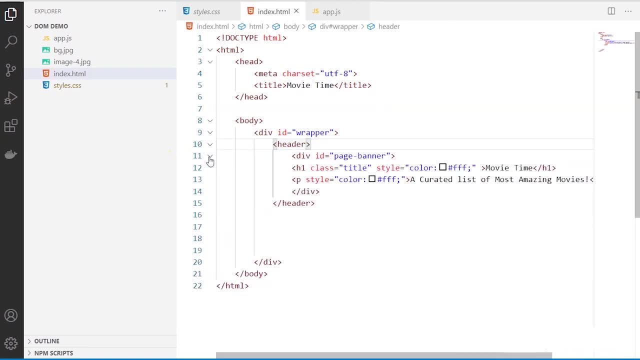 This is the entire thing, is your header you can see. So this is your div, which is your banner, and this entire thing is my wrapper. So I still have my list of movies that will be coming up here in this section, So this will be the title and the tagline. 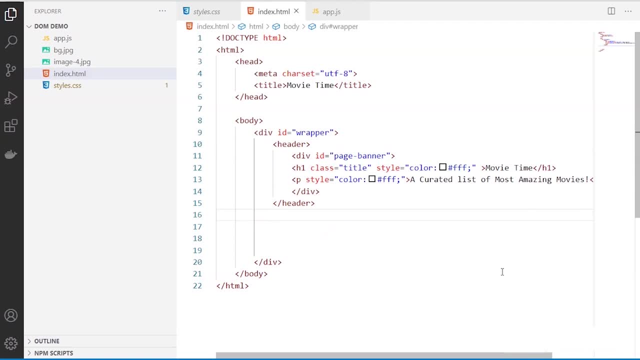 So after this, After this header, I want to include a div which is going to be my movie list- So we'll call this movie different list- And inside which I'm going to have the title again, something like a subtitle. So I'm using my HTML. 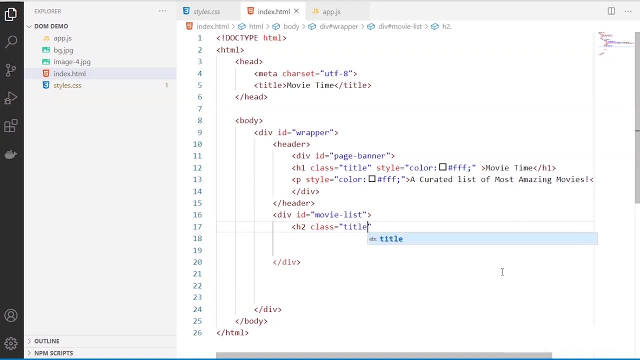 So where I say again, I get this title, class so which will be used in styling And within which I will say movies to watch, So this will be the title for the list, So, after which we are going to include our unordered list of movies. 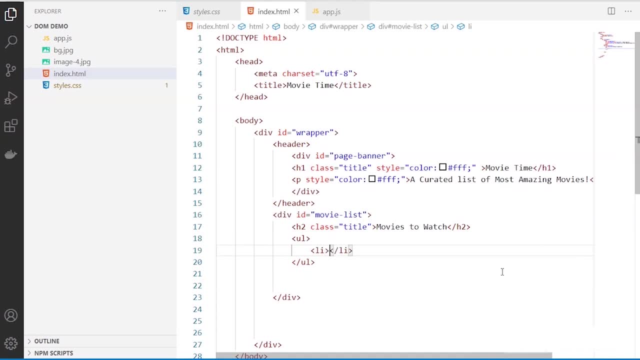 Now inside which? Inside The unordered list. I'm going to have now see two things here. If you could recollect the movie page that I had shown, We will be creating the name of the movie in the row wise format and it will also be. 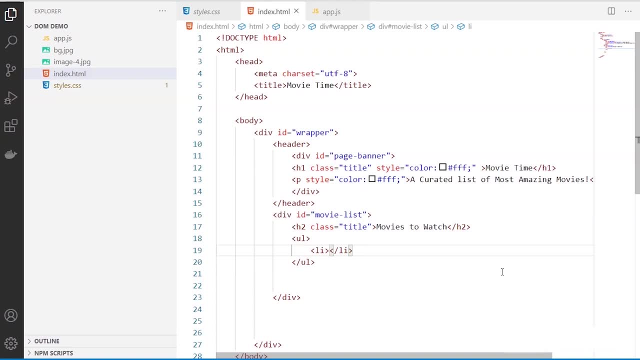 having the delete button So you would be able to see that the delete button would be there, And so both elements have to be there For each movie list. So I will be specifying the name of the movie here And I will also be specifying the delete button. 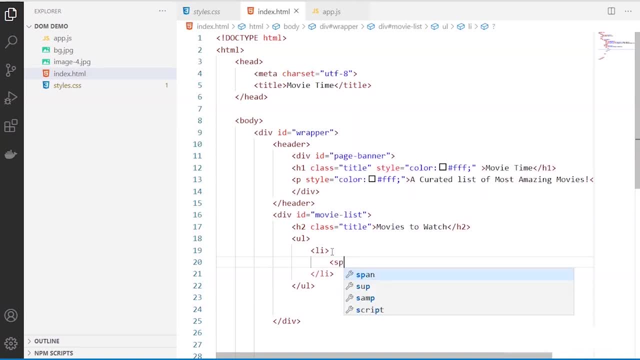 So inside my list item I'm going to have a span. Now this span, So I'll say so, it will have name and where. let's include the first one. So I'll say So, it will have name And Where. 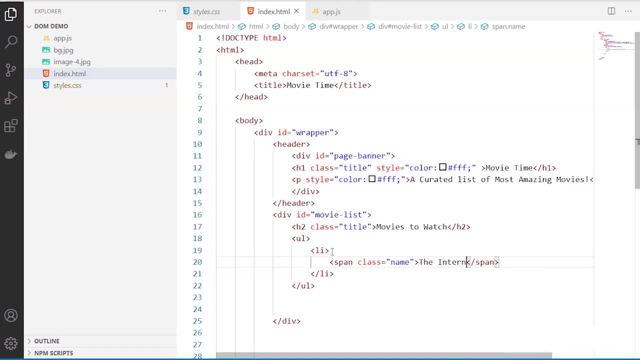 I've done and I will be including a span element for the delete button also, And I will just say, Okay, So let me copy this one, because we are just going to use this for all the, this particular style, for all of movies. So I'm copying this: 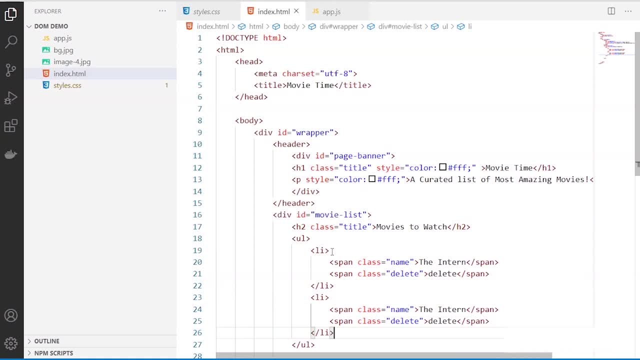 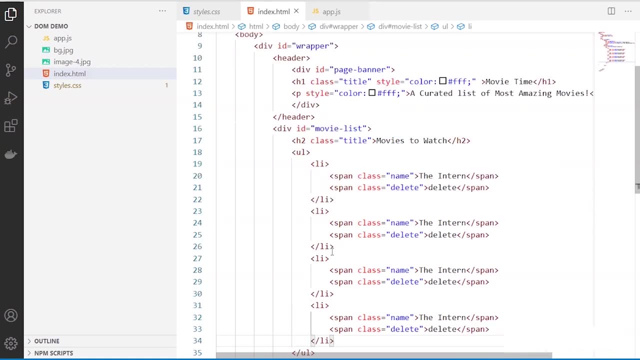 And then- And I'm pasting maybe 4 or 5 movies, so 3,, 4 and 5.. So let's write whatever movies that you want over here. So let me just change these movies quickly. So all of my favorite movies: Inception again. 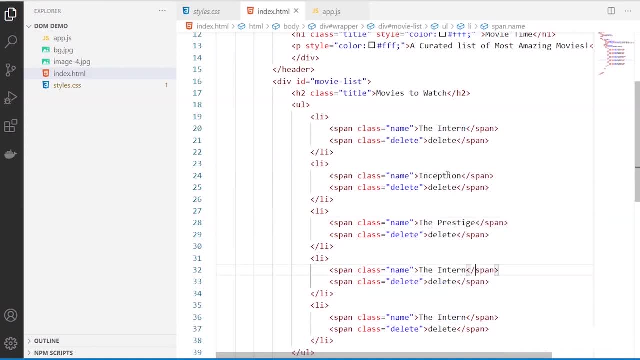 And Love in the Middle And Stage right. Alright, So the last one. Maybe I have included one extra, it's ok, The Avengers or Avengers, ok, whatever. So we have included this movie Now till then, thank you very much and good luck. 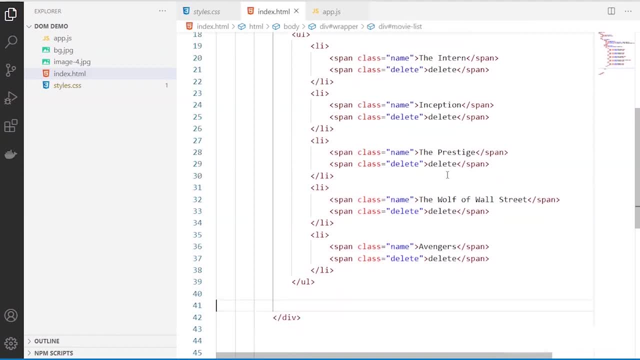 five movies now. so with this, this movie list is over. so now, next, what we will do is we'll have to do one more thing before we move on to JavaScript file. so in this one we have to create, we will be having a form element here, the main reason being we have to include a submit button so that I can inform the. 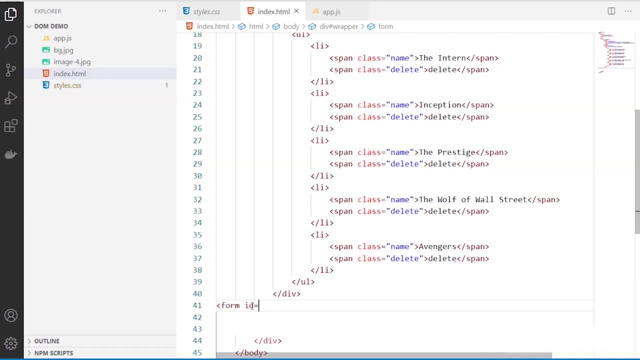 JavaScript module or the function, so which can handle the addition of new movie. then I have to click on the add button here, so I'm giving a name for the ID, so this will be the form, so which will be the parent element, and inside the form I'm going to 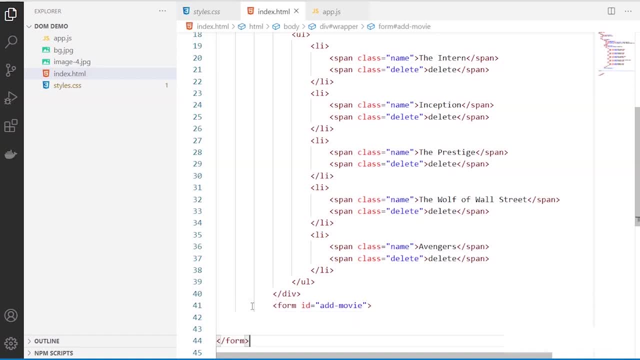 What we are going to have is we are going to have the button and also the input box. So the input, the text box, we will be including so you can see the list of input elements of your HTML. So we will be selecting text. 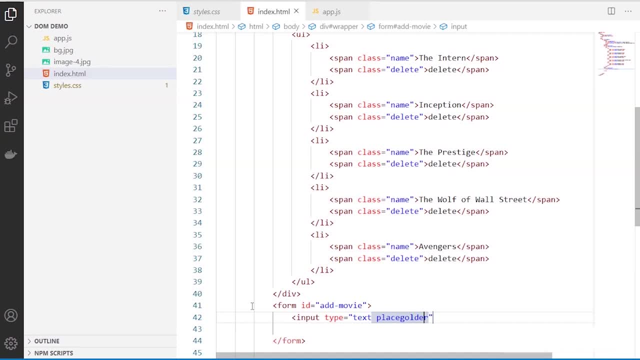 And we can have a placeholder, it's nothing but the text. So where I can specify: okay, so this is this- should not be inside. This is text. So the placeholder property where you can give some hint of what is supposed to be entered. 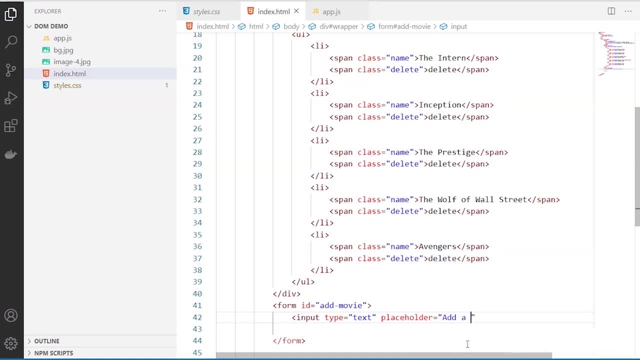 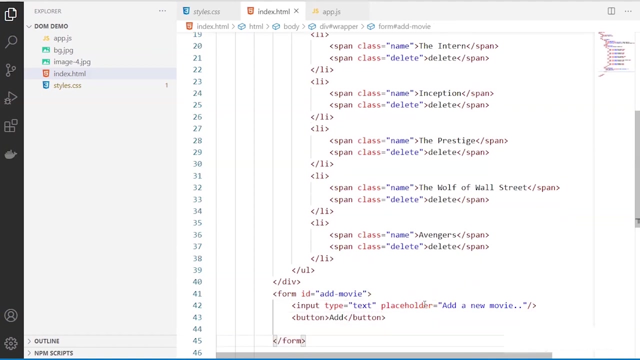 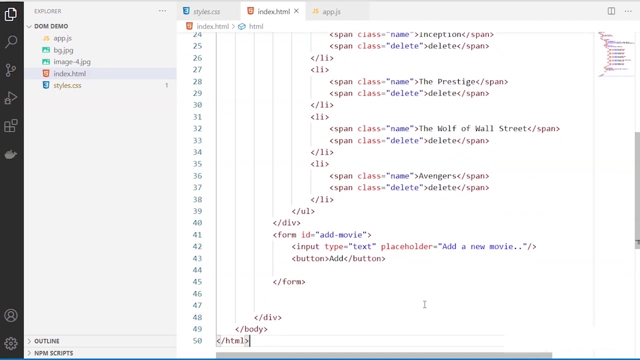 in that text box. So I'll say add: So let's close this input box. Now this button let's add: So now this is going to invoke the function which we will be adding in the JavaScript page. So with this, we have closed this form and we have also closed this div and body. 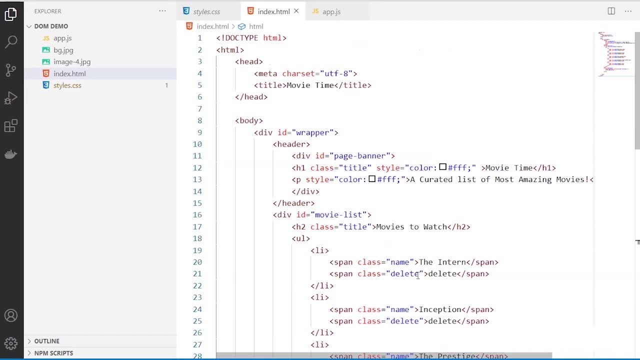 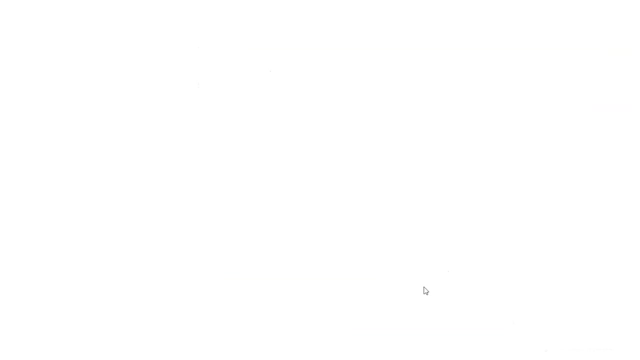 So with this, the HTML content, Okay, The code for the HTML content is ready. So if you have to see this page, so I have this option set up here, So open in default browser. So when I click this one, okay, so you can see this. 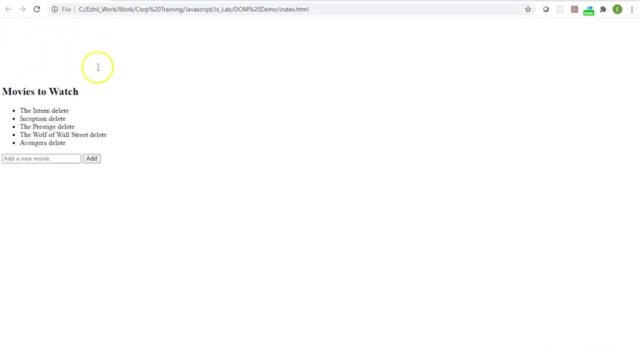 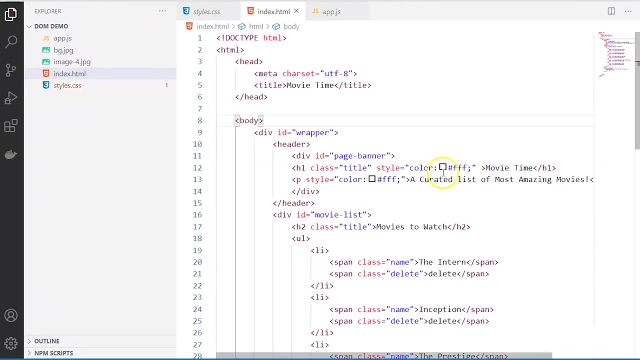 And so if you're wondering, why is this blank over here? you can see this here now. Yeah, It's. the main reason is I've given one Okay, I've given white text because we'll have to include the style. We have not included the style yet. 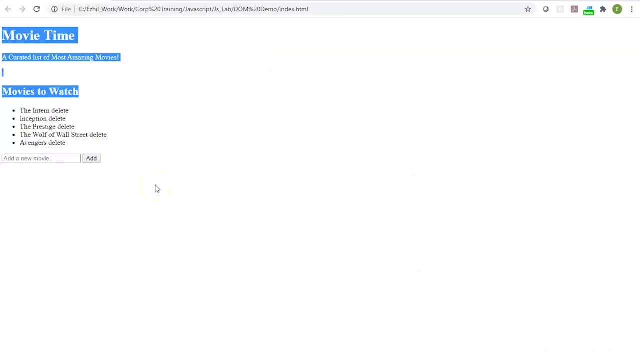 So just the HTML content. it looks like this. So it's not. it doesn't look so great, I know. So there is no JavaScript function also, But we can see that whatever content that we have mentioned, so it has been displayed. 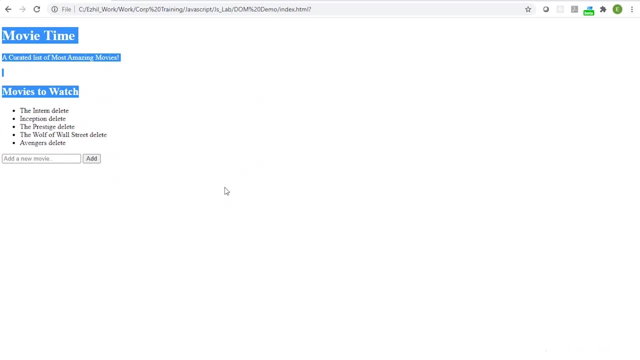 properly. So the next step for us, For us to do, is to add the CSS and see if it matches the style that I had shown earlier. So if you have to add the CSS, so let's see. okay, so we have now seen before adding CSS. 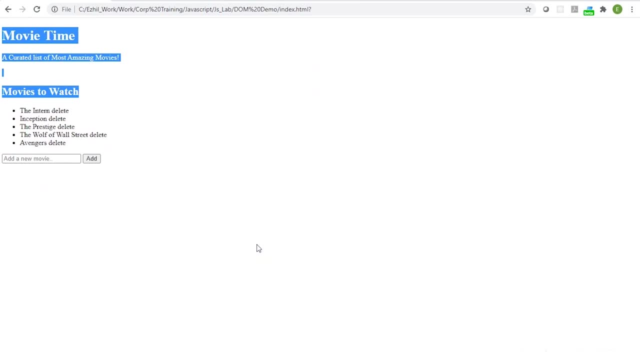 So I keep saying about the importance of the style and theme also. So I know your content is ready, but it doesn't look so attractive. So how could you make it so engaging And so that the probable customer or your business user can start using your web page? 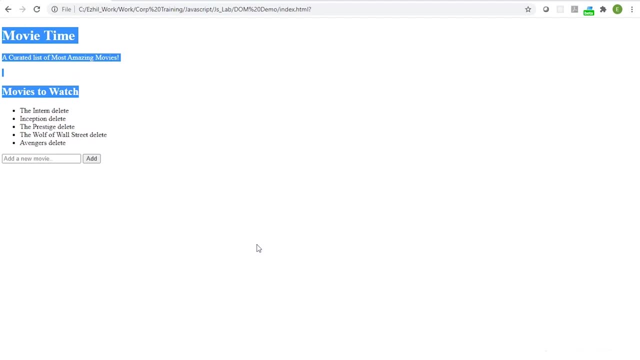 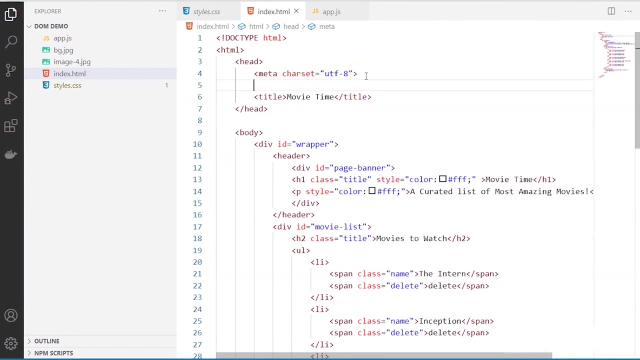 So how can you make it much more engaging and attractive? Let's add the CSS and see if it creates a magic or not. I know this is not our prime focus, but CSS definitely helps. So the link is the Tag that you will be using to specify the reference. 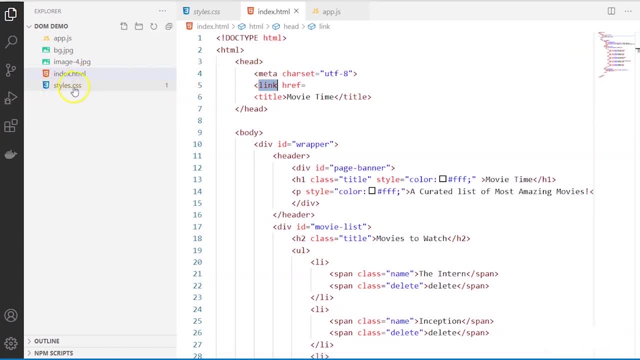 So this is the reference where I have to add: So, whatever is your CSS style, So this is an external style, So I use my HREF property to attach this external style here. So I'll have to include so you can see that it gets listed. 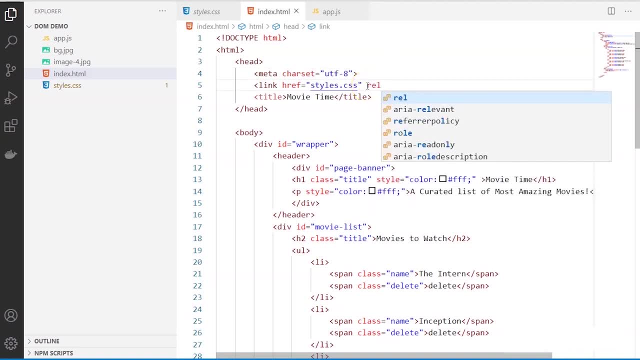 Yes, And it's not mandatory, but still, you can mention That it is a style sheet. So CSS is the default style sheet and JavaScript is the default scripting language for your HTML. So we have attached this now. Okay, So let us see again. 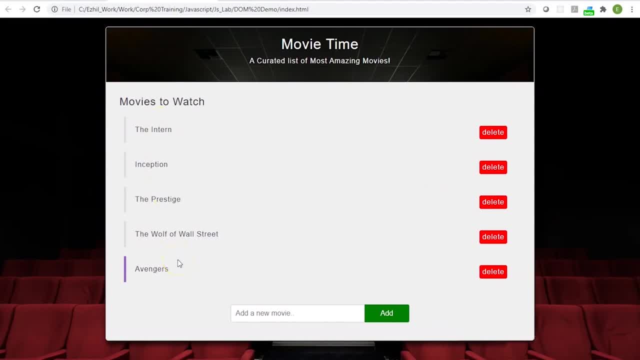 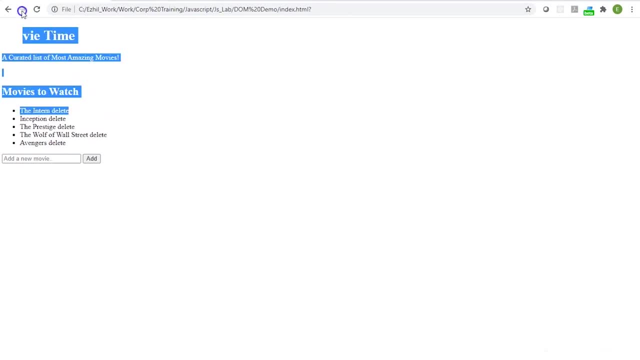 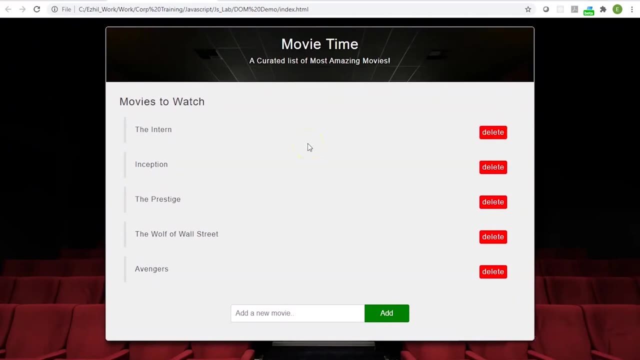 Okay, Look at that now. Look at that So you can see this before CSS. So, literally, it is nothing, it doesn't look like anything at all, but you can see like after CSS. So if you are, if you have fancy taking for your fonts, if you love fonts, maybe you can. 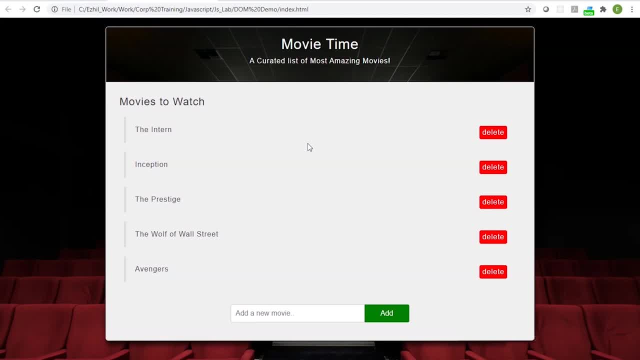 change all these fonts. I've used some default fonts, So how would you want? you can go ahead and change it. You can see that whatever we have given in the CSS that I've highlighted, It's now on the default font. So you can see that. 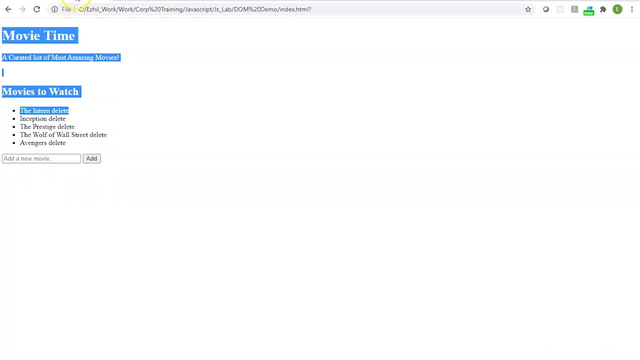 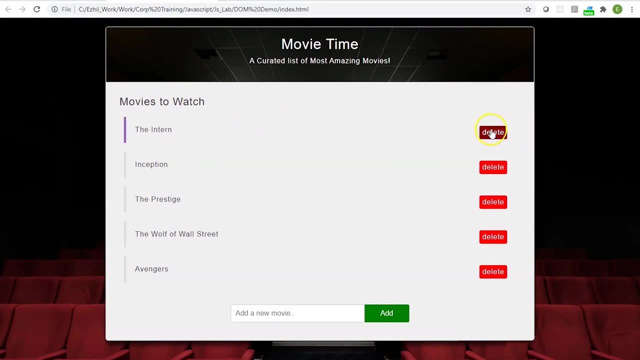 It's now getting reflected in this new page So you can see the difference between this and this. So that's why I opened another tab for you to show the see the difference, but nothing is going to work. So you can see that the hover, so you can see the red, is changing into maroon and this: 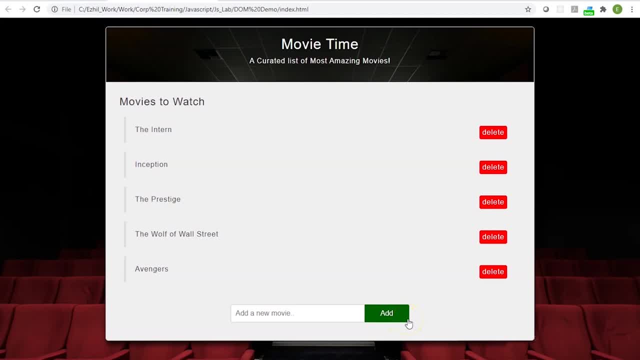 maybe not much of a difference, but you still can see. I would say, if you're using CSS, don't change those text size and you know the alignment and placing, because there it the effect that you will be getting there. it will be like 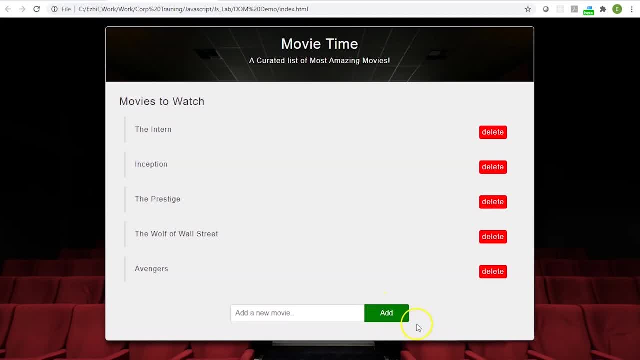 flickering a lot and it will be. the alignment will be an issue. Always change the color or some highlight those things, not the size and alignment, So you can also see, like, how nicely these rows are getting highlighted. So now, whatever we add, so nothing is going to be coming on because we don't have a JavaScript. 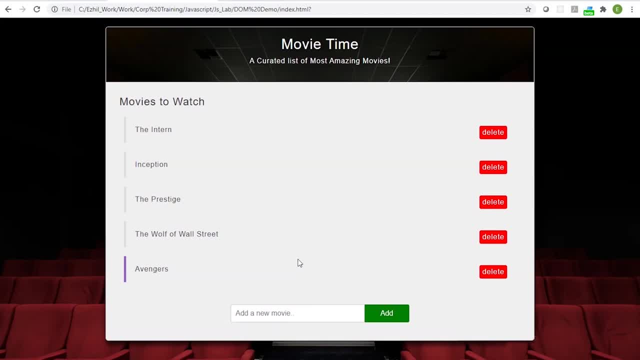 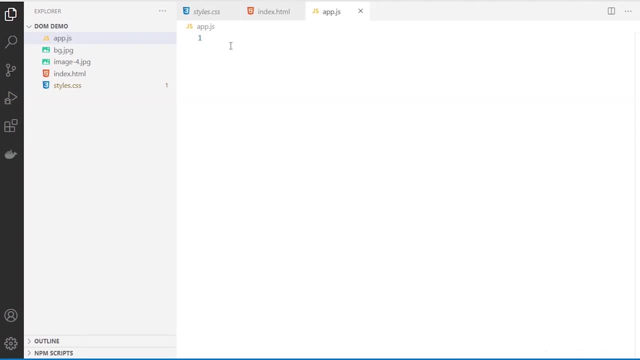 functionality yet. So that's it. So that is what we are going to see now next, So let's start our JavaScript coding, which will be the next module. Now let's start with the appjs, which will be your JavaScript file that you will be including. 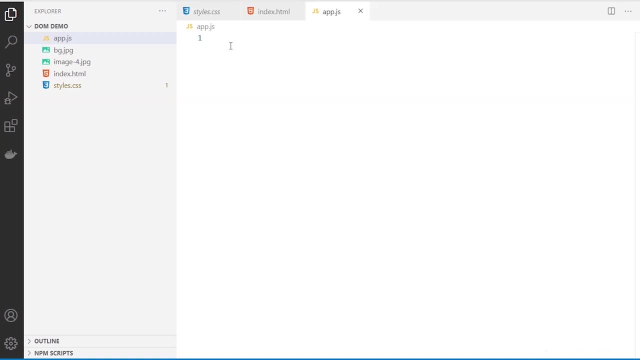 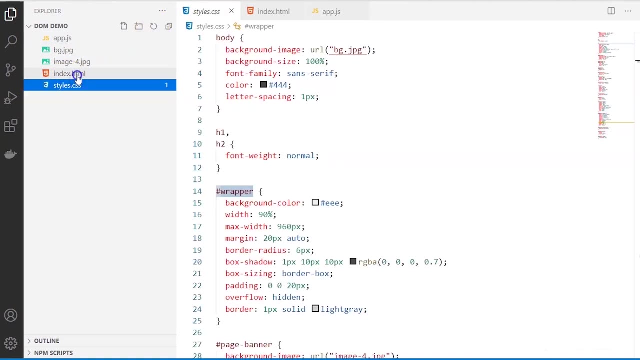 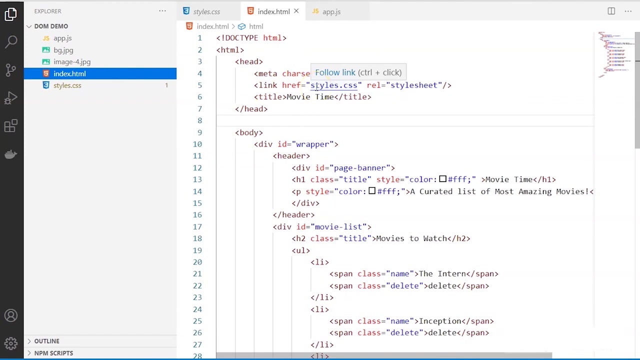 and coding for DOM manipulation. So this appjs file has to be integrated inside your indexhtml. So, how we have integrated Our style, we will have to use another element, which is your script, and we have to include SRC instead of href. 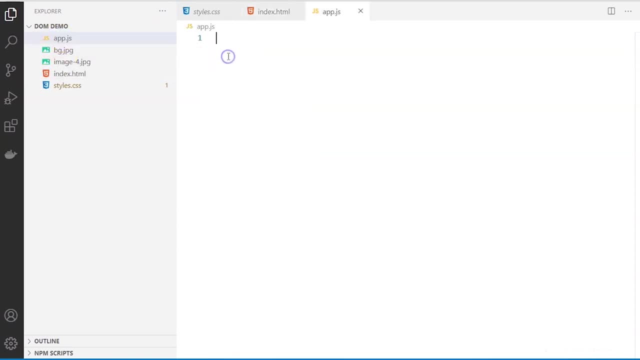 So that we will do it later. So now let's start creating this code for the appjs. So let's start with this document element and we will have to do the coding for one of the event. So we'll be writing those functionality. 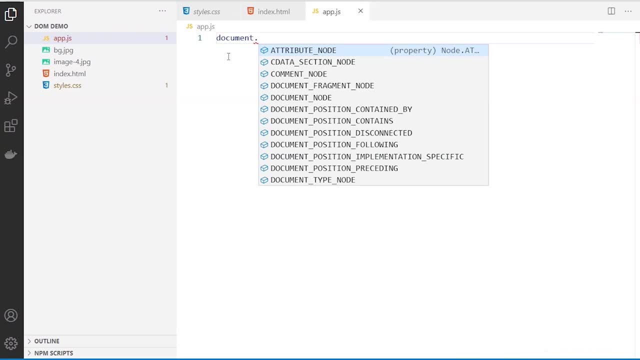 So let's go ahead and create the event and attach your functionality for that particular event. So there are ways, different ways, by which you can do it. An event listener is one of the ways. So I can specify. So, as you can see, in this internally sense, this purple color box indicates that it is. 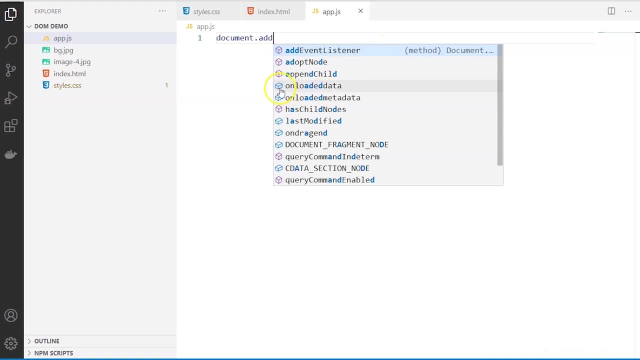 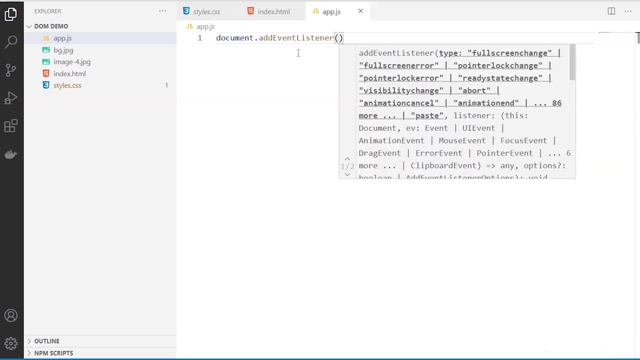 a method. So you can see that it is a method and this blue brick that you see, So that is a property, So that's it. So we'll be using this method. So I'm adding an event over here. So what is the event that you're going to add now? 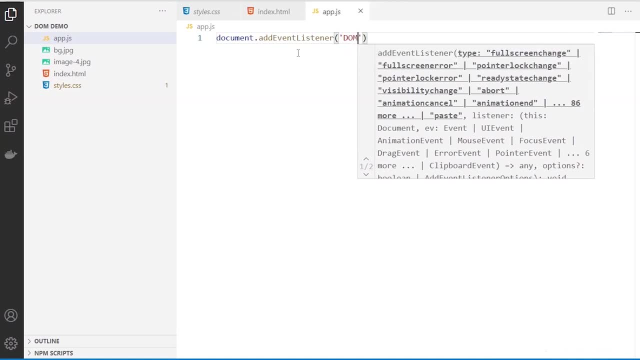 So we are adding this event which is called as the Dom, So I will explain. So what exactly is this DomContentLoaded? Now, this event fires when the initial HTML document has been completely loaded and parsed. So this is the DOM content loaded. 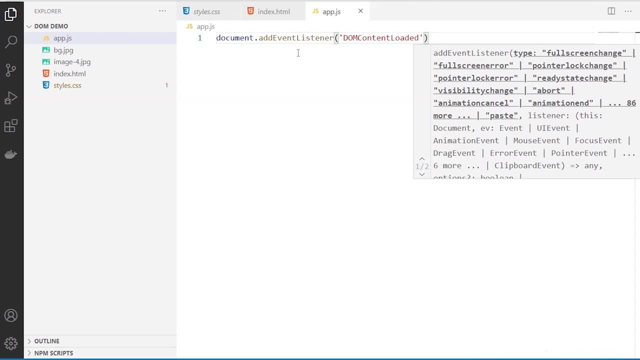 Now this event fires when the initial HTML document has been completely loaded and parsed. So this is the DOM content loaded. Now this event fires when the initial HTML document has been completely loaded and parsed. So without for other dependencies like your CSS files, style sheets, images or any other. 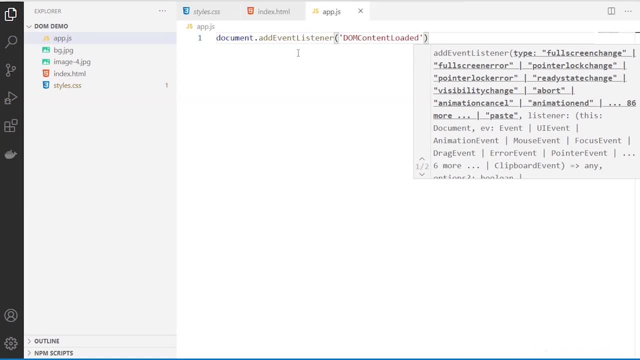 elements to finish loading. So your original content. so if it is loaded and parsed, this event will be fired And the target for this event is your document itself and that has to be loaded And you can listen for this event on the window interface to handle it. 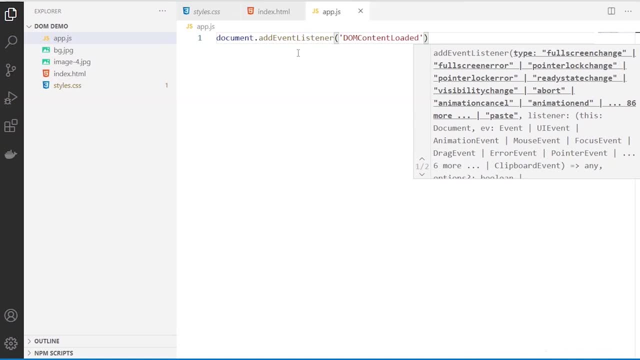 How to load-out is A And B And C And O And Y. So that was our content of the day and it can be captured. so there is another event which is called a load. now that will be. you will not be using that for this particular purpose, so here I'm. 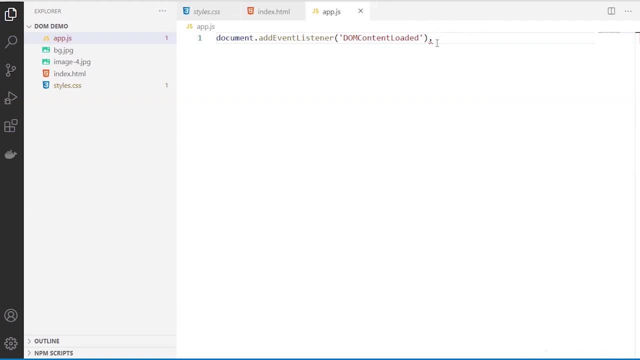 just using this event to check if the content if that particular document, your HTML document, is loaded without the other dependencies. that's what I said, without the style sheet or other features to be loaded. but another event is there which is called as just load, and it should be used to detect to 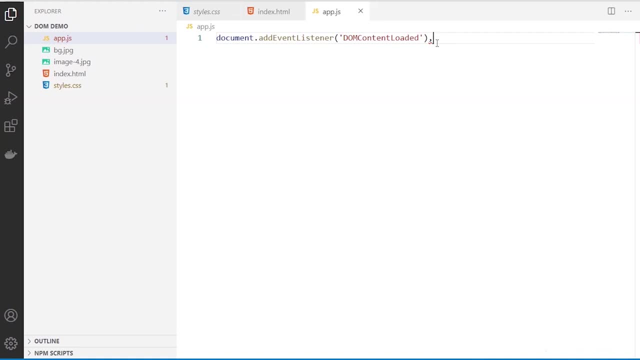 detect a fully loaded page along with style sheet and everything. so it's usually people confuse between this load and the document content loaded. so understand the difference. for load it is like fully loaded, whereas Dom content loaded is only when the Dom features or the HTML content is loaded. so let's 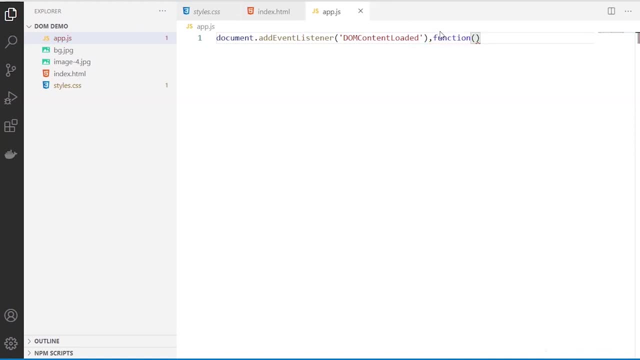 write the function for this, so using this syntax. so first is this event name and here we are going to include the function, so all of the function that we will be including, so it will be going inside this main function that I have. first thing that I'm going to do is 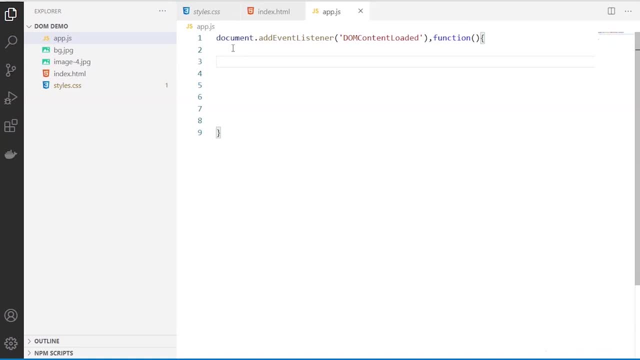 create variable. in this case we will be creating a constant, because we are not going to change anything to capture where exactly these event and the functions are going to be written will be affected. so in our case, the list movie list- is where we are concerned. we 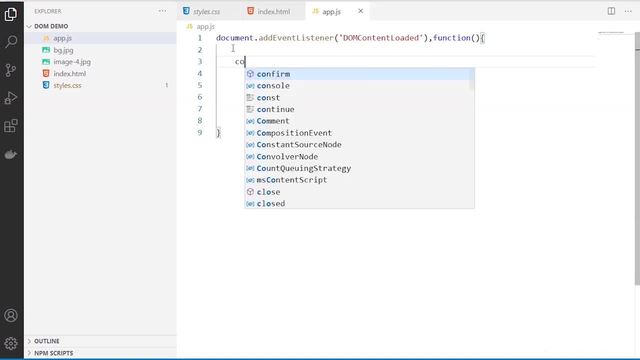 can add a movie, we can delete a movie, so we have to create entity which can refer to that particular list. so I'm creating, so you can use a var also here, since this is not going to be changing. so I'm using a constant, so I'm using this. 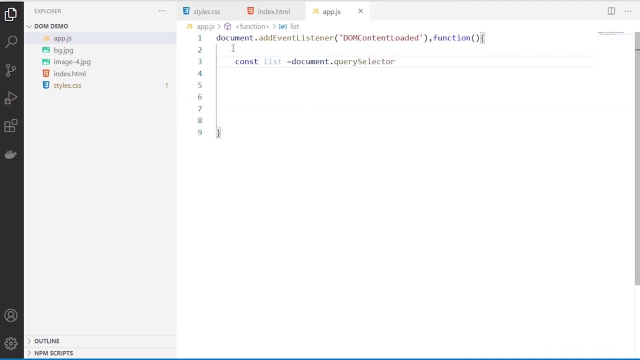 method which is called as your query selector, by which you can select that particular, you know the element, whatever element that you have created. so here I want to select my unordered list. so I'm using this movie. so it is present inside container which is called as your movie list, so inside which I'm 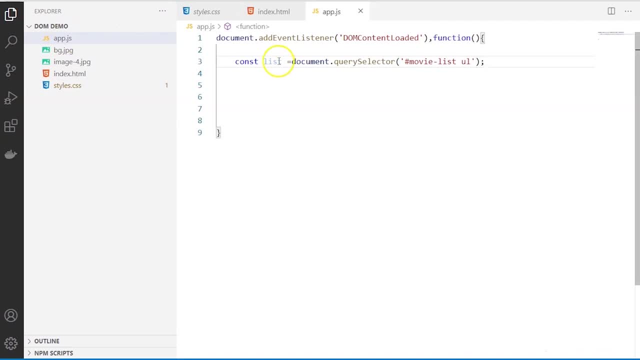 selecting this unordered list and that is getting stored in this list. so this is it's like disabled or like grayed out, because we have not used this list object yet, so when we use it, so it will be highlighted. I'm also going to create one more to store my form. so whatever forms you can have, like multiple forms. 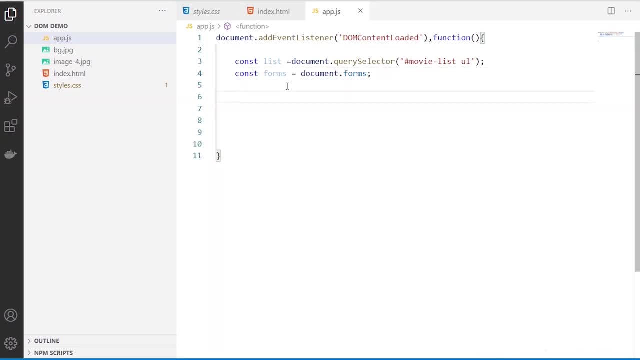 also and all the form elements I'm storing here. and so let's do the first one say: if I have to delete my movies, so to delete these movie, I'm going to attach. so we have already created that list. so to that list now. I told you right. so now if you start using it, it will be highlighted so you can see. 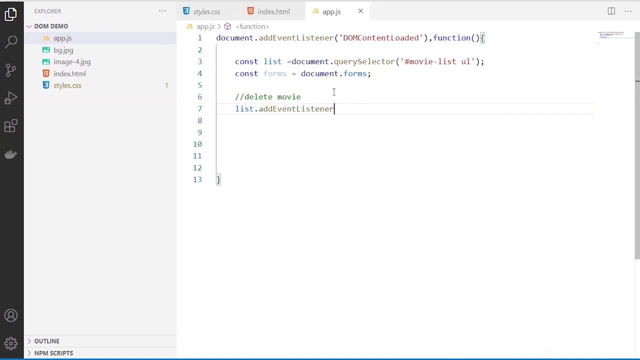 that one. so I'm adding another event listener. so whenever I'm going to click that, I'm going to check if the user is clicking the delete button or he's clicking something else. so I'm using this click event but so I'm attaching a event handler and I am attaching here and then I'm 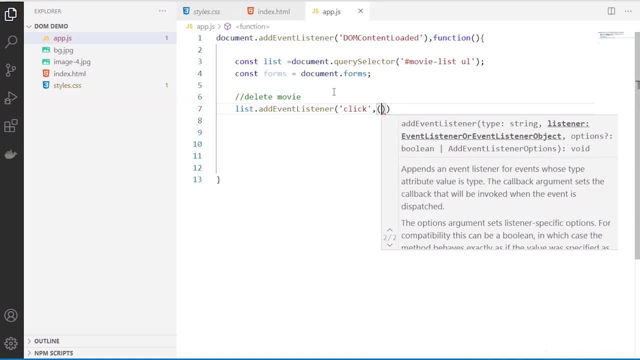 also, you can also pass on another parameter. so in this case I'm passing some E parameter, which is you can also name it as event also, or whatever name that you want. so this event parameters nothing, but all the metadata will be stored in that particular event list. also, as I said, in this case I'm coming currently. 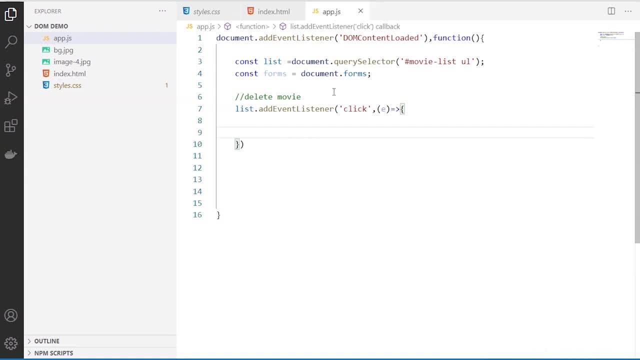 using MeSiko. so going back to that object e or the event object, so it will have all the necessary properties stored there, so you can find out the source of the event, you can find out the target of the event, so everything will be stored in the event object. so here i'm checking using my if condition, so i'm checking if the 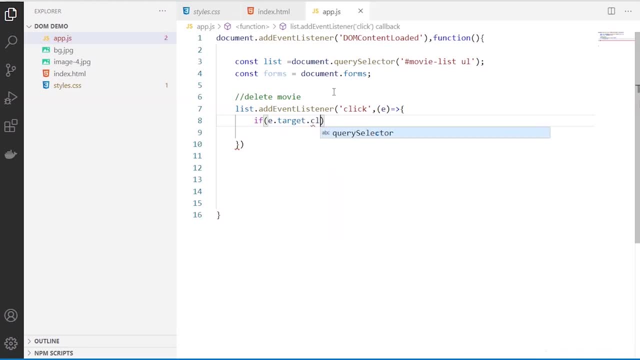 target. okay, so if the target element has, i told you, the event object will have the source where it originated and which is the target. so here i'm checking if the class name is equal to is equal to delete, meaning if i'm trying to click on the delete button, i'm checking that. so if it is, 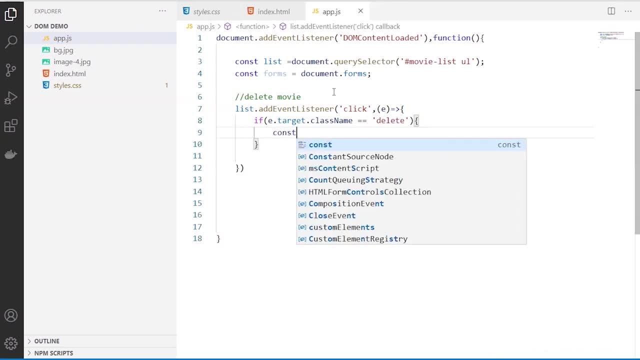 right. so if it is true, then i'm creating a li which is your list item and i'm trying to remove that particular element there. so i'm saying the target, so i'm saying which is the parent. see, when i have to delete the element, it has to delete the entire li right including the span which is the movie text. 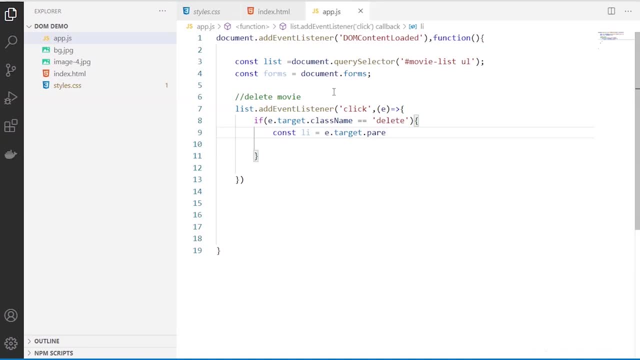 also one more span which has the delete button. so i have to delete the parent element. so here i'm mentioning that i'm creating the li which is the parent element, and now i say the parent node of this particular li. so i want to delete this, so to delete an entity. 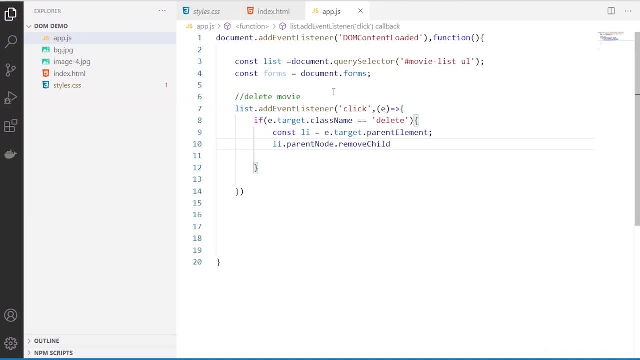 in dom, if you have to do it, you have an uh method which is called as your remote child. so you can see that. so the parent node along with your, so both your span, so the entire li element i have to remove. so i'm removing it like this: i'm calling the parent node, so i'm removing the parent node. 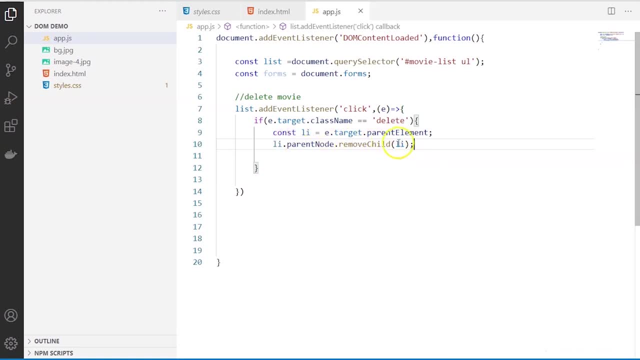 removing it like this: i'm calling this method, which is called as your removed child, which is going to remove that particular li element. so now this is with your li. so here we have added this and we are trying to delete it. so this is one of the functionality. 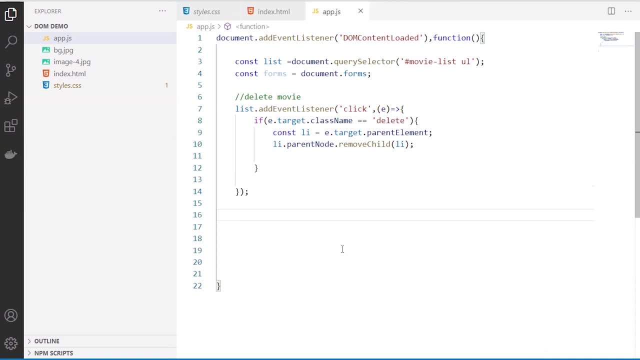 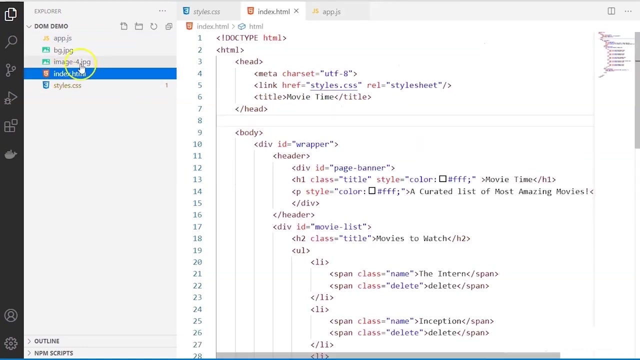 and the next one that we have to do is add movies. so, before adding the movie- so let's see if we had this is going to really work. so for that we have to include one more step. what is that? yes, right, we have to attach it. so your indexhtml does not have this appjs. 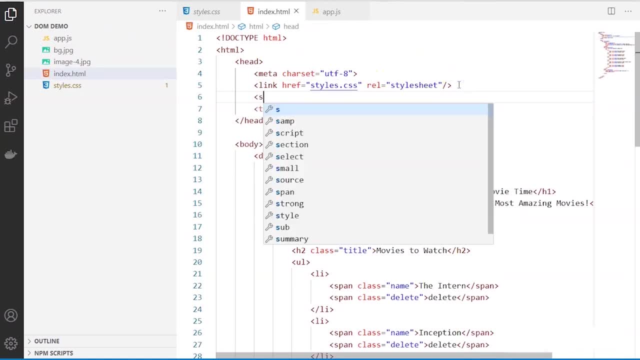 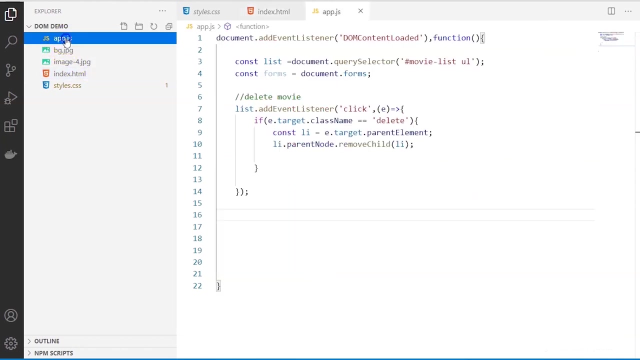 linked yet, so let's add that. so here we'll be using script. src is equal to, so this is my appjs and let's include this one. so once you have included so in my appjs, i have given the main dom content loaded event, so underneath i have these: 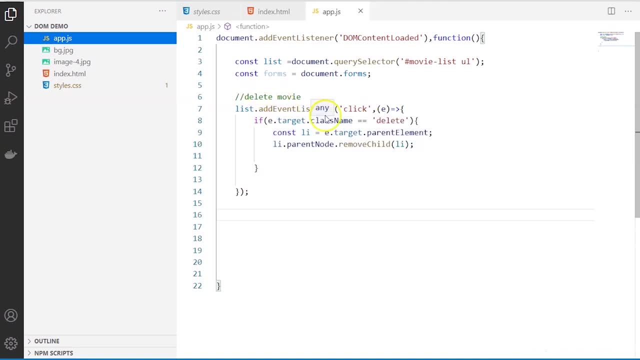 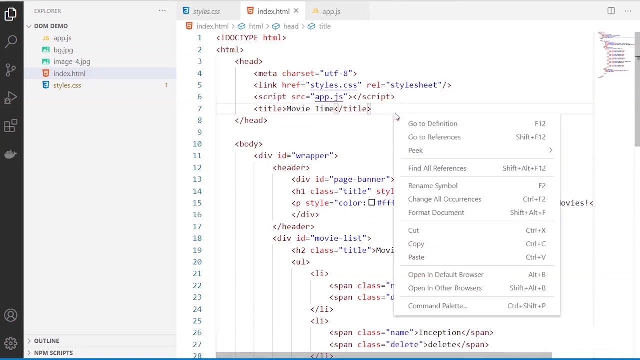 different features included. one is the deleting the movie. one is deleting the movie. another one that we will be writing is adding the movie, so let's see if this is going to work or not. so go back to this. i've already added the script, and so you can open it. so, or you can refresh the. 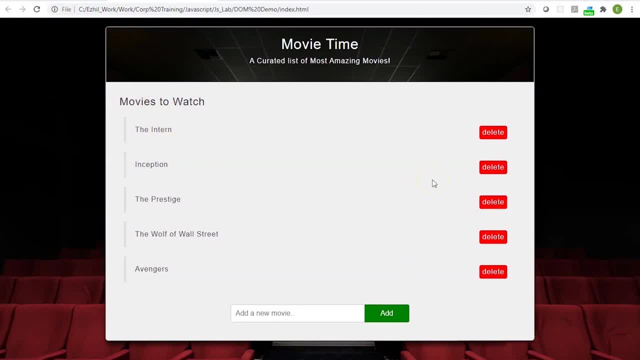 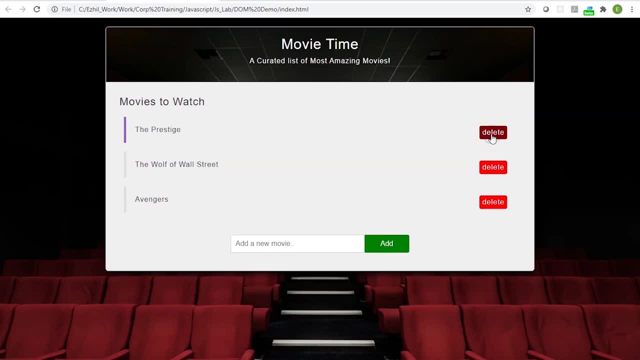 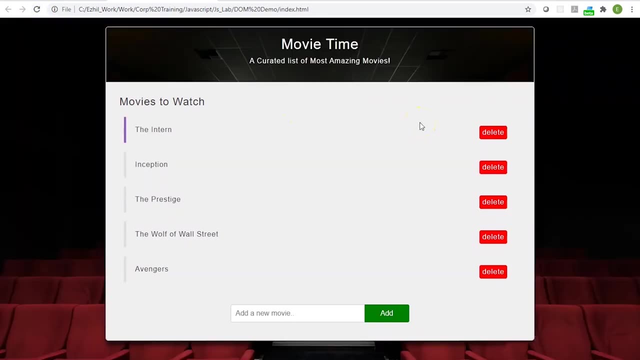 existing page. also, let us see if the delete button really works now. yes, it works. so, okay, i just deleted everything. but, as i told you earlier, this is um, this is not good. but if you see this new release page, well, we are going to delete that page. and because 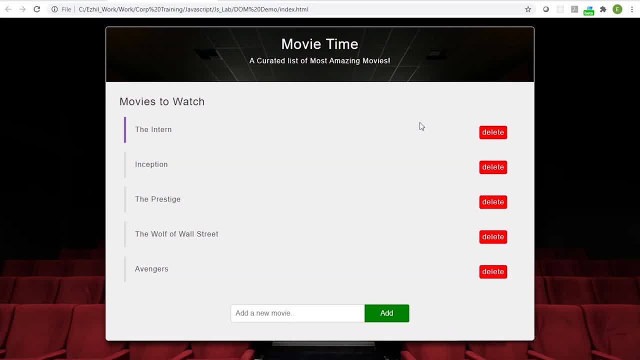 of that. we already have a permanent database that you will be like storing, so these does not get reflected persistent in a persistent way. so when we refresh the page we are going to get it back, but we can see that the deletion by our dom manipulation using javascript code. 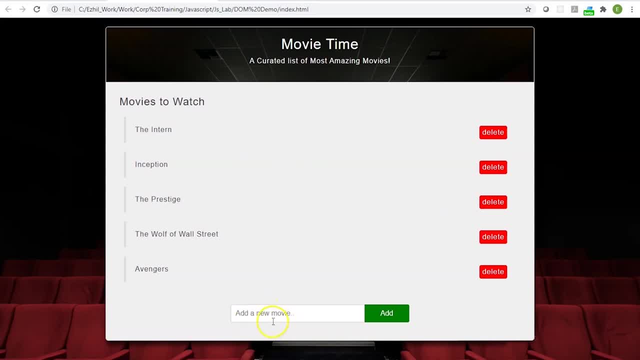 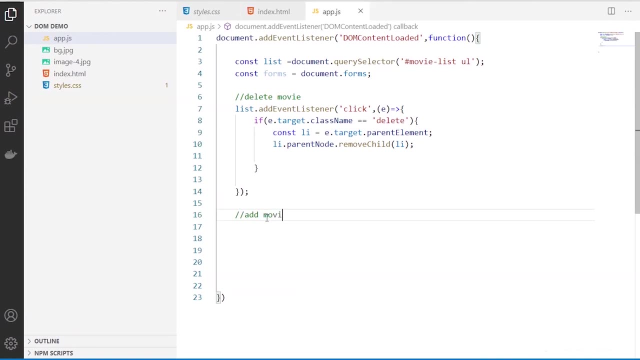 has worked successfully now. so we are done with the first feature. so we will have to move on to the click on this button. it has to be instantly added. let us go back to the editor to add the next feature now. so let's get started with adding the new movie. so it's not like the straightforward. 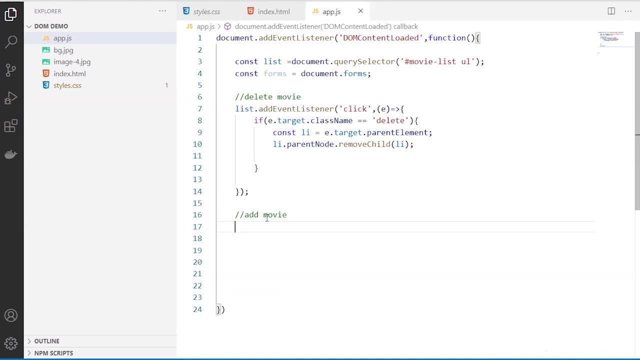 delete feature. there are certain series of steps that is involved when we are adding a new movie. so first being to creating the elements, look whatever elements that we are going to add, so it's just not one text or the movie list. we also have to add the delete button along with that. 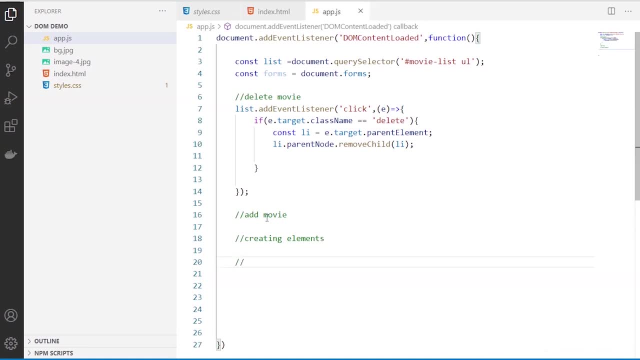 right, so that would be the first one, and the second one would be to add the text content as such. so what is the text content or value? what is the new one? so the delete text and also the name of the movie. so that has to be added, and you can see that each and every um you know these- it has a distinctive. 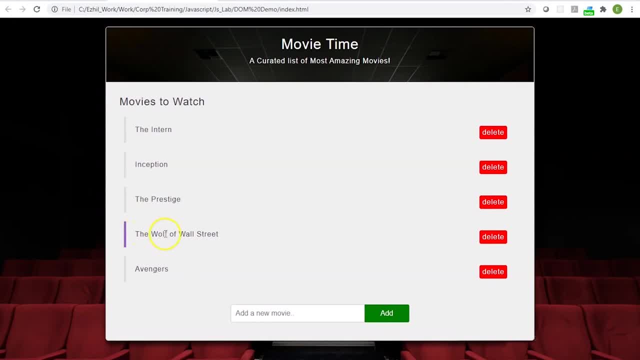 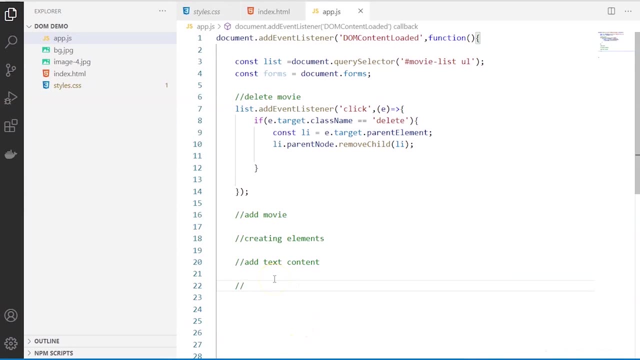 style property: the left, a purple border when it is highlighted, and each row it also has a delete, which is like a red color button which is curved on the edges. so these different style features have been included. so how do we do that? so that would be another step that we have to do, which is adding 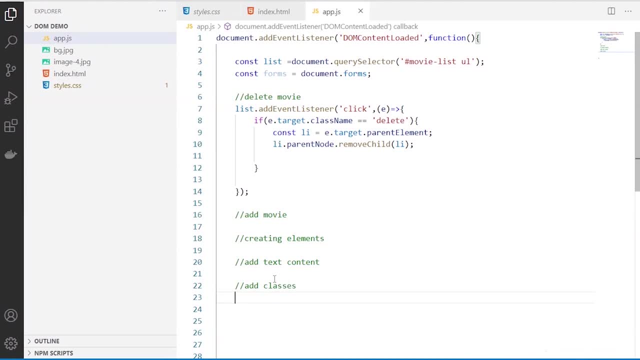 the classes, and finally we will have to attach it to the dom. so then you attach it to your dom element. so let's start with the first phase. so all these elements, now it's present in the form. so from the form we are trying to add the new movie, new element. so for that we'll have to capture the form. so form is in the form of an. 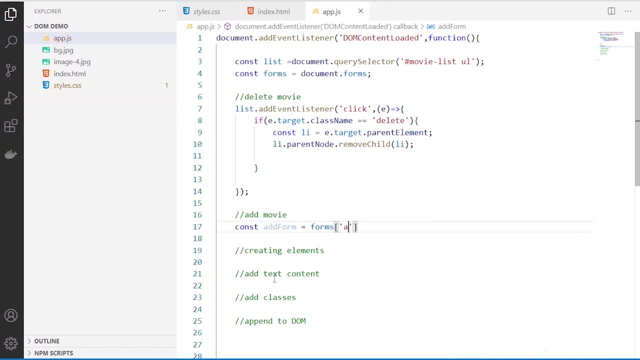 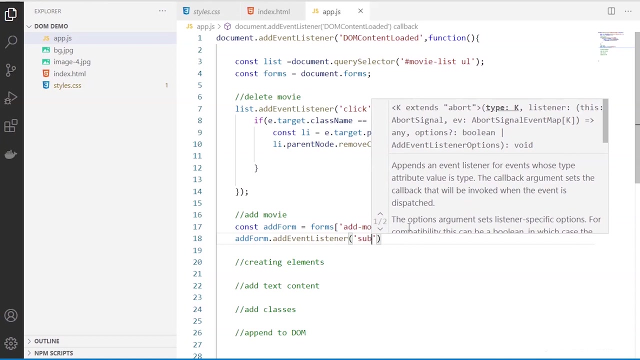 array, so each html element can have n number of forms. so we have already given the id as add movie for that form. we just have one form. so we are retrieving that and i'm storing it inside my add form constant. next, using this add form to add this event listener over here. so when the button so which is so here? 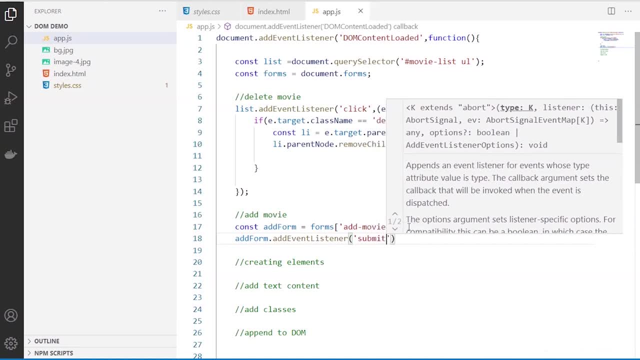 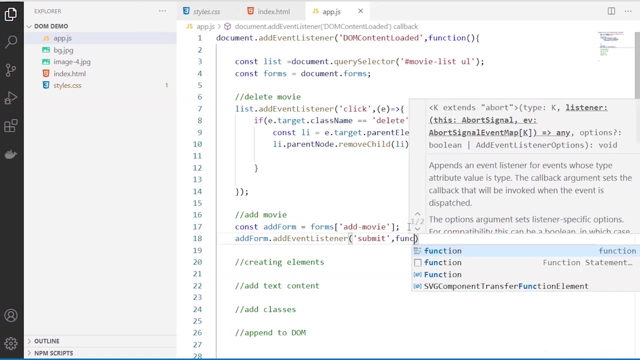 you can have all these events. so here i'm saying: submit is the event, so submit is the most important event so by which you can actually supplement the value. otherwise, um, whatever changes that needs to be captured will not be done properly. so i'm including this function. 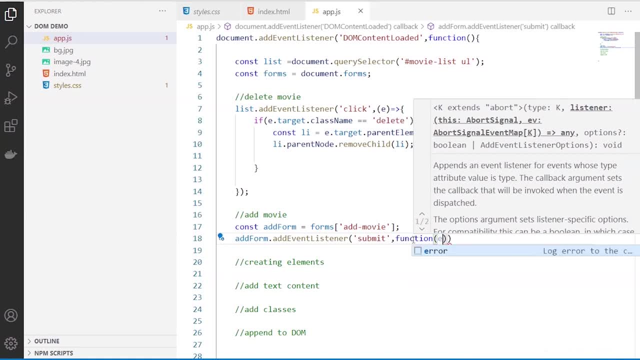 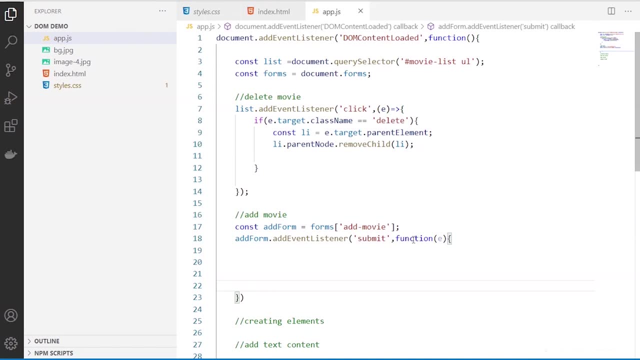 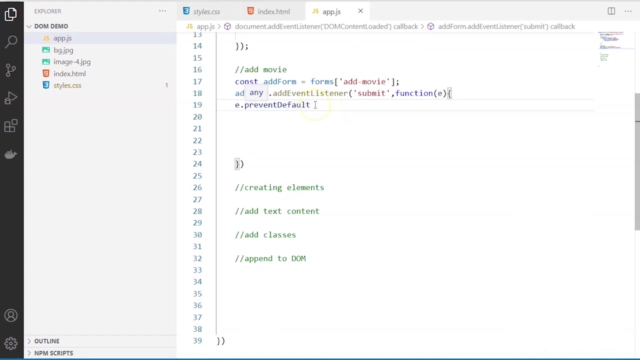 and again, i'm passing this event object, which is your e. so now here, um, i'm adding all these ones. so first one that i'm doing over here is to include your prevent default method, and it's a function to prevent default. this prevent default method cancels the event if it is, uh, cancellable, meaning that the default action. 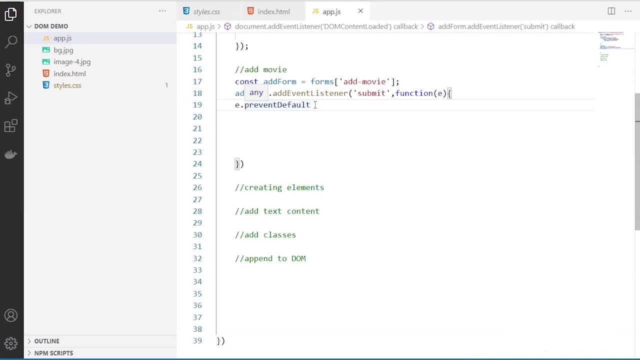 that the uh that belongs to the event will not occur. um say, for instance, if we have to use it for when the user clicks on a submit button, but it has to prevent that clicking or submitting of a form or there is a clicking on a hyperlink or something, but it should be prevented. so these default. 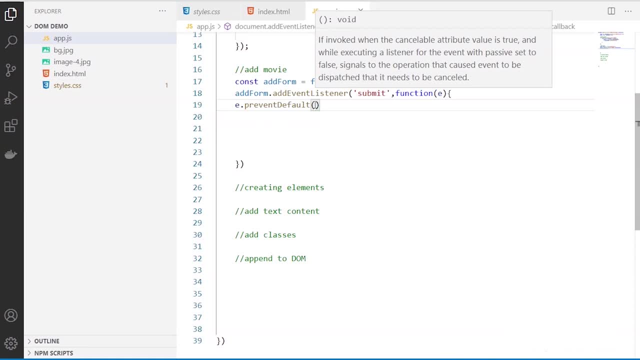 actions. now, if you want to prevent, so you can use this one. so here we are going to use it because we don't want this to be literally bubbled up, and but you also have to know that not all events are cancelable. you can use the cancelable property to find out if some event is cancelable or not. 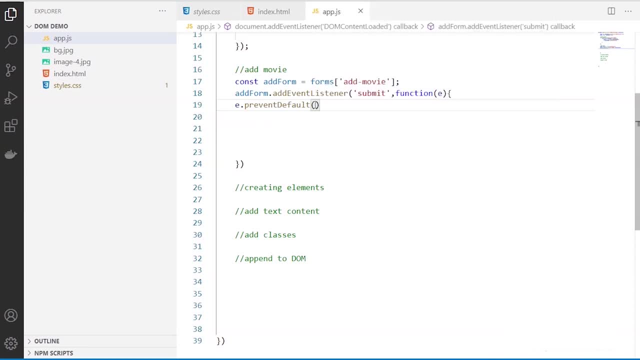 and these. this particular prevent default method also does not prevent further propagation of an event through the dawn. so if you want to literally stop it, so there is another method which is called a stop propagation. so we are in working this method first, and so let me just close this one. 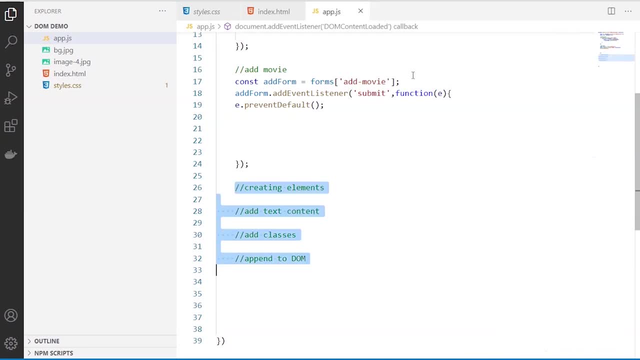 also, and i want all these other feature to be included within this one. okay, so, first step, after creating the capturing the form element, i want to create the other constants for these values and elements, the other elements. so, first thing, i'm creating a constant called as a value. now here i am selecting the using the query selector. again, this: 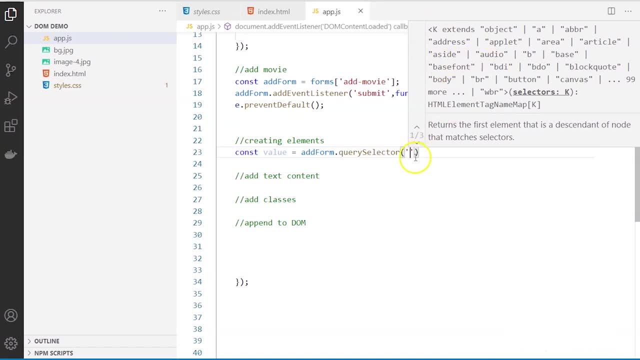 and i want to retrieve this input type. so where i say my text box, so i want to retrieve it. so where i say the type as text, so i want to retrieve the input type, where the type is text. so be very careful with the quotes. so if you are using thepping, 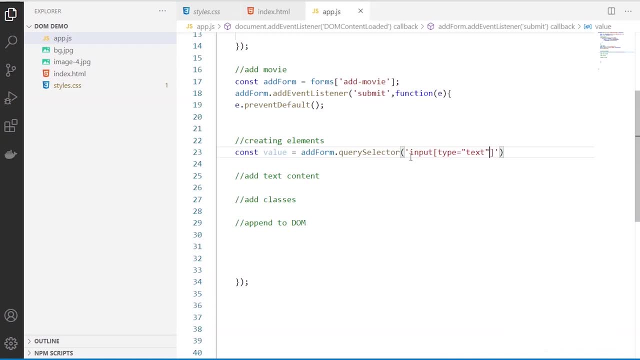 codes as the outer one, just use it for that and use an inner. for the inner code, use a single code, so vice versa. so check on that and how it is closing, so otherwise it will not throw any error, but you will not be getting the value that you expect. also, and the second constant that i want, 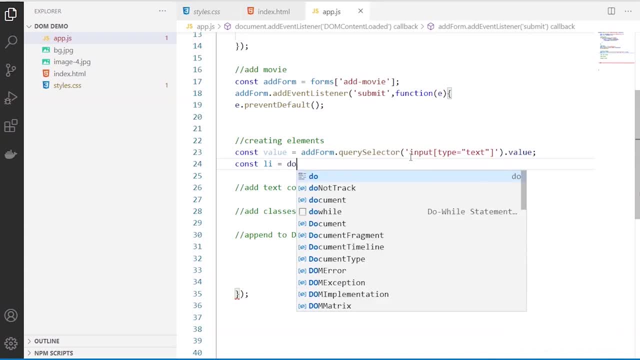 to create. it is for the list item, so here i have the document and here we are going to use this special method. you can see that there are so many number of create element create. even many create methods are there as a part of javascript dom feature, so we are going to use 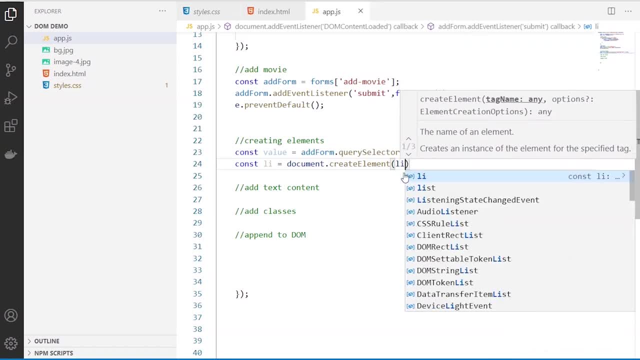 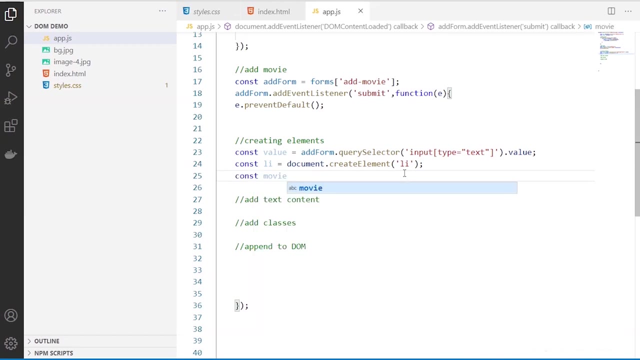 this one create element and i'm going to create a new li element, because this is the one that we want, which needs to be added to the unordered list, and of course, we will have to create the um, the corresponding variable or the constant for the name of the movie. so that has to be there, right? 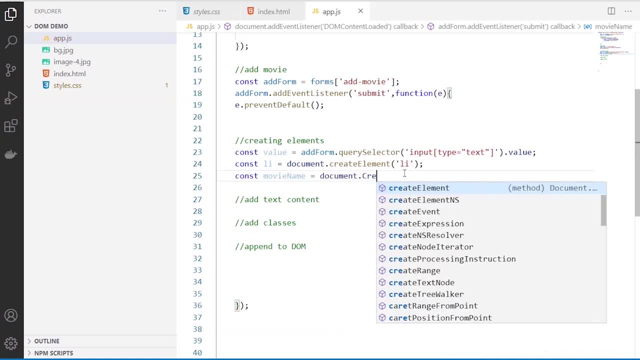 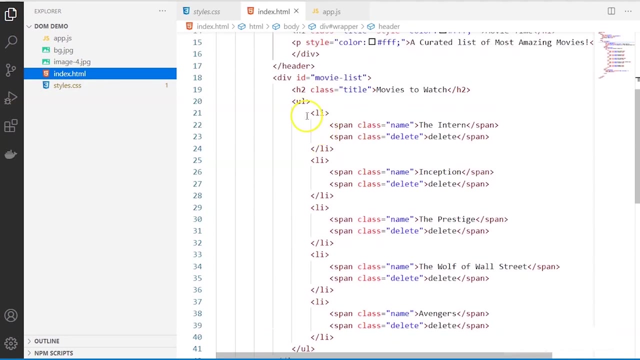 so I'll have to create that one, so that one again is. as you can see, it's a spam, so I'll show you the HTML code here. so quickly let's go, and so you can see this once. this is what we are trying to create here in this feature, so I will. 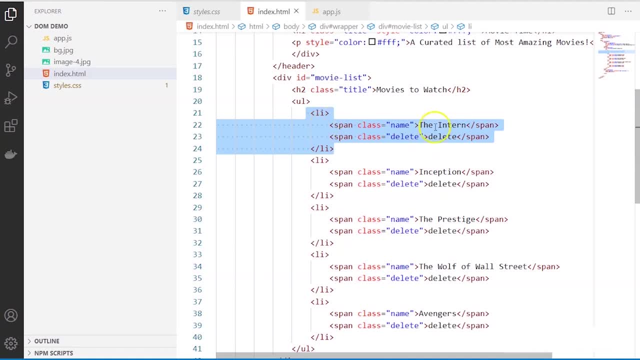 have to create two elements over here. so one is for the movie, another span is for the delete button. so these two has to be created. so this is a span and you can see that the class will have to add next. but this Li element we have to create it. 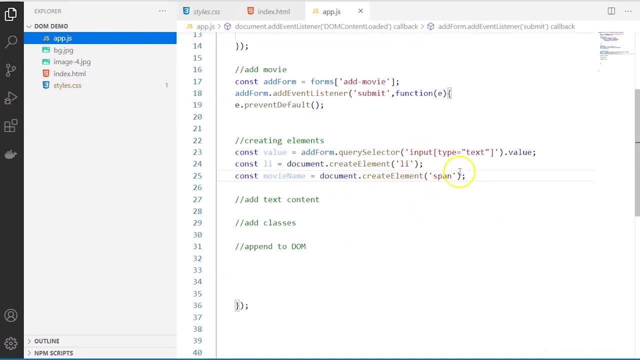 like this. that is what we are doing here, so I am creating a span, so one is for the movie name and another one. we have to create a delete button. so if we have to create a new record, so each record has a movie name as well as. 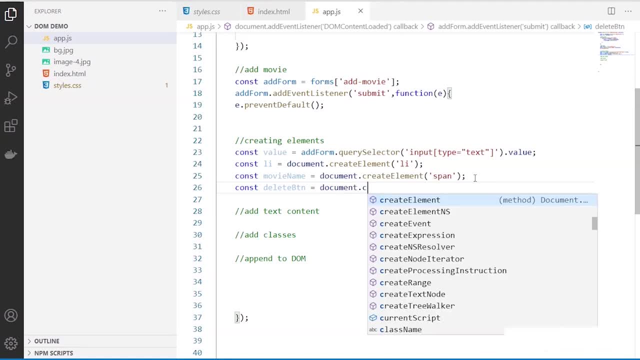 the delete button, so I'm going to create that as well. so in this one again. so what is the element that we will be creating in both the cases? both are span, which is present inside Li, so Li is the parent element and these two span will be the child element. so all these have been now created individually, or 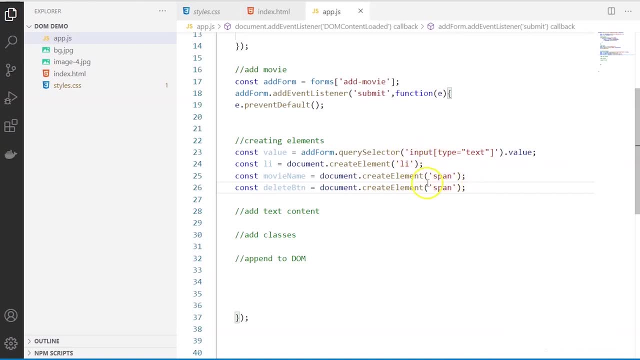 separately we have created. now we have to set the hierarchy, so we have to append these two as child of this Li, and this Li has to be attached to this body, so this one, so this appending will do it at the last right. so first step we have. 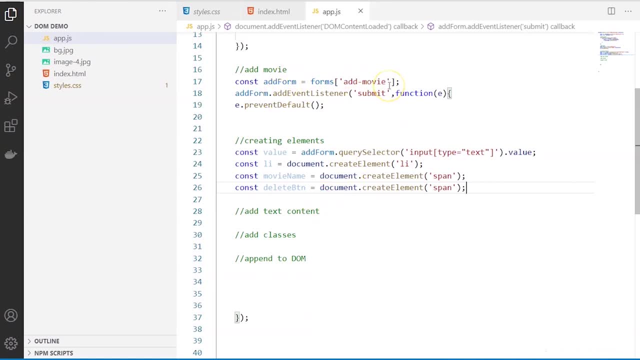 created this elements. so first we have retrieved the movie and we have added attached eventual is now for the Submit button. and And then in the second one, second phase of creating elements we have created. So we have checked if whatever is the value that the user is entering inside the text box. 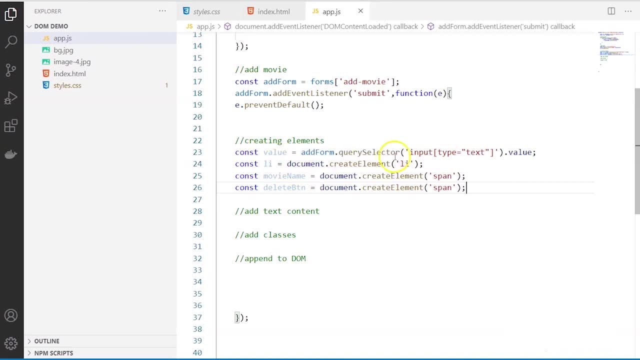 So, using that, we are going to create it. So then, we have created the ally element, which is your list item, And then the span element for the movie name, span element for the delete button. So all these have been created. Now let's go to the next phase, which is to add the text content. 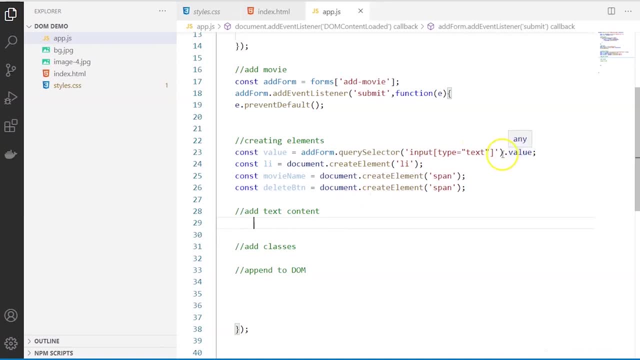 So we have already received the value that the user has entered in the text box And we are storing it in the constant called as value. So now that we have to attach it to this particular element, which is the movie name. Okay, so that will be the next one. 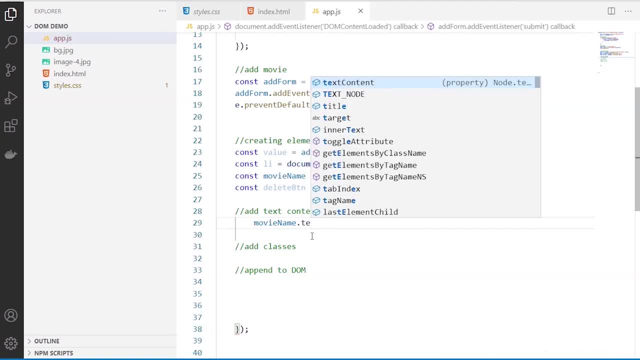 So here I will say: movie name dot. So it has this property, as you can see, which is called as the text content. So this is the span element. So if you have to create a text for that, So I'm saying that, 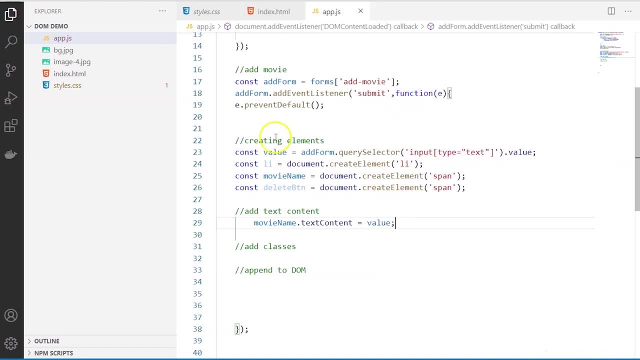 Whatever the user has entered in the text box, that is stored in the value constant, so that I am storing it here, that I'm passing to my text content. property of the movie name, which is nothing but the span that we have created. Now the second one: we have also created this delete button span, right. 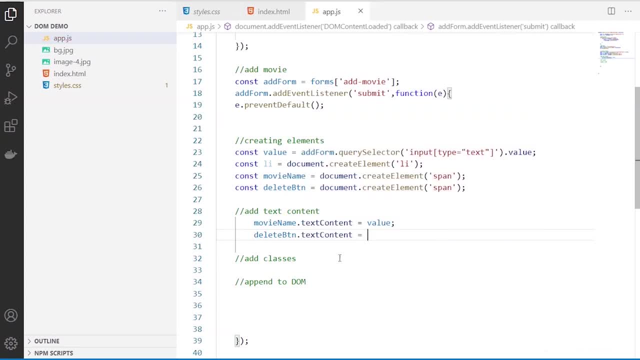 So that so content we have to create, so, which is nothing but the text that will be displayed. So here we are, creating the button as delete button. Okay, so however you want to create, it, remove or the decaps, however you want to create, you can go ahead and create it. 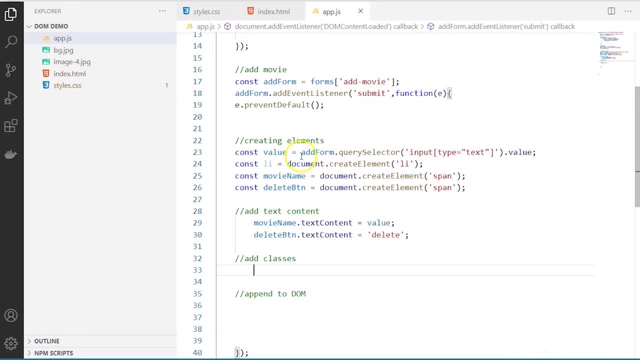 So now this step is also over. So first we have created this form, and then we have created all these elements, the corresponding li and then the movie name span, delete button, span, And then we have also attached the corresponding content for these two span elements. 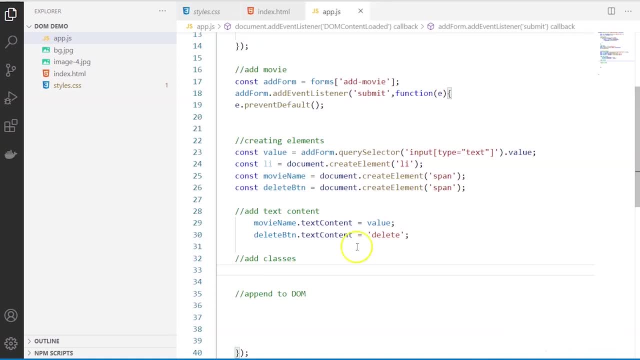 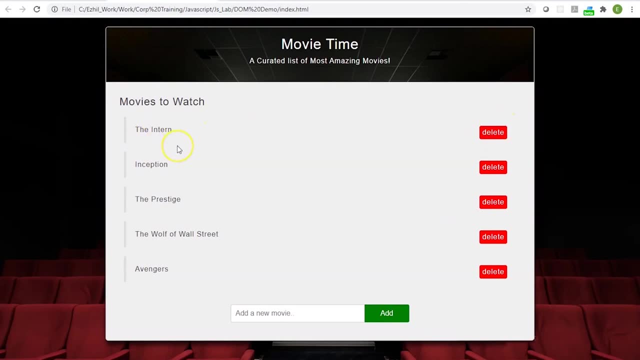 Now we have to add the style, So of course you can see like how it is displayed. So this one has the red color buttons and then you can see the different these borders so that we have already created in the external style sheet. 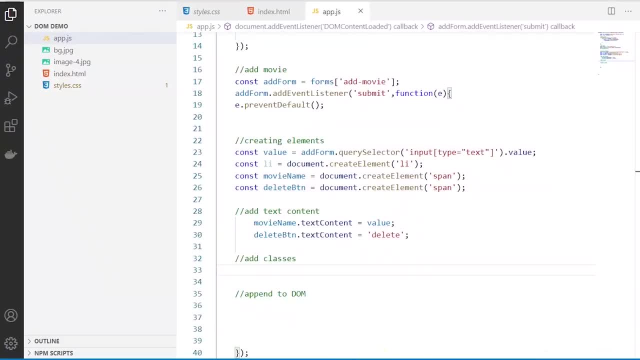 This has to be updated here. So we are doing this. So I say class list dot add. So this is add. So we are adding the class name for the corresponding element that we have created so that you get the style feature that we have already defined. 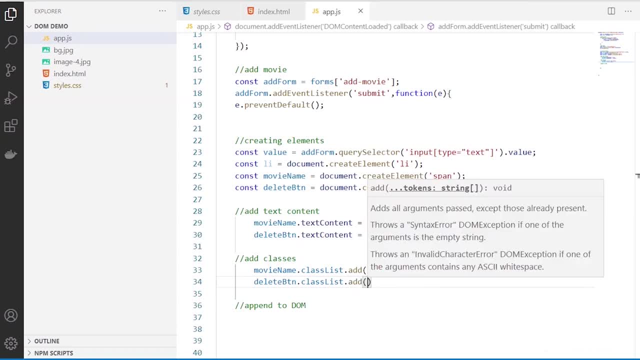 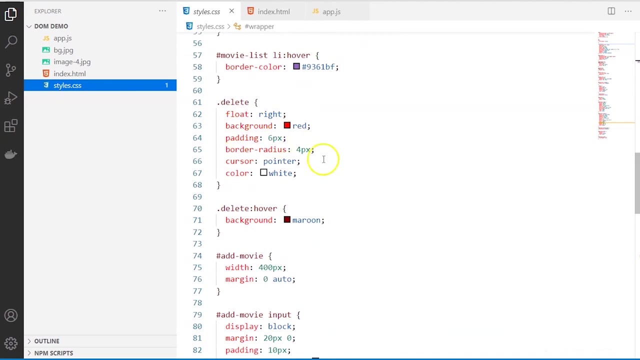 Okay, by default, it goes on with your add event listener. All right, So this is. this is the class name. Okay, so we are adding it. So let's go to the style dot CSS, And so you can see this: delete and name. 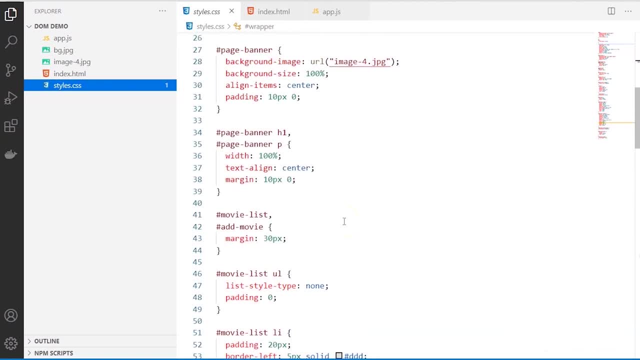 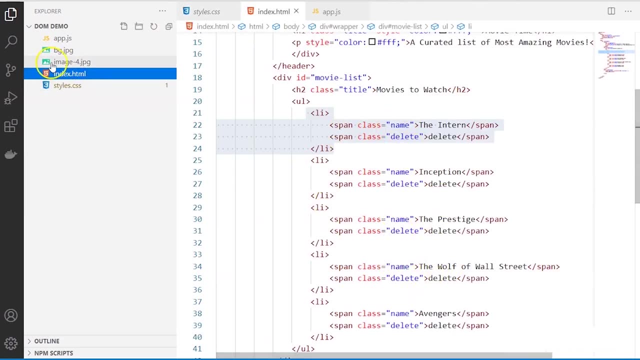 So all these are present over here, All right, So all these are there. So I want to attach, So you can see this one name and delete. It already has this one, So that we are trying to attach it here. So this step is also over. 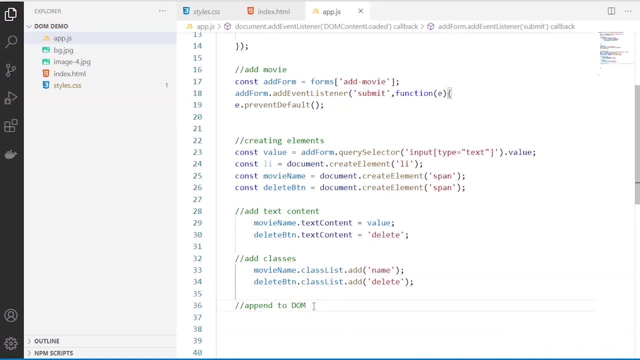 So we are attaching the class for the Style or the theme purpose. Now, final and most important one, is to attach it to the DOM so that all your content, along all your elements, along with those textual content added with those class properties, with the CSS features, 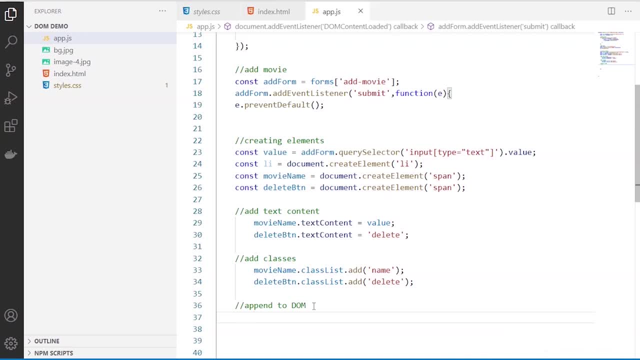 Now it is all rendered onto your DOM in a proper hierarchical way. So that is now is very important, So that is the final step. So I'm saying LI, So now LI is your parent element, Right? So I'm attaching my LI. 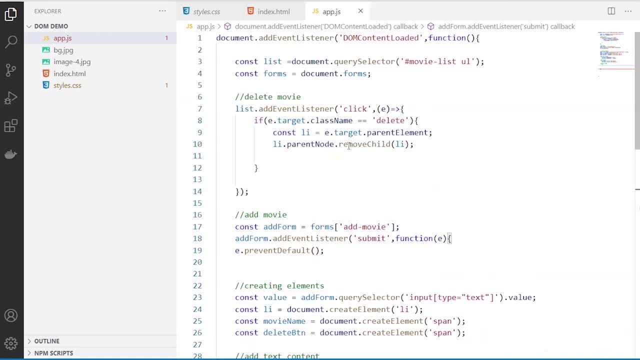 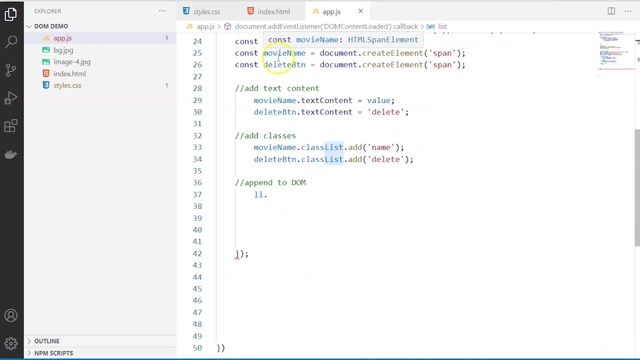 But your LI has to be attached to the list. I think they've already created this list, which is nothing but the unordered list. So this LI has to be attached to the list And inside your LI these two spans your movie name and delete button. both has to be attached. 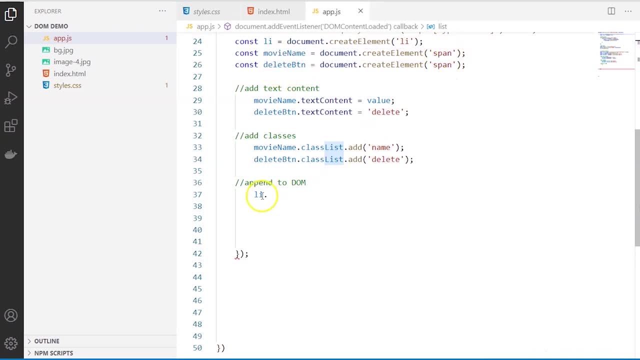 So your movie name And delete button are the child elements of LI And LI is the child element of your list, So it has to be attached. So first let's attach your movie name, So the child of your LI, which is the first span. 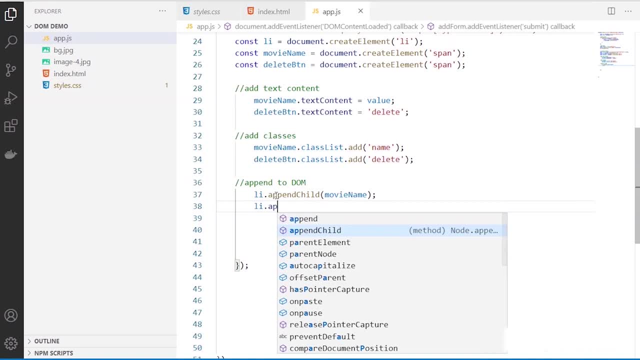 And I'm also attaching the delete button, So which is another span. And finally, I'm attaching the LI, which is in turn a child of the list element. Okay, So here I say listappendchild, which is your LI, Okay, 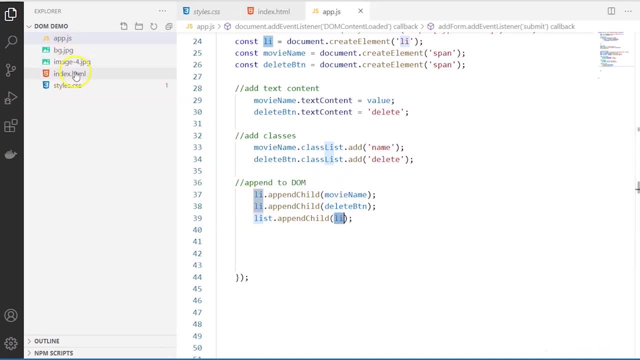 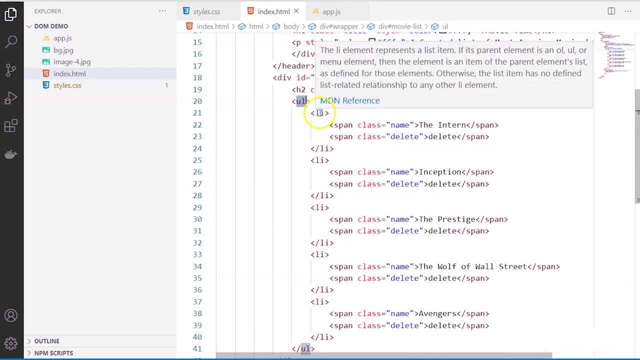 But inside your LI you can see the movie name and delete button. We can go to the indexhtml to check. So UL or the list is the parent element Inside which I have my LI list item And the LI. it becomes the parent for these two, which is the name of the movie and the delete button for each corresponding record. 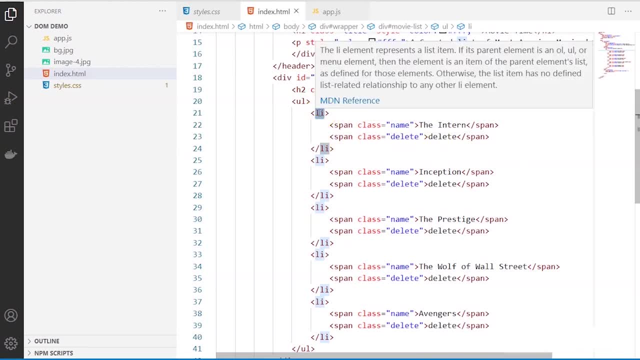 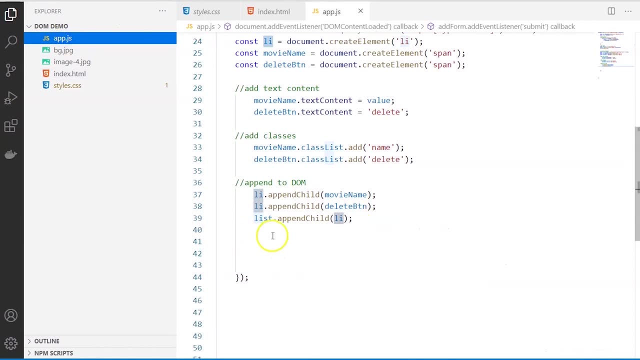 So these two child elements, first we are attaching to LI And then this LI we are attaching to the UL. So that is what we are doing here, Right? So this will be the final and most important step. So with this we are done with the. 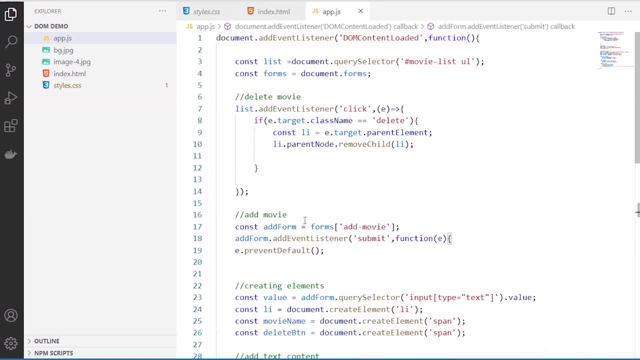 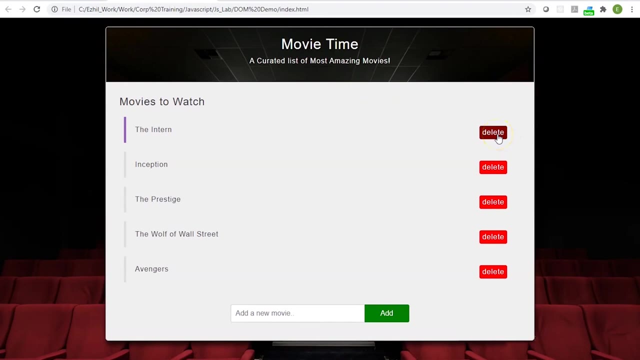 Script, So make sure you save this one And let's go back to this And refresh it once. Okay, So this delete button, it is working As usual. We have already seen that, And let's see if a new movie can be inserted. 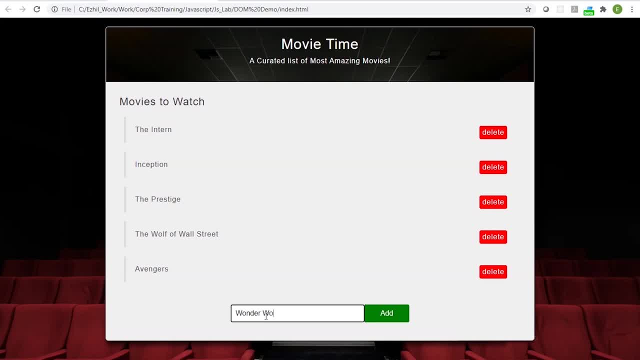 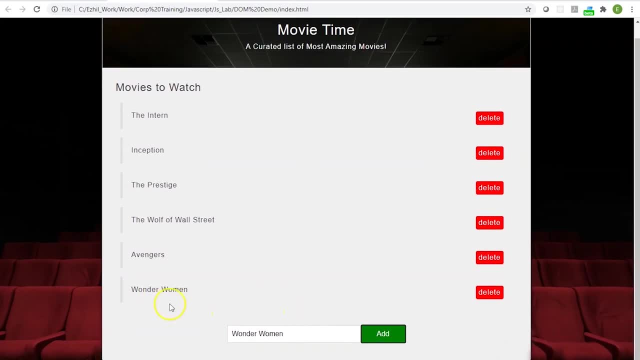 Okay, Let's say Wow. Now you can see that instantly. a new movie has been added at the bottom and you can see the two span elements. which is the child of the LI? it gets added to the parent, which is the list item. 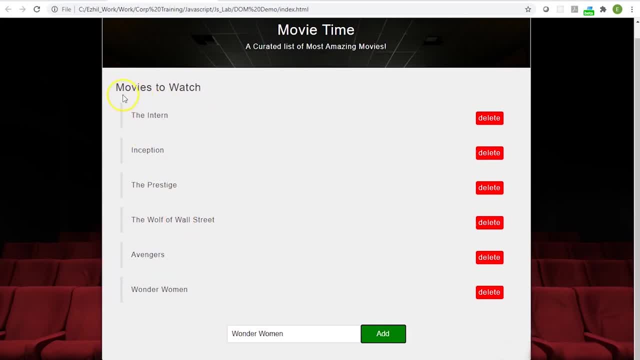 So this is the outermost one, which is the UL Or your list type list, and then each one is the child which is your LI. The LI has two child, which is your movie name, as well as the delete button. 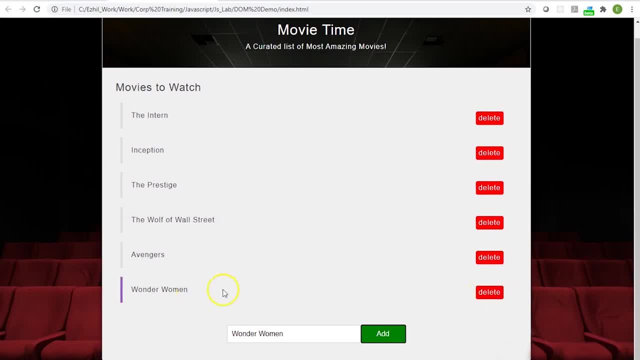 So we have first created these values and then the classes have been added to ensure that the CSS is consistent, And then, finally, we use the doms append child. You can use your append method also to attach it So that This hierarchy is formed. 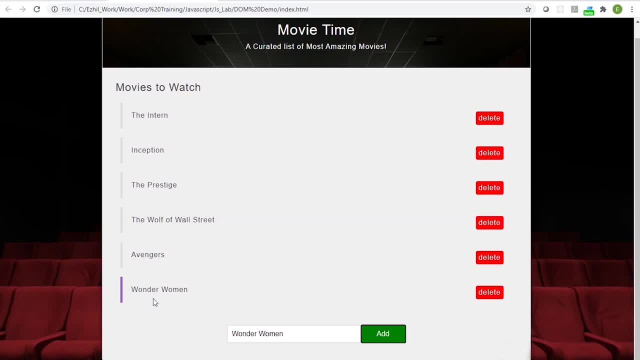 So using dom manipulation via JavaScript. So we have seen that as a very, very powerful in a very in a powerful way and in a very simpler and effective way, how we can add new elements, new nodes, attach events, listen to events and also to delete it. 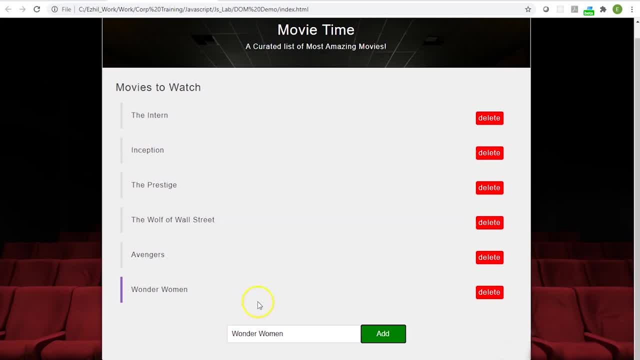 All these. it can be done So effectively, So you can keep adding more. You can try to validate this also and say: if I want to edit this, I won't edit the existing movies. Even that is completely possible. You can do that. 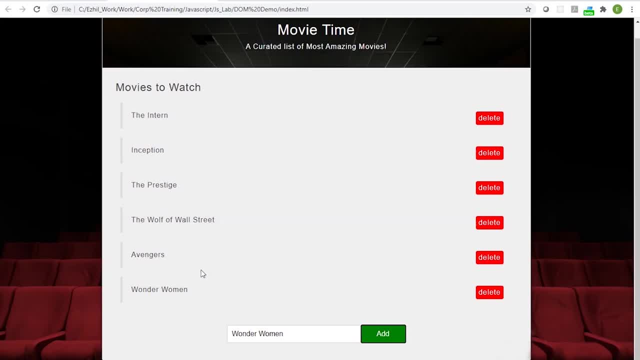 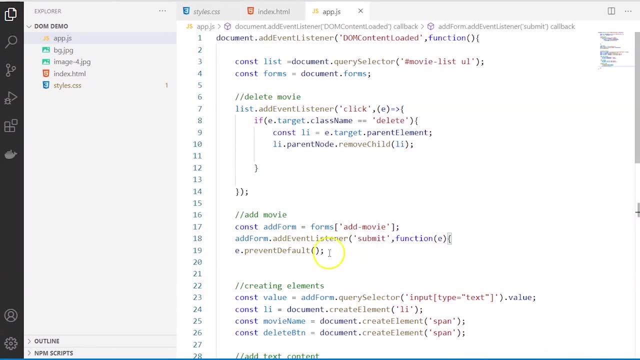 Or only the style. if you want, You can change that style also. So everything just with JavaScript. So just with JavaScript. So how you can create the elements without the HTML content at all. So just with JavaScript. So how you can create the elements without the HTML content at all. 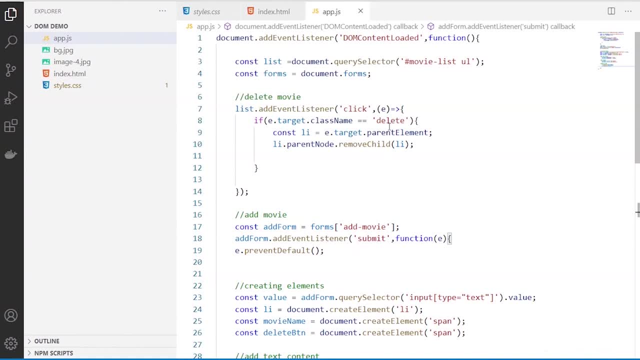 you can create the elements without the HTML content at all. You can just write from the heading to the footer, to the content, Everything you can create just with your JavaScript. So that is the power of JavaScript. So I think we have done quite enough with this manipulation. 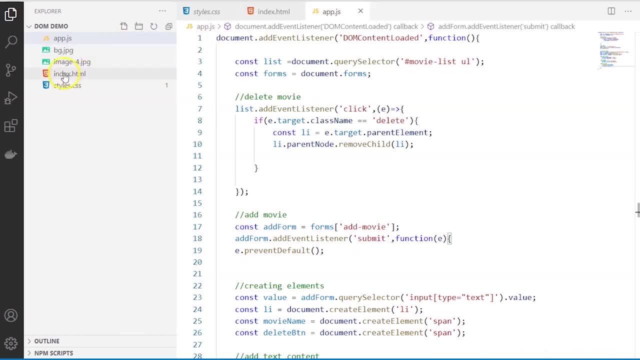 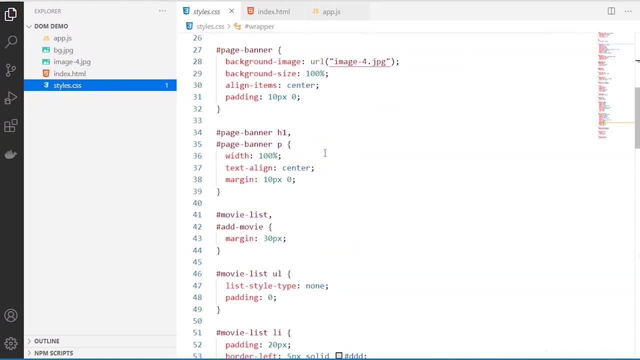 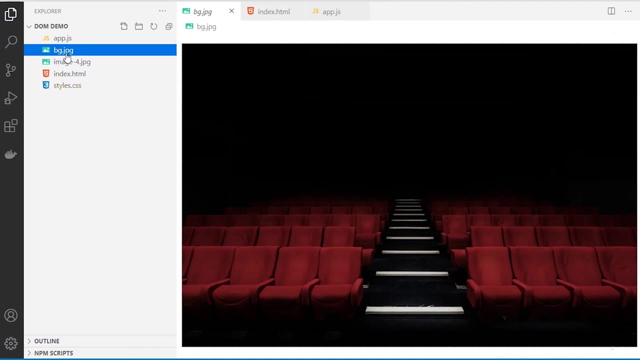 So, for a quick recap, we started with these three files, So stylecss, So I walked you through the entire style and theme features I have incorporated And we also had these two images already So you can include. So this is just an overview, guideline of how this DOM can be manipulated in one way. 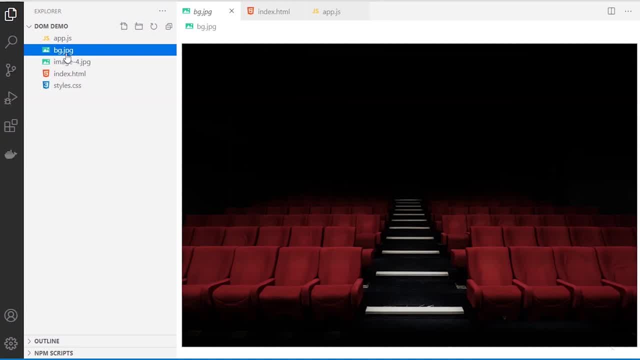 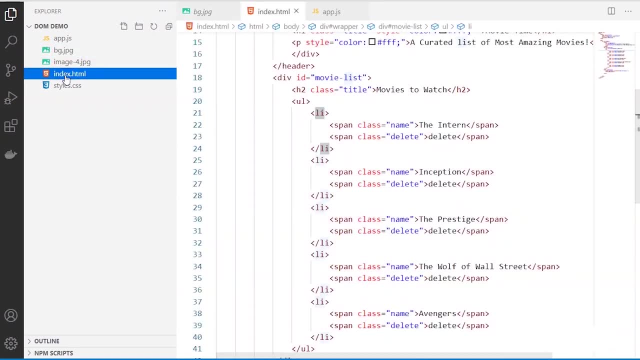 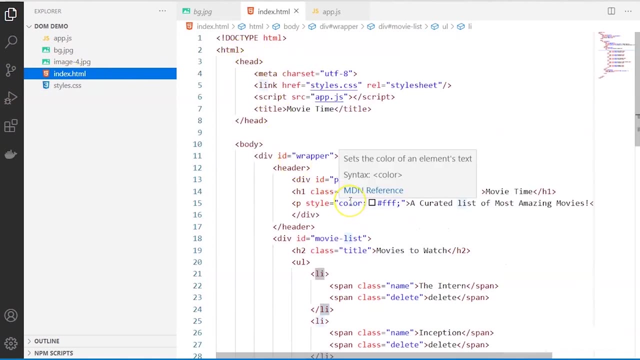 You are free to explore having this as a base And you can just work upon how you want to carry on with your DOM manipulation. So we created first this indexhtml. So we created all the content, the head and body, And initially we didn't attach it with the style sheet as well as the script. 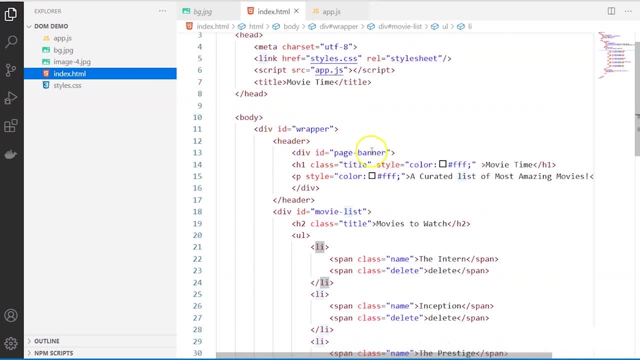 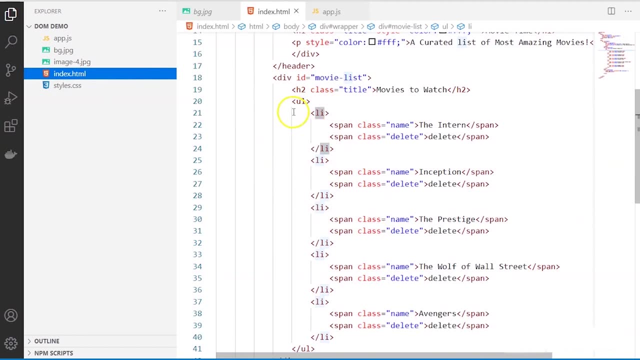 Then we created those containers, the wrapper and page banner, so that we had the corresponding styles for all these, And we also created a ul, which is an unordered list with all these list items. So these list items internally, so it has each one had two span. 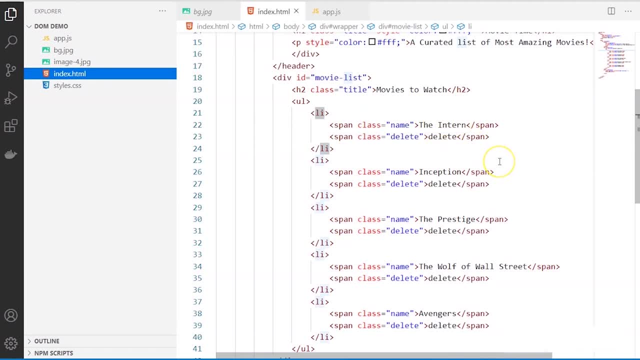 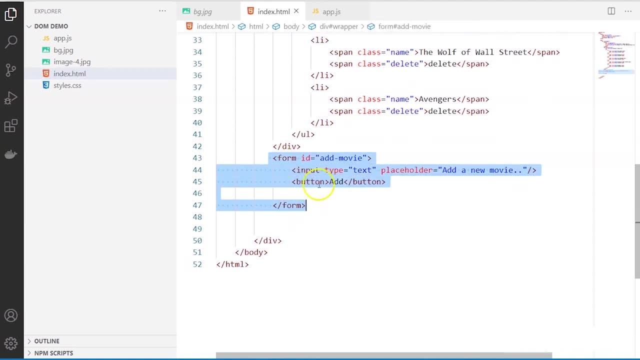 One is the name of the movie, Another one is the delete button for the movie And you also can see that last. we have also added an input element for the text box where you can add the movie, and also a button to submit so that the new movie has been inserted. 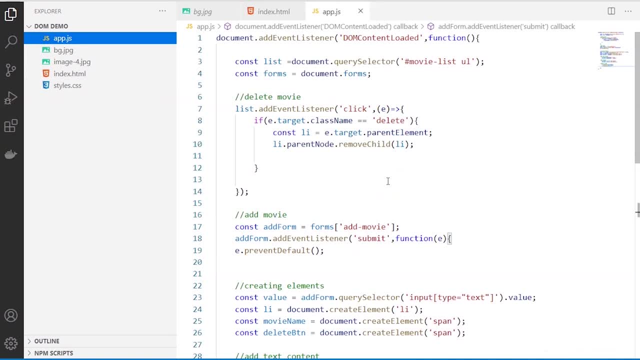 So after this we created this JavaScript coding. So we started with the DOM content loaded and first we saw the delete movie. We use the event listener whenever I click on the delete button. So, based on the event object, I check for the target and I'm removing that particular element. 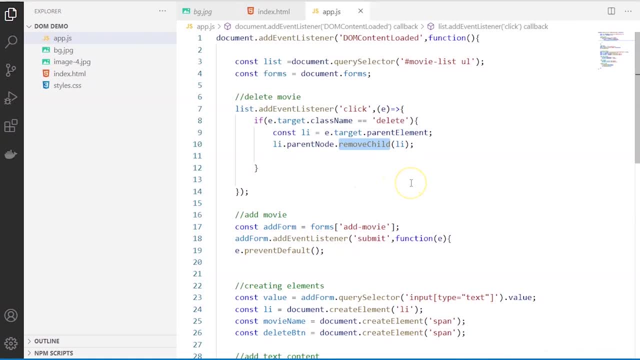 So I'm using the remove child over here for deleting a movie or deleting any particular mode as such, And we are using append child to add the movie. So these two are the important functions that you have to keep in mind, And in the second one we added a movie. 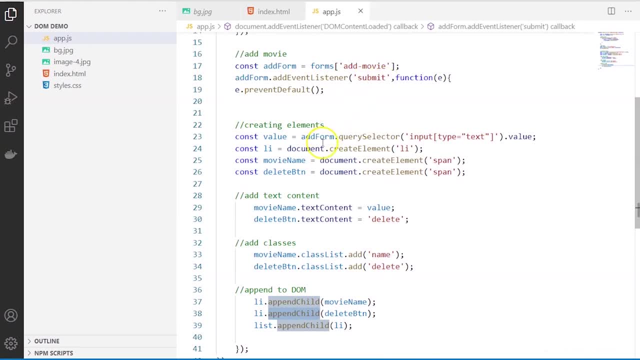 First we created this form, We captured this, and then we created those individual elements, The li span for the movie name, And then we added the movie, And then we created those individual elements, The li span for the movie name, And then we created those individual elements, The li span for the movie name. 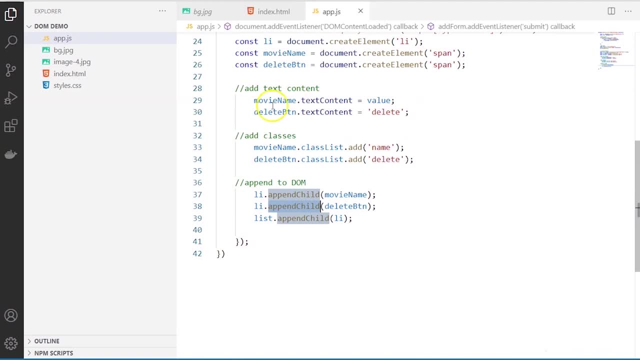 And then we created those individual elements, The li span for the movie name and delete button, And we also had those values that needs to be written, which was added, And then we added the class And finally we use the append child to append these to span element to the li. 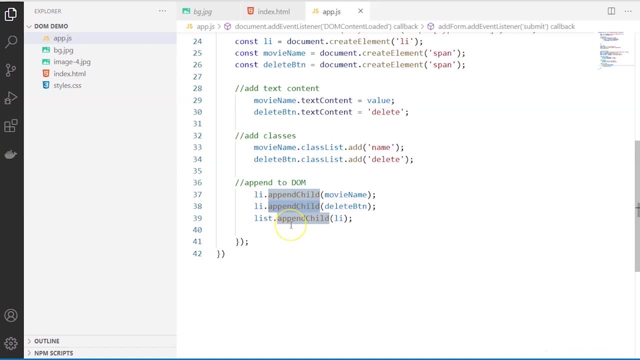 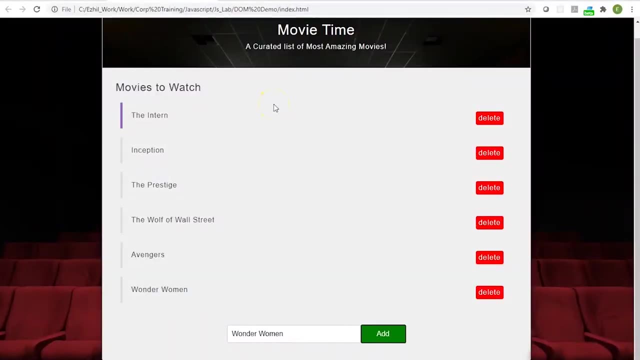 And then li, which is the child of your list, gets added. So that is how we saw this DOM manipulation. So I hope you all enjoyed this demo and also the concept of your DOM manipulation via JavaScript is clear to all of you. 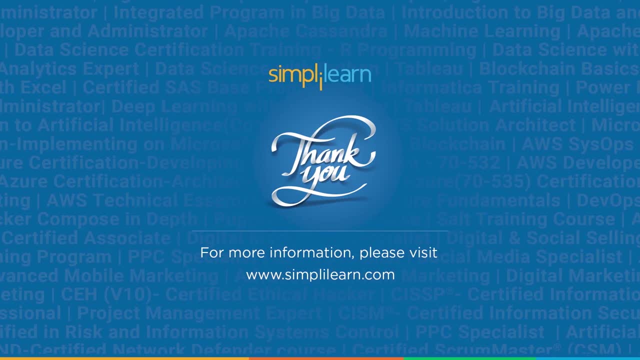 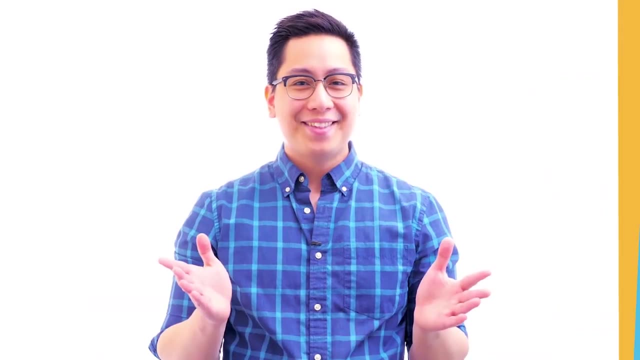 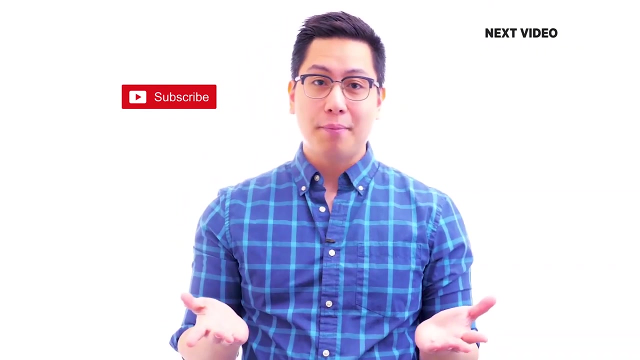 So hope you all enjoyed it. Thank you all so much for watching Hi there. if you liked this video, subscribe to the Simply Learn YouTube channel and click here to watch similar videos. To nerd up and get certified: click here.